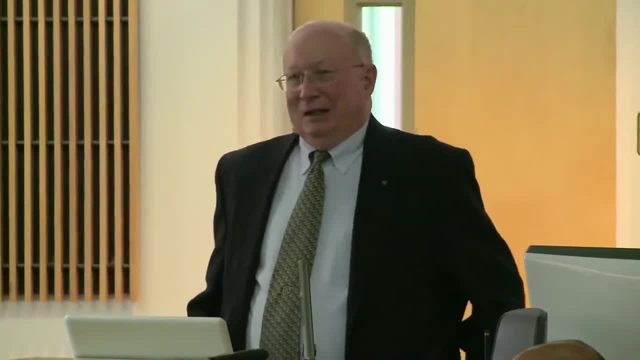 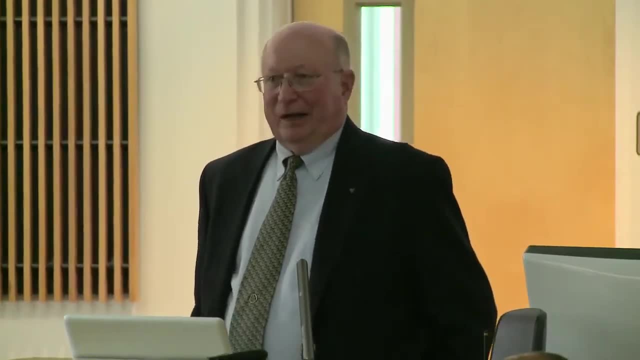 is volunteered. We've been volunteers in Boy Scouts, Girl Scouts, Nordic Ski Association or Nordic Ski Division of the US Ski Association when we lived in Alaska, So we've been active doing this. But the trouble is we live a thousand miles away from Irvine now, So we had to come up. 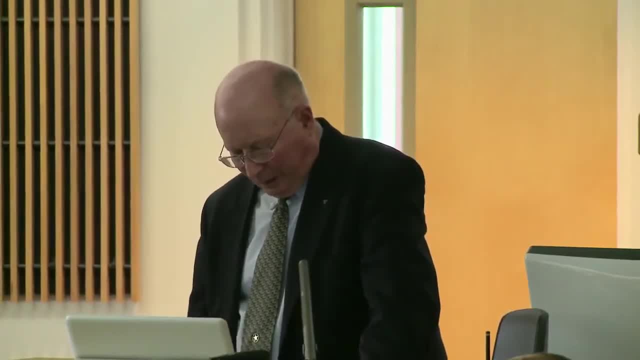 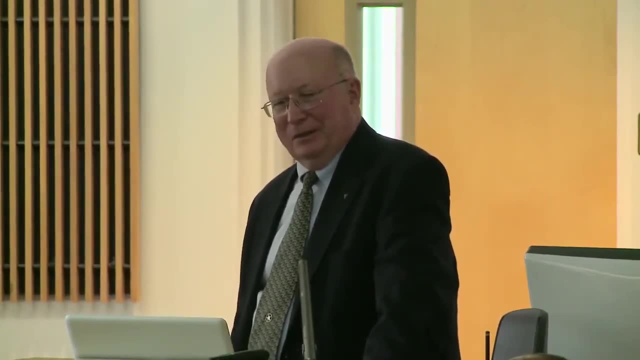 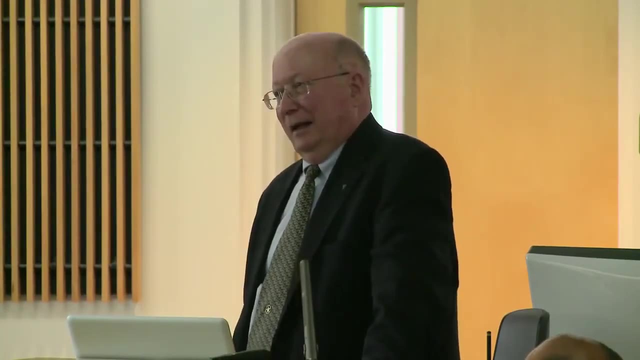 with some sort of a different idea, And so what we decided on was a lecture. I think the department needs some sort of a celebration. It needs something to kind of commemorate your stature with how far you've come, and felt that this was an important way to do it. It's sort of modeled after the Lee. 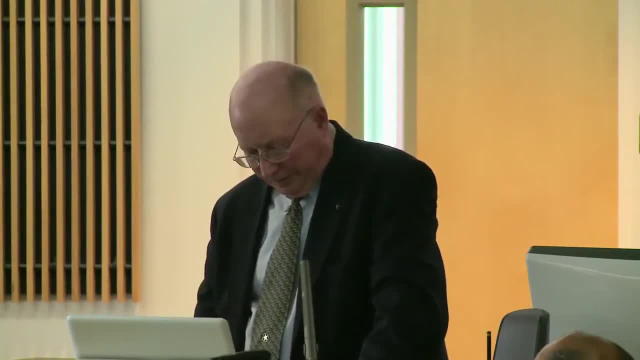 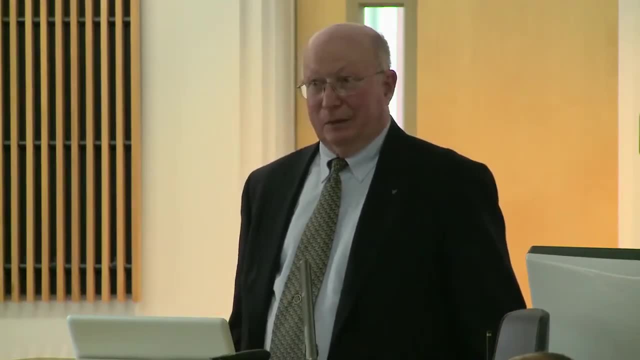 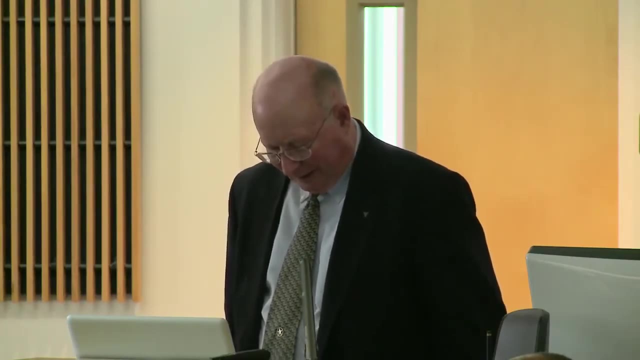 Lecture in Chemistry. They do something very similar each year. The number one reason is that I'm so incredibly proud of what this department has grown into. I was one of the founding faculty and it's come a long way, believe me. It turns out that I regard the 16 years 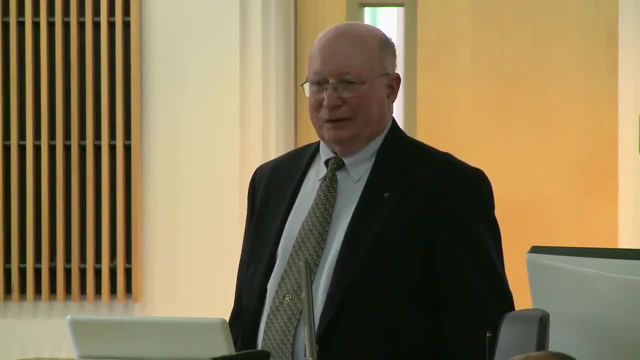 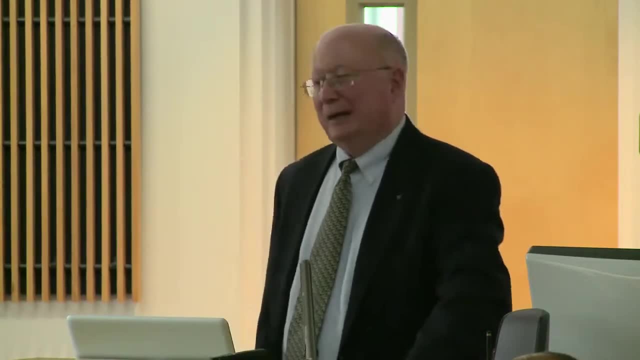 I spent here as probably the best of my career. They were just, super, just electric the whole time, And I'm especially proud of the kind of process that we went through when we put the initial proposals together to form this department. We had to write two. One was a. 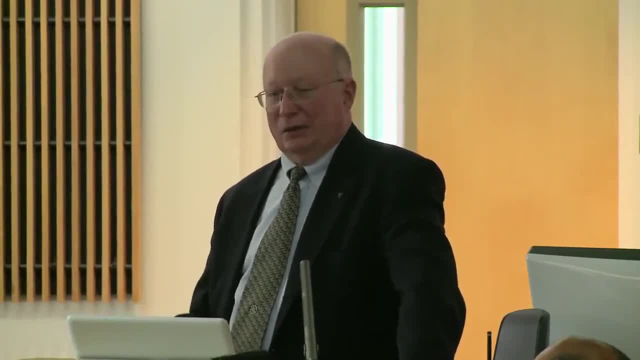 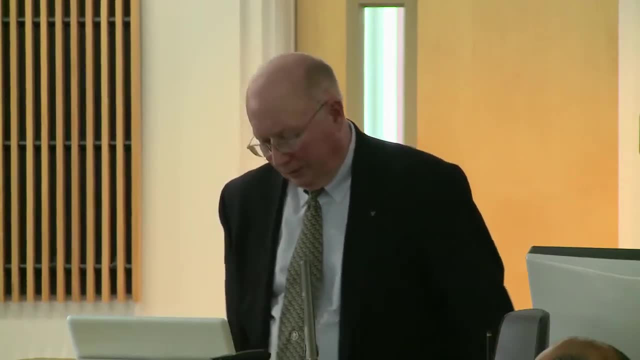 one that dealt with resources and this sort of was to be sort of for internal consumption by the university. And then the second one was a department proposal, after the first one had been approved, And so we did that, And one of the things that I'll never forget- 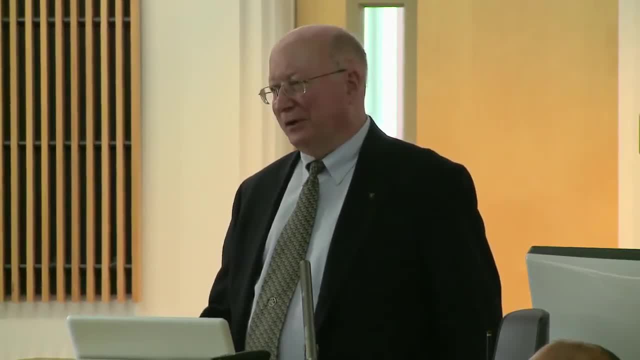 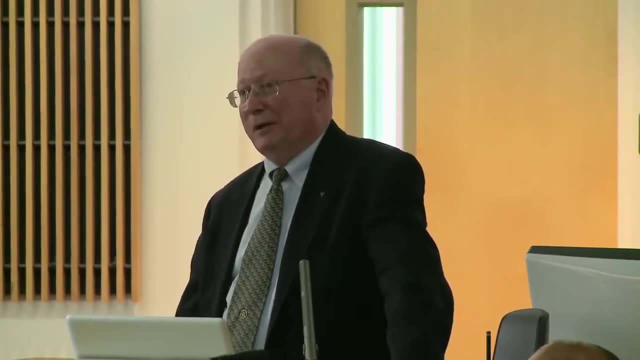 is the way that the initial faculty- we always checked their disciplines at the door And we all came in and focused on the hard task of producing the best possible program- new program in a new area or system- science- that we could- And it looks like it's a little bit different than what we might have expected And the 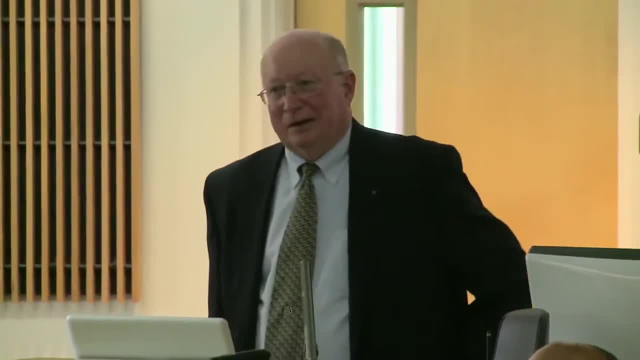 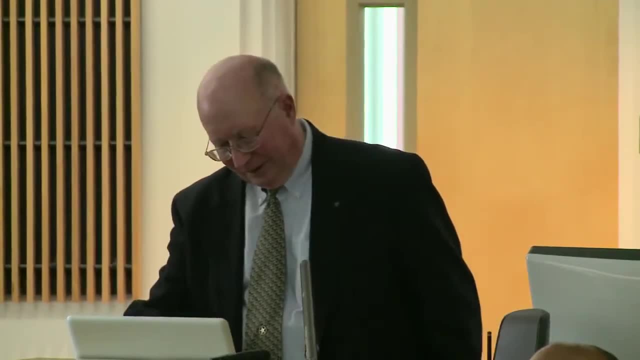 like we were successful. I think that the NRC rankings bear that out, and all I can say is that something went right in those meetings and they lasted a long time and I thought they'd never end, but it was a very, very good thing. What we sort of have as a 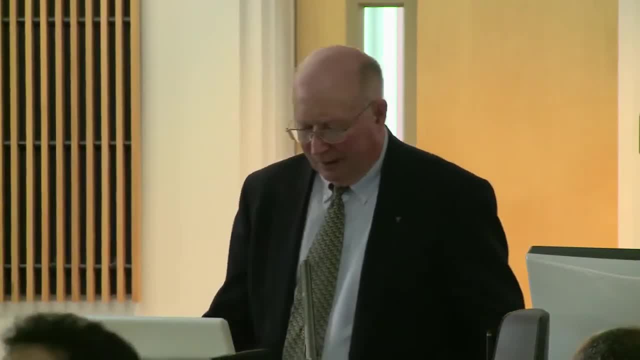 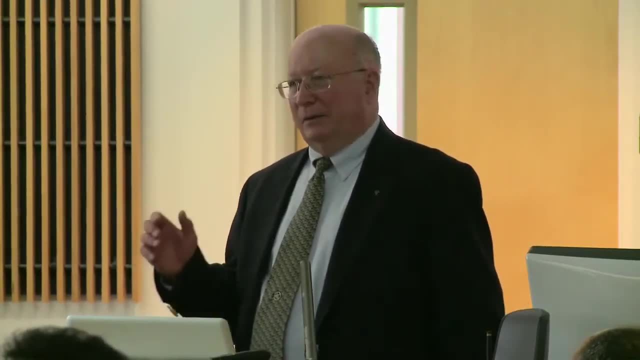 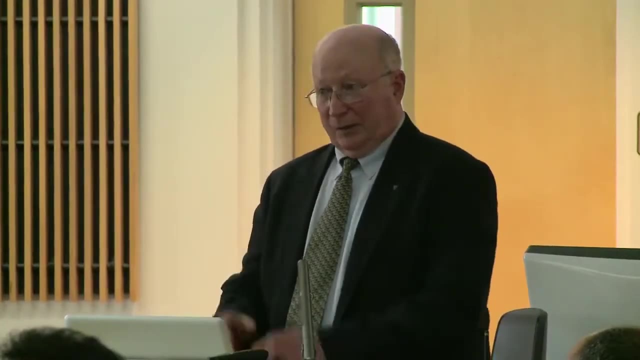 goal for this are stipulations about it. The first thing is that we wanted the speaker to be chosen by researchers- not just the faculty, not just the committee, but by researchers, and so what Mike Goulden did was to set things up so that two research groups each year choose. 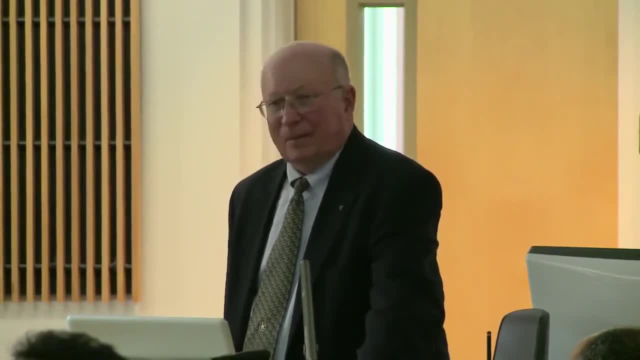 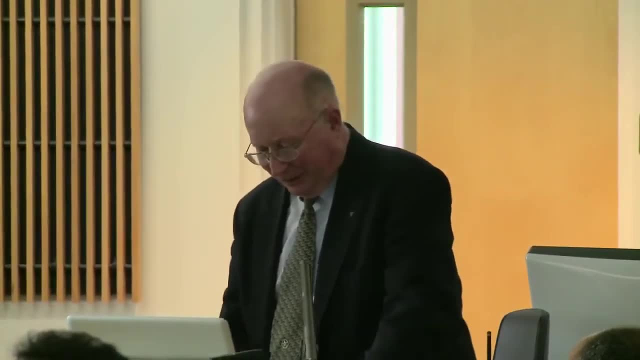 the speaker, and so that I think is a- I call it a piece of administrative parsimony, but I think that he'd have a hard time getting a big committee together anyway. so that was one thing that I think our initial days were people really run from big committee meetings. 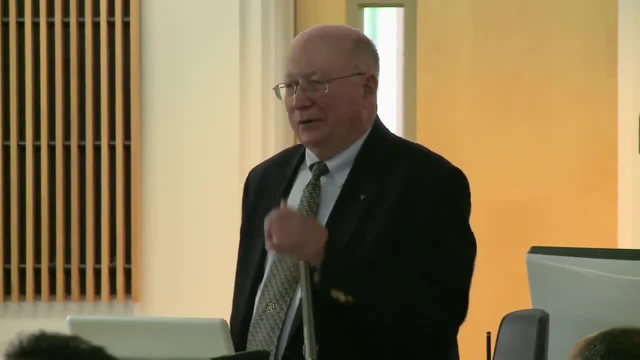 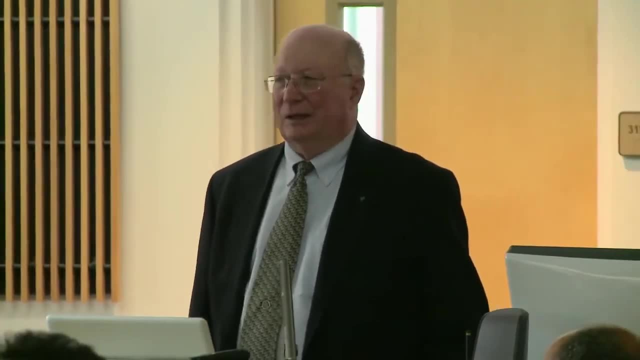 The other thing that we wanted this lecture to have was to have a roundtable. Roundtables are kind of a tradition, if not a hallmark, in ESS, and it turns out that the student roundtables in particular are very effective, and I just heard from a speaker. 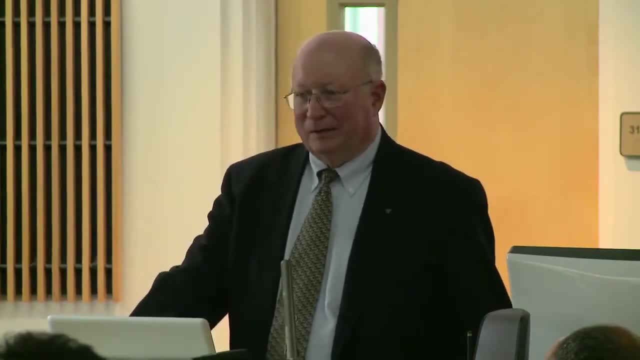 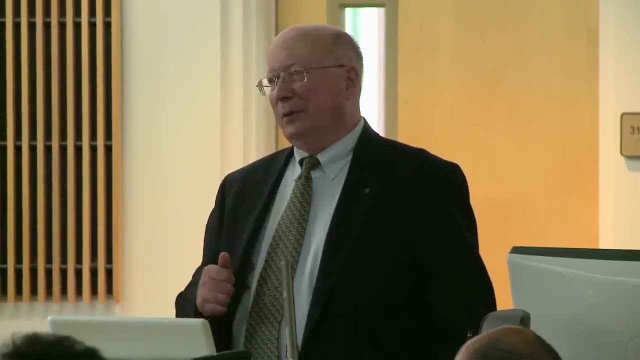 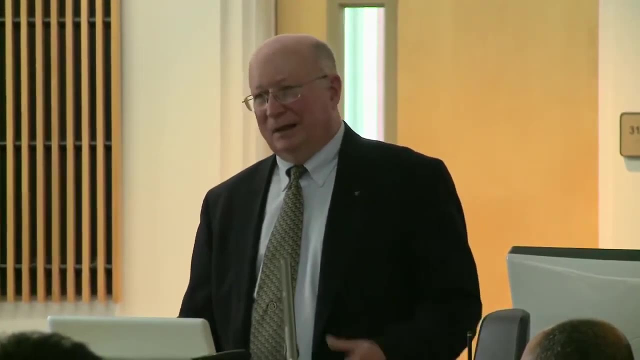 today saying, hey, it was great. so that's another part that we want to have, And the third thing we wanted to do was to ensure that the lecture alternated between modelers and measures. It turns out that, from its very beginning, ESS has always had a constructive 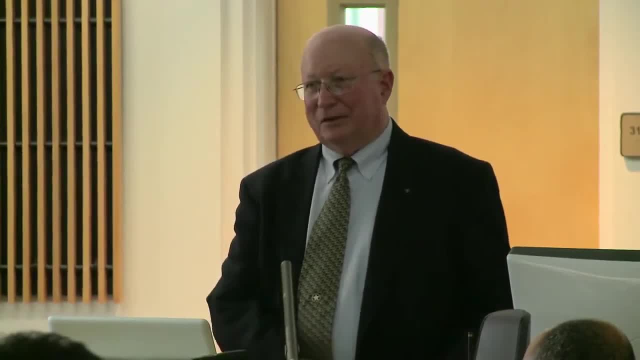 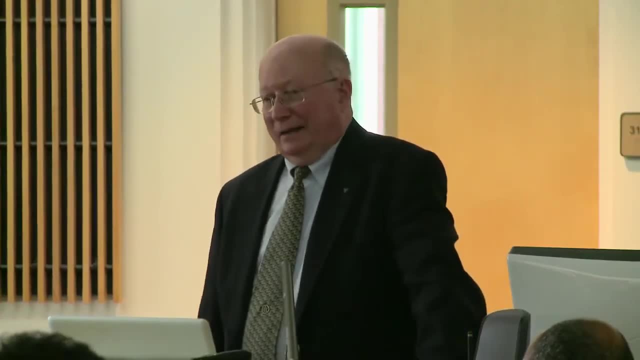 productive tension or balance between theoretical and modeling studies and field and laboratory measurements, and I think this is essential for the field. I think the field is can't, neither can exist alone, and it's important to have that kind of that kind of tension. 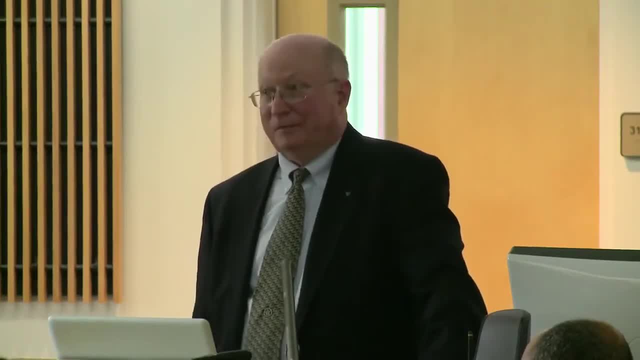 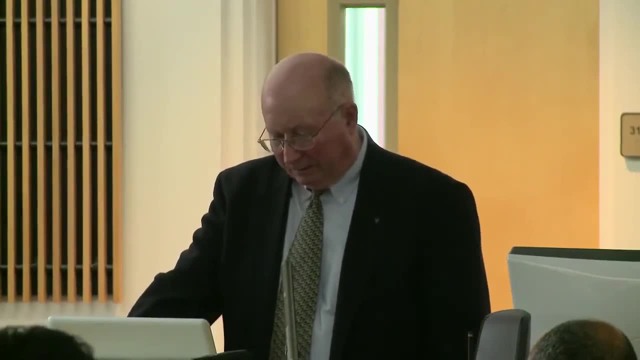 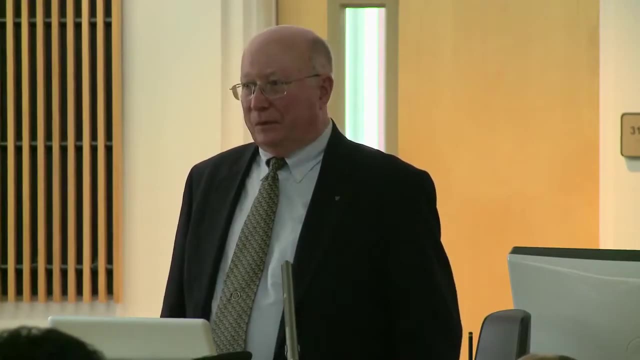 so I think it's a good thing. So anyway, today we have a measure. First, the inaugural one is a measure. So what our hope is that the department and the speakers benefit from this celebration each year. I think this will do, should do a lot to keeping the department together as a cohesive group. 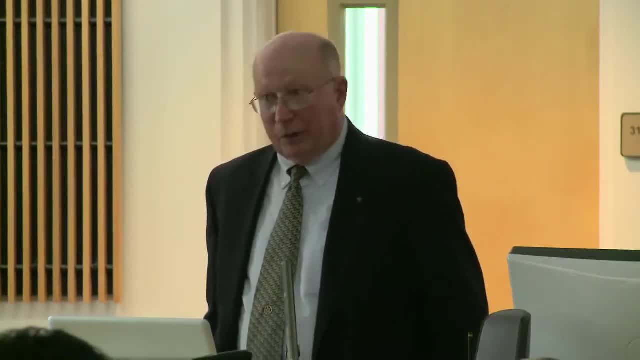 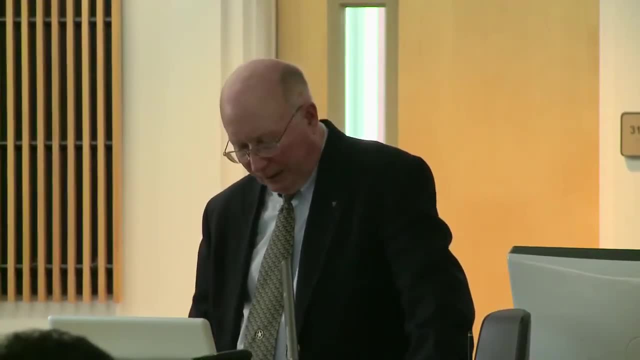 that they're so so well known for a model department in that regard. So we wish you the best. And now to introduce the speaker, Jim White is from the University of Colorado. He was chosen by the Moore and Family Yeti groups as the inaugural Rehberg lecturer. 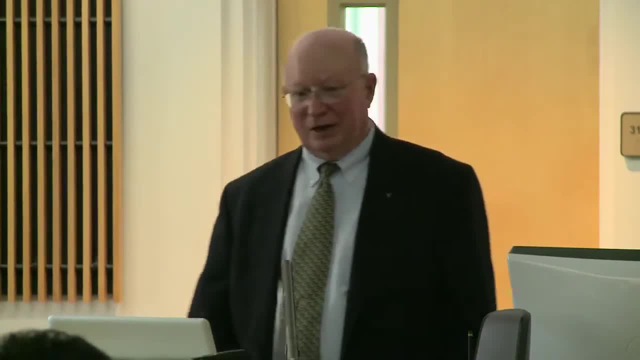 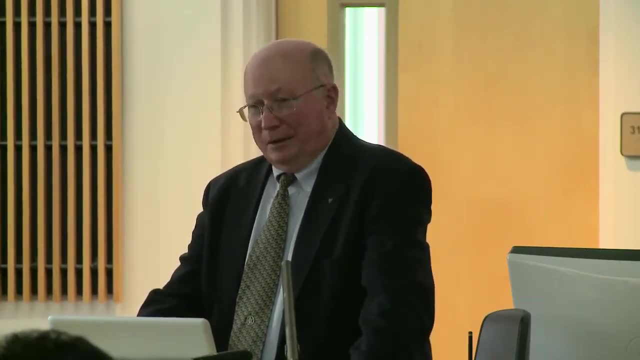 Although it's not present in public public forum any place. I learned last night that he was raised in Tennessee. bachelor's degree in chemistry from Florida State He went to Lamont Columbia University. After Columbia University he spent several years in Europe. 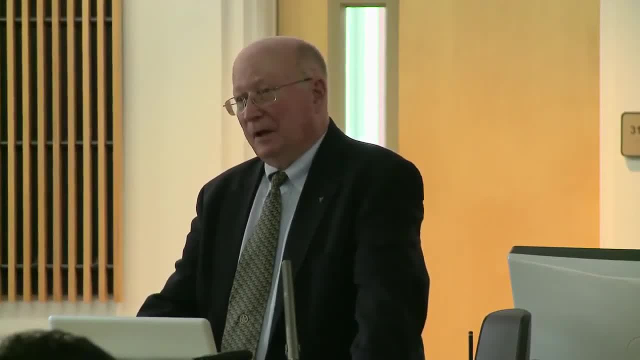 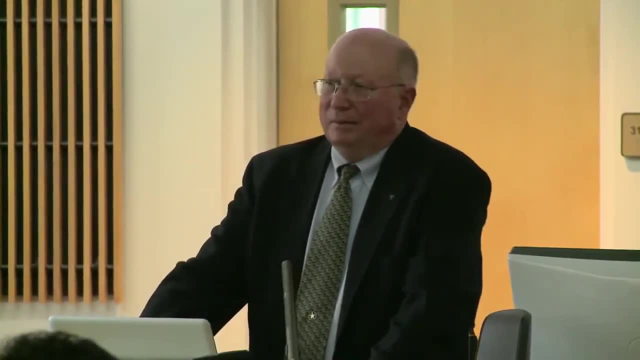 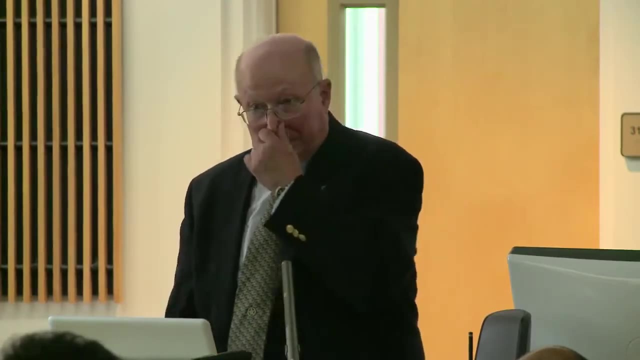 working with the CNRS lab at Gif-sur-Yvette in France, He came to the University of Colorado. He's presently director head of the INSTAR, the Institute for Arctic and Alpine Research. He has academic appointments in geological sciences and environmental science and he's 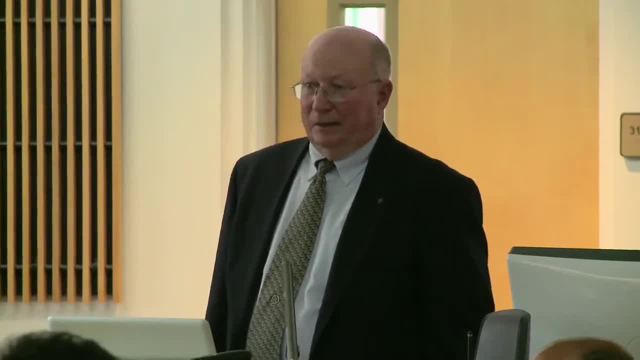 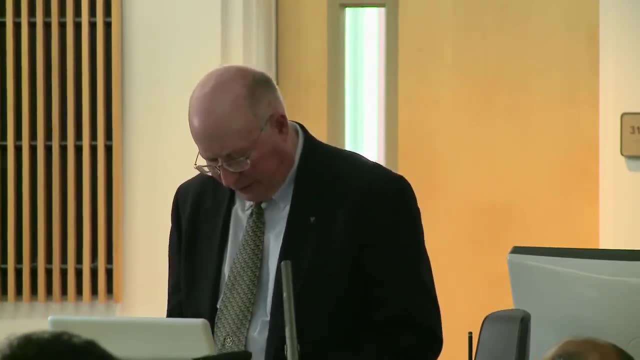 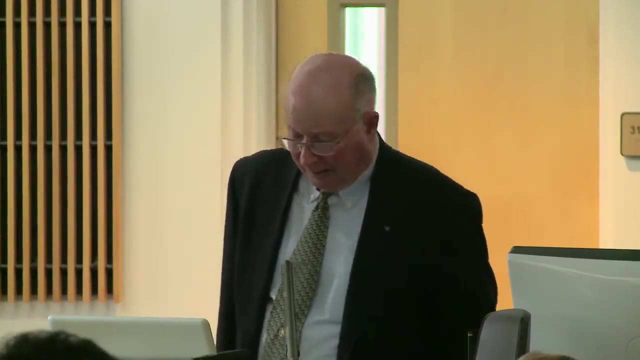 been a big chunk of his time getting this environmental sciences program off the ground, He's. the title of his talk is going to be Ice Core, Sea Level and Abrupt Climate Change. You've probably all seen an abbreviated abstract, but he's going to be talking about the latest. 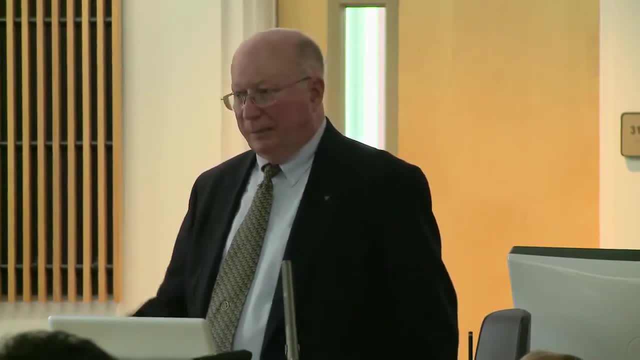 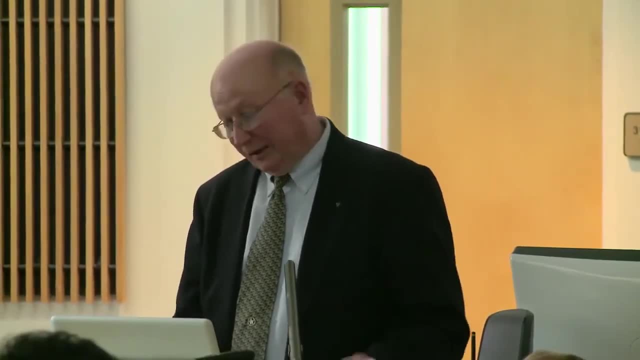 findings from the Neem Core. The Neem Core is one that's a very deep one that basically drilled through the Eemian into the previous glacial period, And so he's got basically going to give us a talk about the results in that core work. So with that I give you. 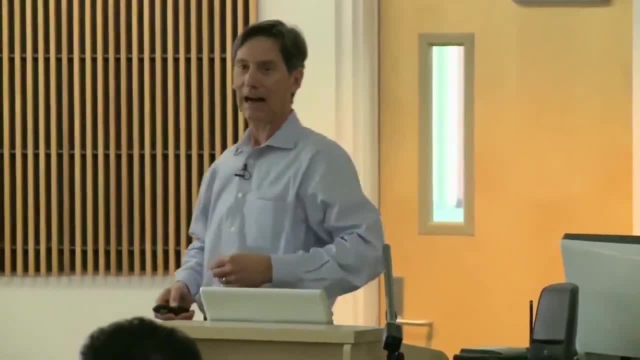 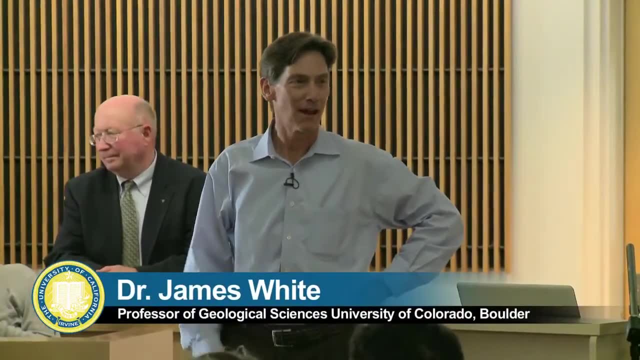 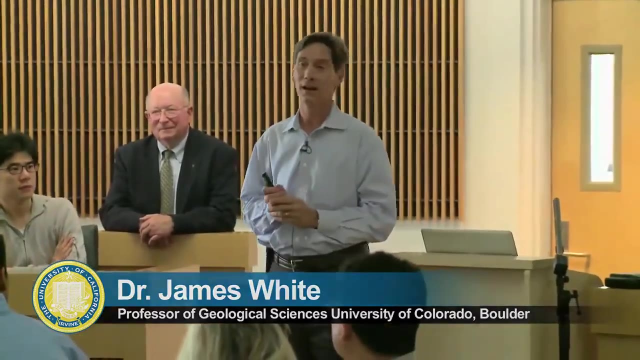 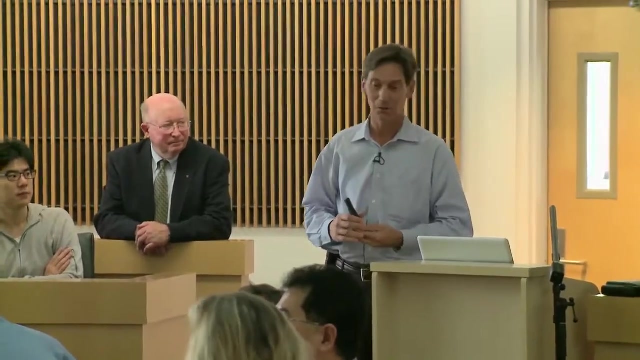 Jim White. Jim White, How does one begin an inaugural lecture? Not that way, Right, You need to be a little snappier. I mean, I am honored to be here, with Jim White to be here. I've known Bill for quite a number of years and he and I have talked about a 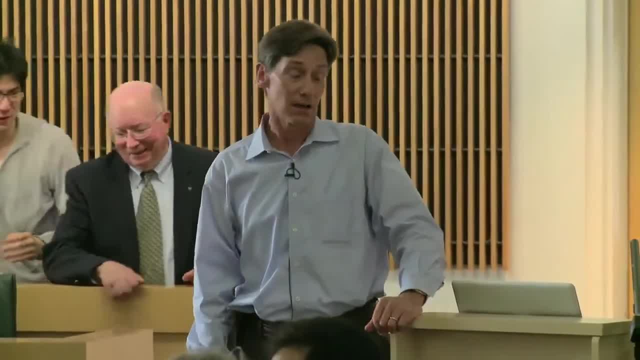 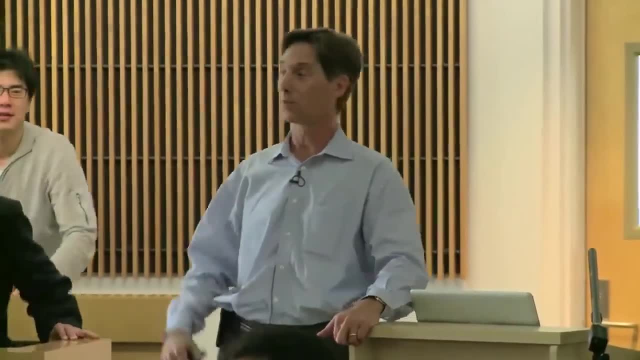 variety of scientific topics, all of our lives, Not all of our lives, but for quite some time, And it is an honor to be here. I think the world of him and I actually think the world of you guys, I mean, I think of you know. there's probably only a few places I could. 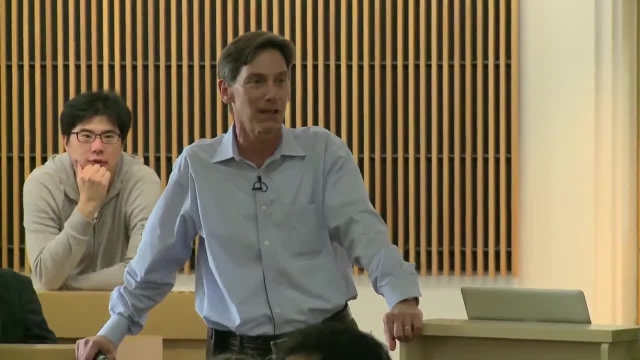 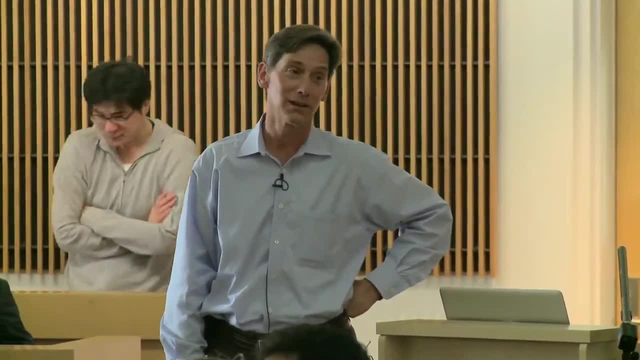 ever be happy, and you guys have one of the best faculty on the planet. This is probably one of the few places that I could find myself really thriving and having a lot of fun. And having a lot of fun as I talk to the students is what it's all about. 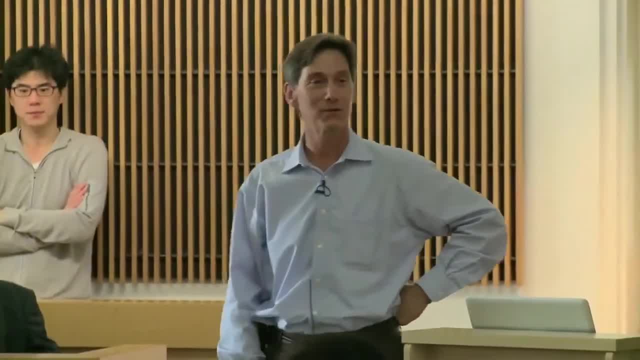 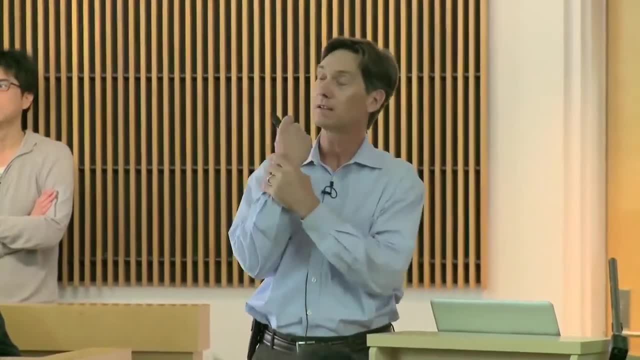 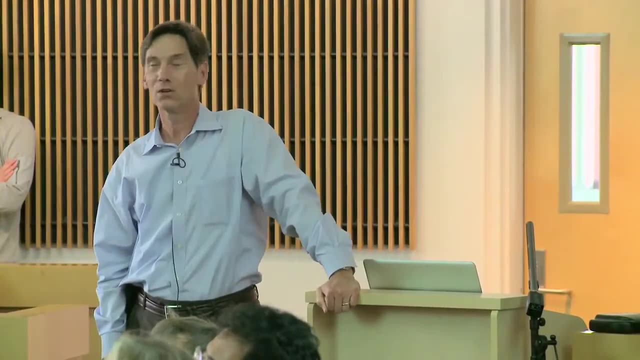 So I don't know how a good old boy from Texas and a good old boy from Tennessee ended up being today's entertainment, but that's what you've got coming. So I'm going to talk to you- basically three talks in one. The first is going to be a look. 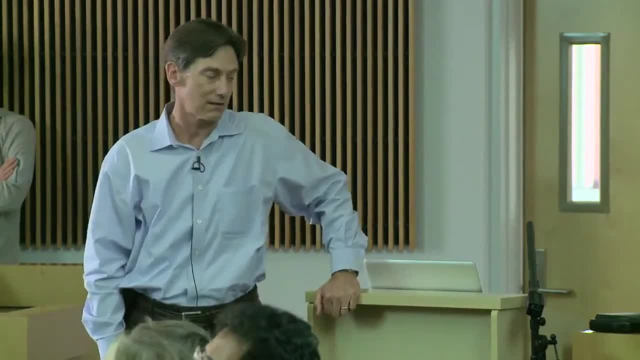 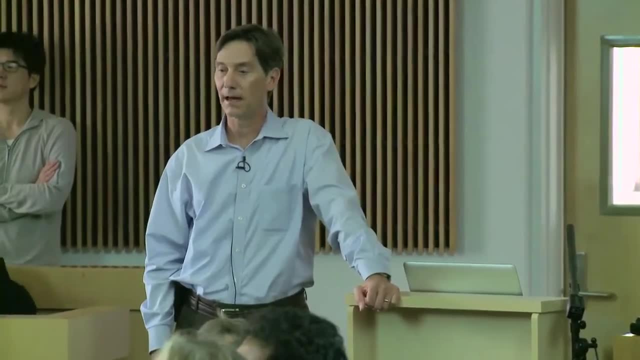 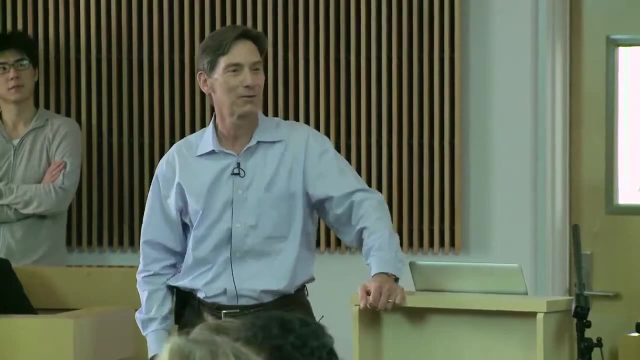 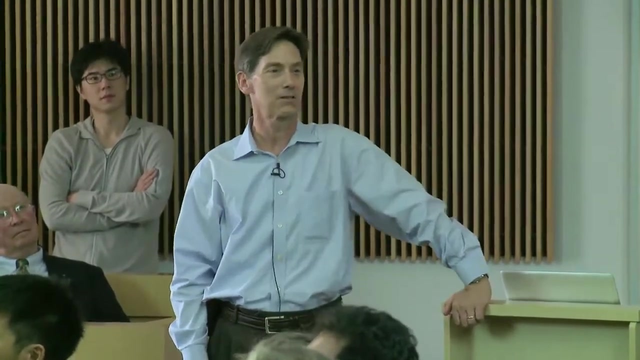 at the latest, The latest information that we have from the last or the latest of our Greenland Deep Ice course, the Neem Deep Ice course. That will transition into a brief but hopefully entertaining midsection, sort of the middle course, on looking at sea level and in particular, 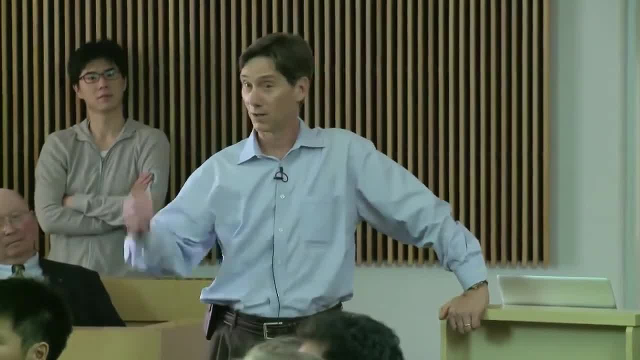 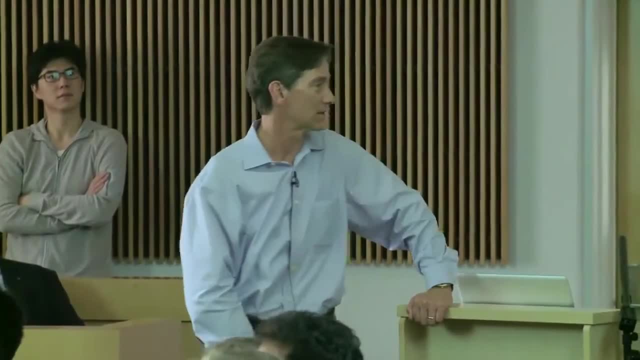 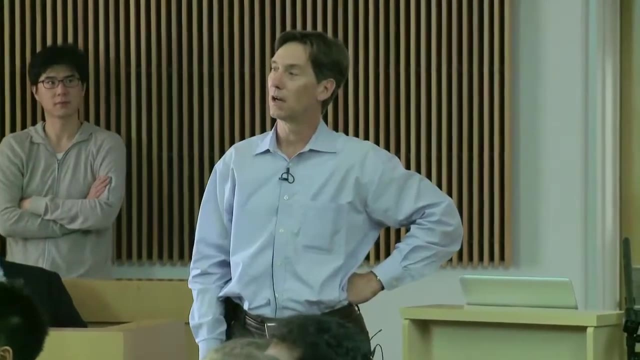 what I like to do when I talk in public about sea level. So we're going to go from a strictly scientific kind of talk to one in which we spend a little time talking about things that I would say were this a public lecture, And then we'll shift gears back to science and talk about abrupt climate change and in 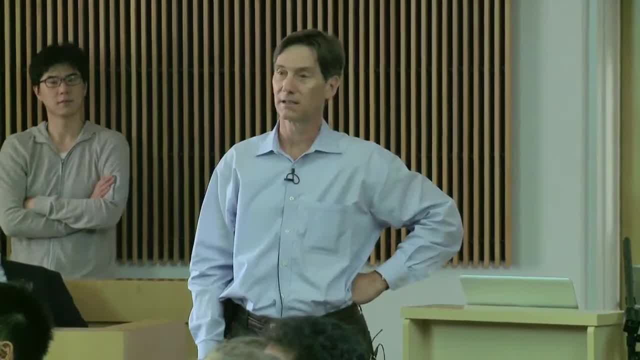 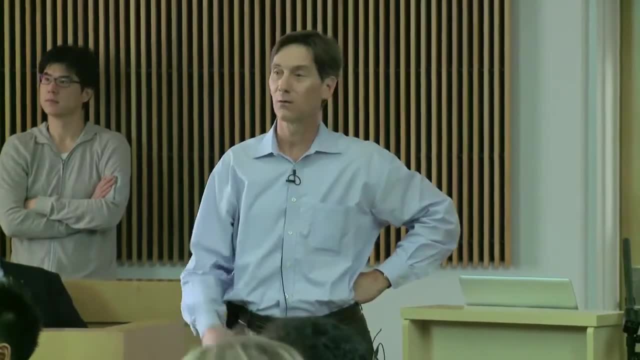 particular, some of the challenges that I think exist in that arena. I would start out by saying I first thank you all. I've had a great time so far and I hopefully you will have a great time over the next hour. I've already had at least one. 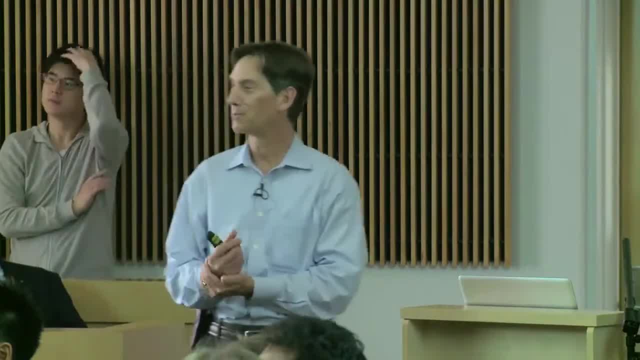 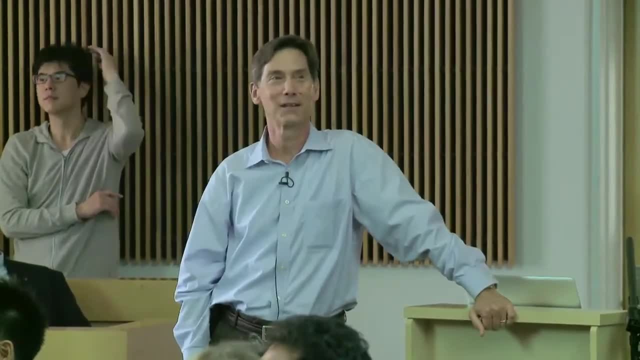 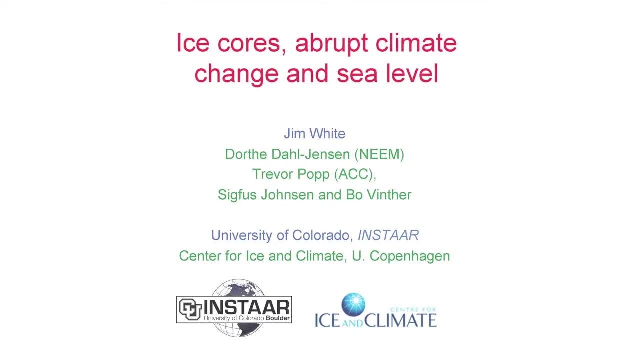 person come up to me and remind me of an event. I had an evening that had way too much wine involved with it in Paris, So you never quite know what's going to happen in life, so just let it roll. I have some co-conspirators on this talk. Dorda Dahl-Jensen is the head of the ice core. 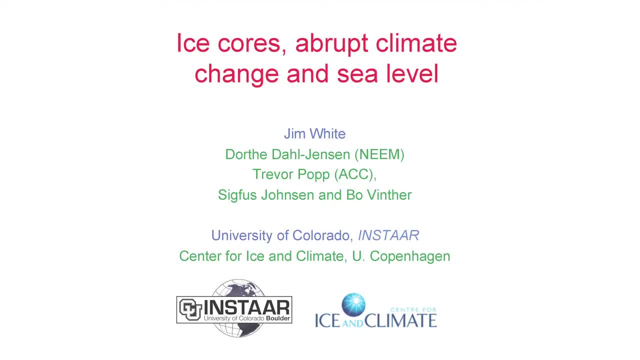 group at the University of Copenhagen Center for Ice and Climate, and she has her fingerprints all over the slides I'm about to show you. Trevor Popp is an ex-PhD student of mine. He and I have worked together for a number of years. We've worked together for a number. 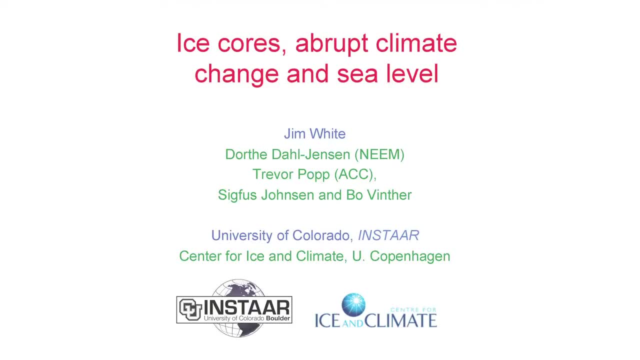 of years We've worked together on abrupt climate change. He now works for Dorda. Bo Venter is the heir apparent to Dorda's lab, And Sigfus Janssen, who I will show a picture here pretty soon, is a very dear friend of mine who just recently passed away, And it 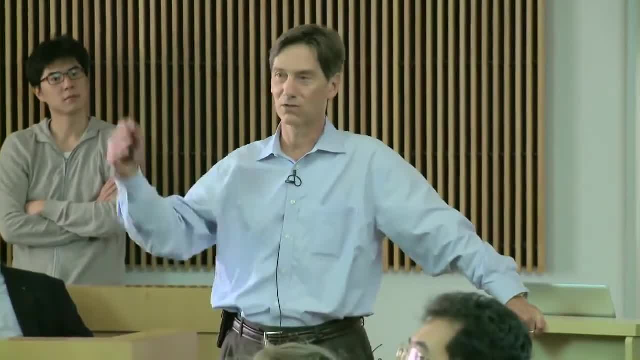 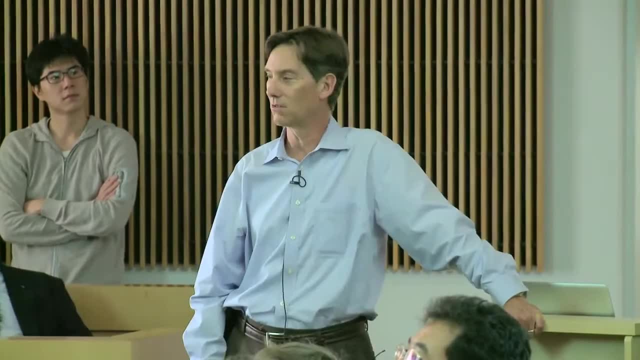 is to him that I owe a lot of what I do For those students in the room. you know that there are people in your lives right now that are helping to shape you and helping you to send you in directions, and treasure that, because those are the people that are going. 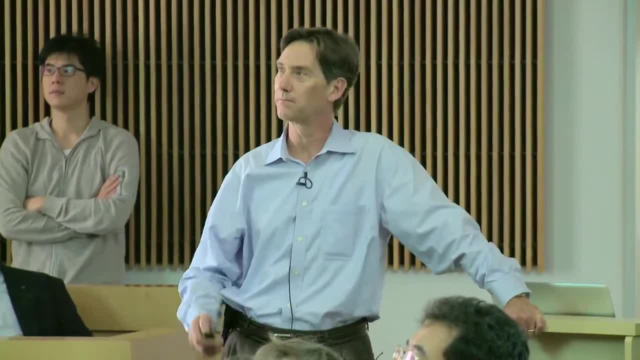 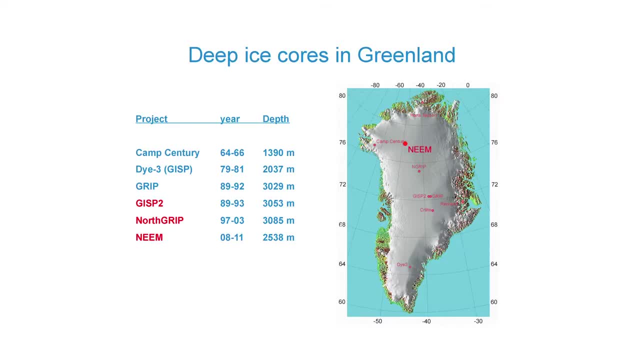 to be lifelong friends, And Sigfus was one of those people for me. So we're going to be looking at the Neem deep ice core. It is important to recognize that we have a series of ice cores now. When I got into this business, the list stopped right here at die three. 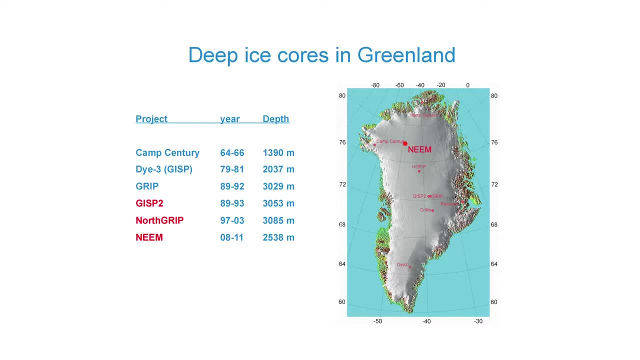 We've added four deep ice cores since then. This is actually a pretty big place. So what I'm going to show you is still very coarse resolution. Still quite a bit about Greenland. we don't understand about climate in Greenland, about the ice sheet in Greenland. we don't. 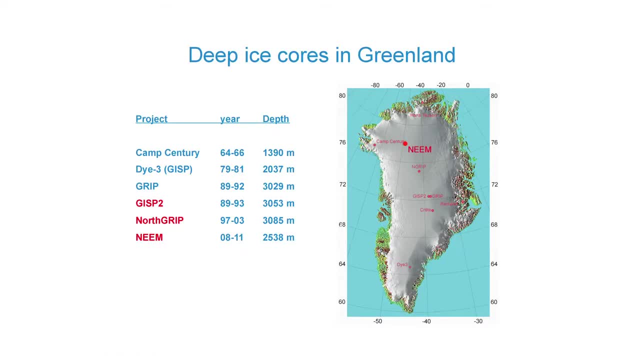 understand And a lot that we need to learn, And I wouldn't by any stretch tell you that we've Swiss cheesed it enough to understand how it works, But these are the ones that we're going to be looking at today. In particular, I want to point out I'm sorry for the print. 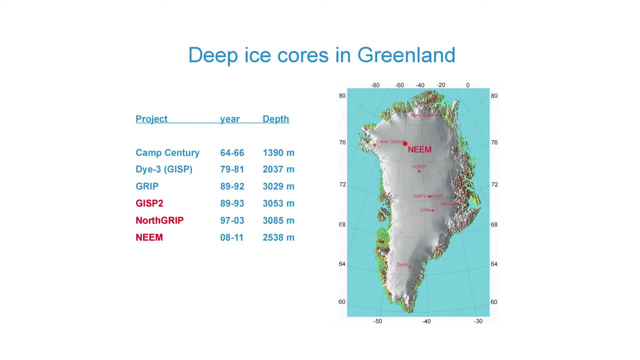 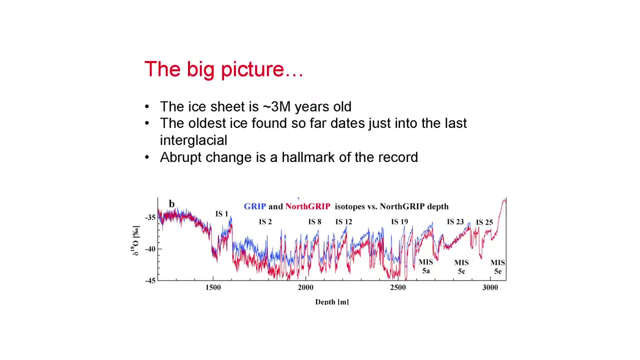 size North Grip here and the Grip and Gist 2 central deep ice cores here. The only one we have in the south right now That goes all the way to base is die three going back into the 1980s. So the big picture. 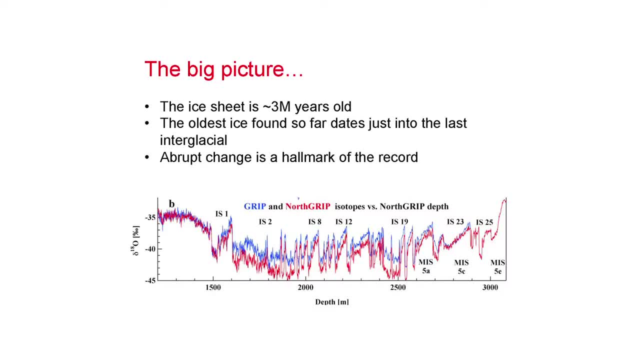 So the Greenland ice sheet is somewhere in the neighborhood of several million years old. We know that from a couple of lines of evidence, One of the probably the best of which is that's when sea level began to change in a way that accounts for that much ice. 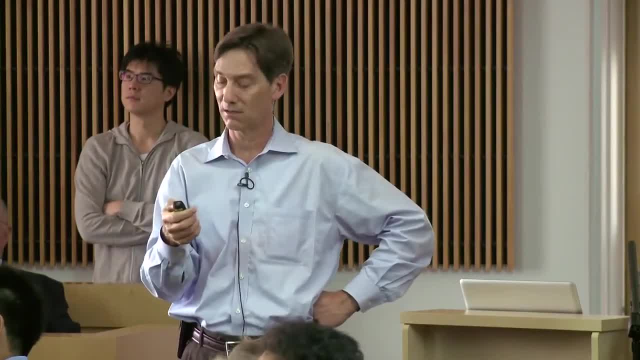 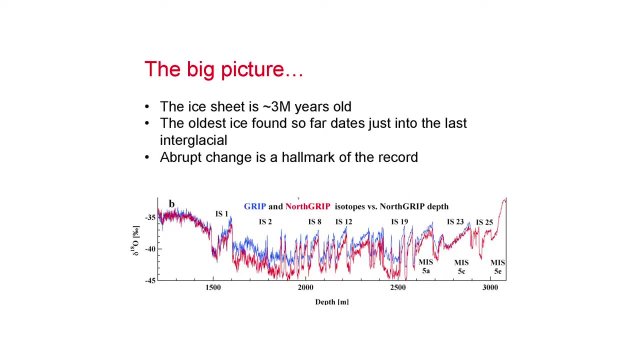 But we have the occasional bits and pieces from the bottom of the ice sheet that give us the confidence of saying it's right around that point. The oldest ice, on the other hand, that we found so far dates just into the last interglacial period. This is the North Grip ice core, shown with the Grip ice core, And you'll see a couple. 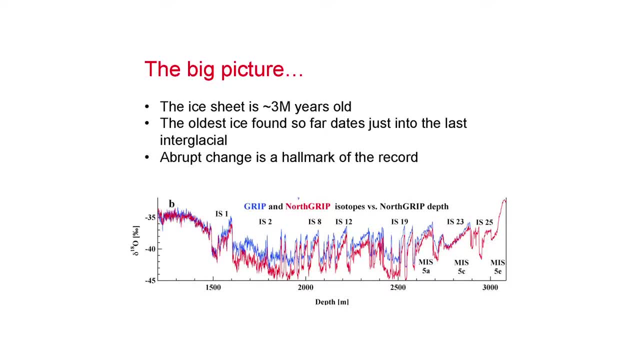 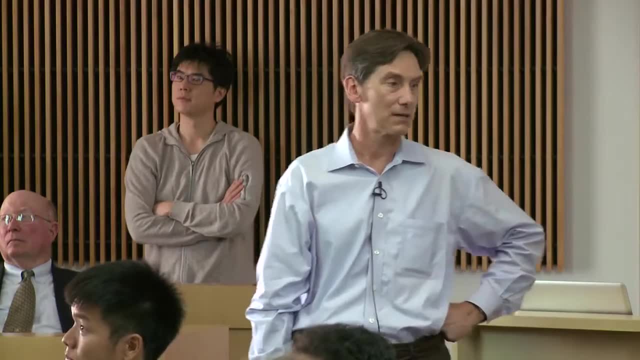 of things on here. One is: I apologize this is not time I have the wrong slide in here, But this is the last interglacial period. We just got into the last interglacial period in the North Grip ice core, A tantalizing little piece of it that turns out to be very 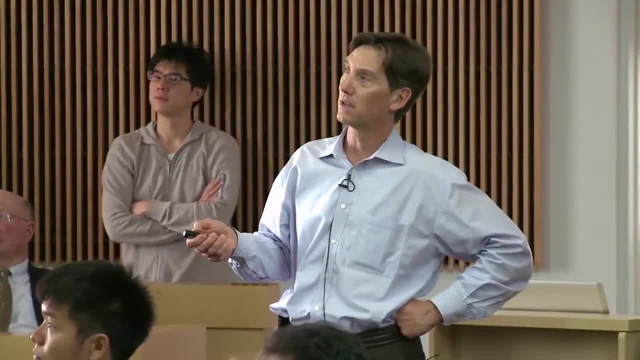 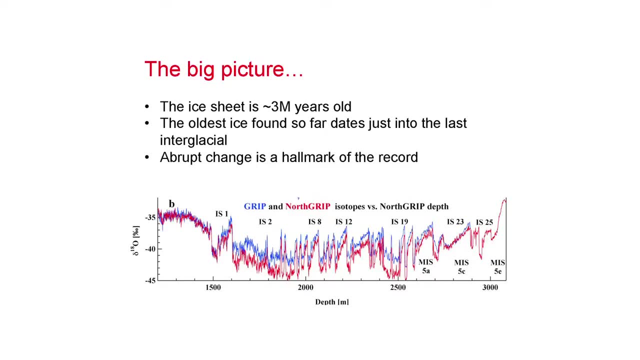 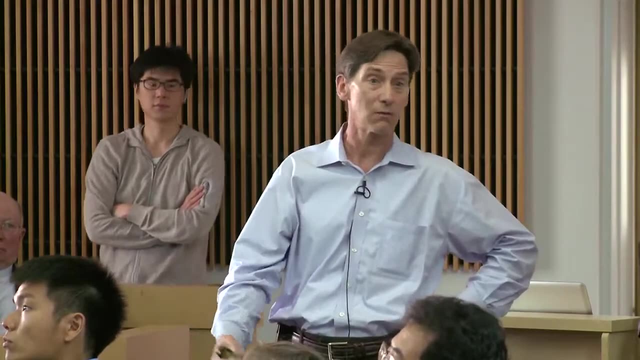 very important for the story I'm going to tell you here. Also note that the abrupt change is the hallmark of this record And as little as 20 years ago, we argued over whether these were climate changes or whether there were some other features that we're looking at in the ice core, Whether there's something wrong with our ice core. 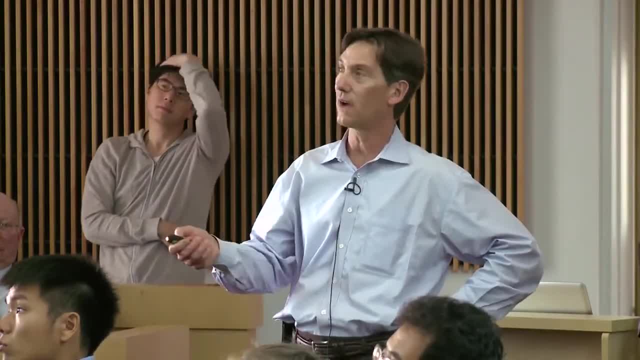 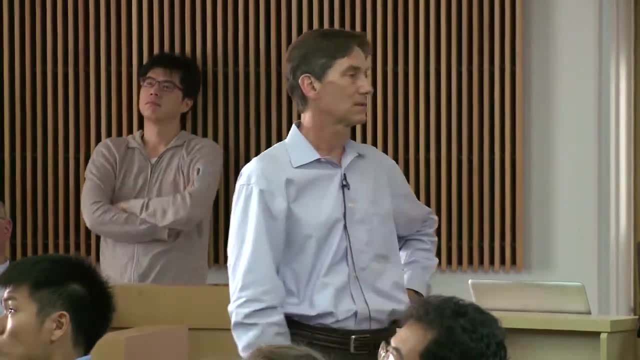 whether or not this was something fundamentally strange about ice cores, It wasn't until we found these changes, not only in many, many ice cores, but we found these types of changes existed in many, many properties that we could measure, Including, for example, temperature. 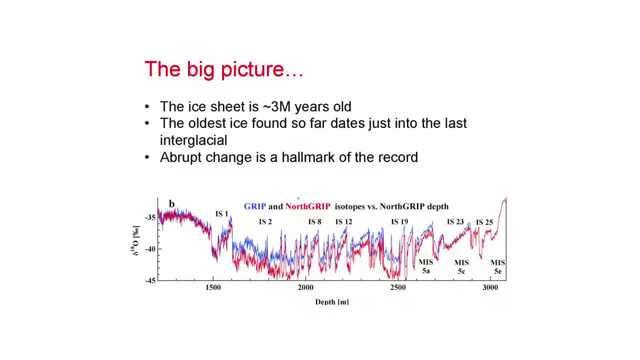 changes That we began to realize, yes, indeed, that these things were climate. I'm going to come back to this, but I want to point these out over here. These are abrupt climate changes that occurred during Marine Ice, Stage 5.. And that's important because we'll come. 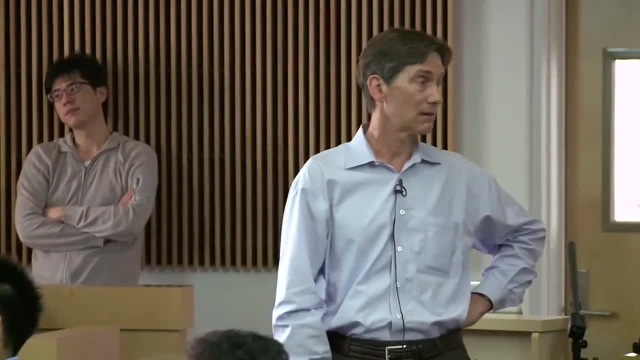 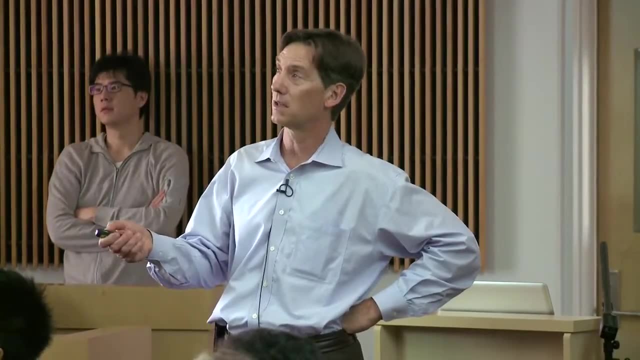 back to that. That's a time of it was cooler than today, but it was- ice sheets weren't enormous- Where this is the beginning of the glacial period. In many ways it's still kind of an interglacial time period. 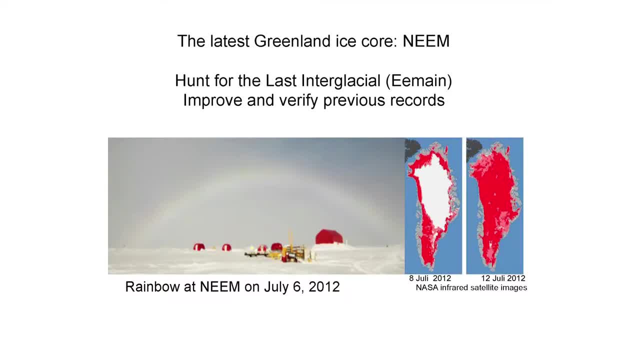 Alright, So what were we after in the Neem Ice Core? In the Neem Ice Core, we had two major goals. One was to look for the last interglacial period, also called the Eemian. The other was to verify- and I'll show you what I mean by that- and improve the previous records. 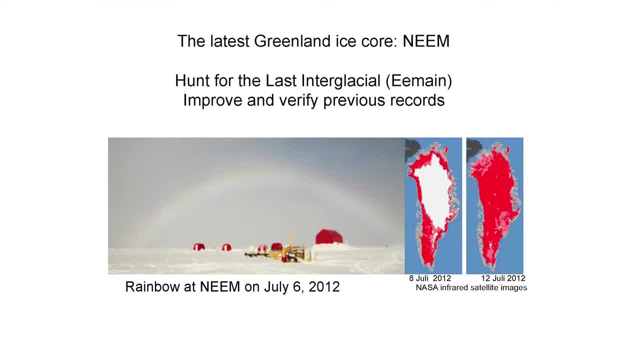 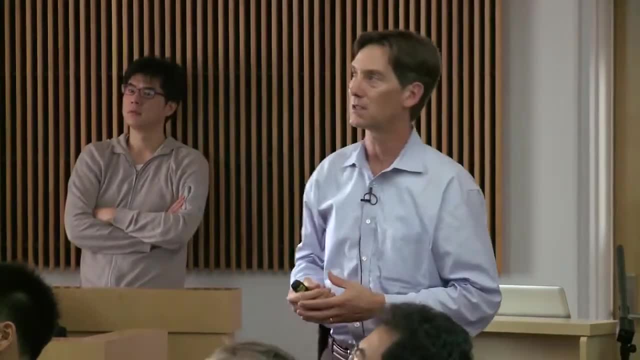 that we had. This is, as I pointed out, the Neem Ice Core is farther north. It turns out there's a north-south gradient in the Greenland Ice Sheet And we had seen this in the other ice cores and we wanted to get some better idea of what that was like. 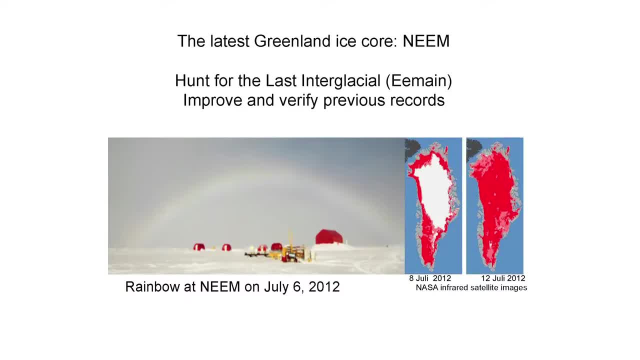 Things have changed. When we first started to do ice coring here, particularly in central Greenland, melting was unheard of, basically, And there's very, very few melt layers that you can see here, particularly in central Greenland. It's gotten much warmer. I don't. 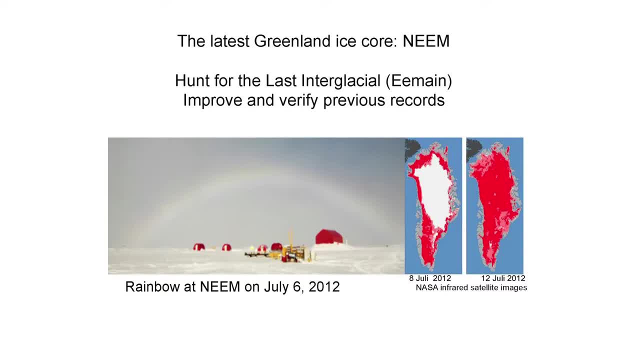 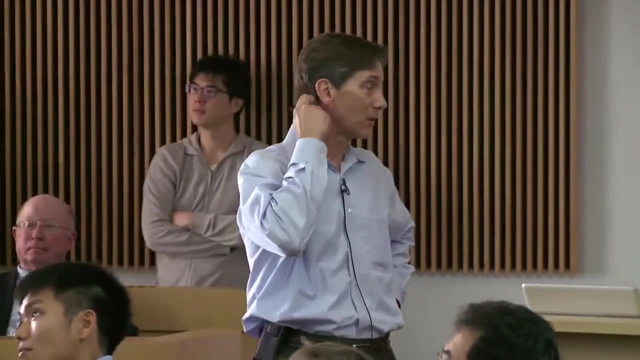 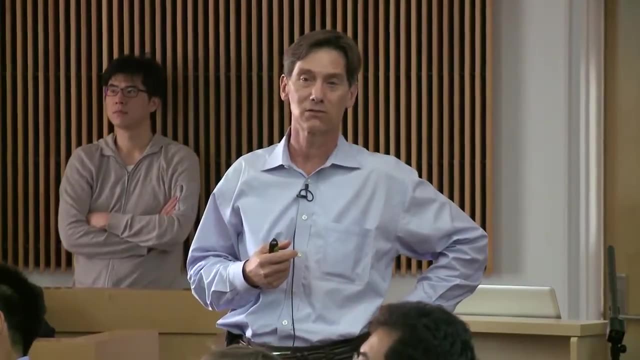 know if you folks have noticed that, but that was a joke. kids, come on, You gotta play along here. It's gotten much warmer and something really interesting happened in July of 2012,: really experienced Greenland Ice Core researchers had never seen before, particularly on top. 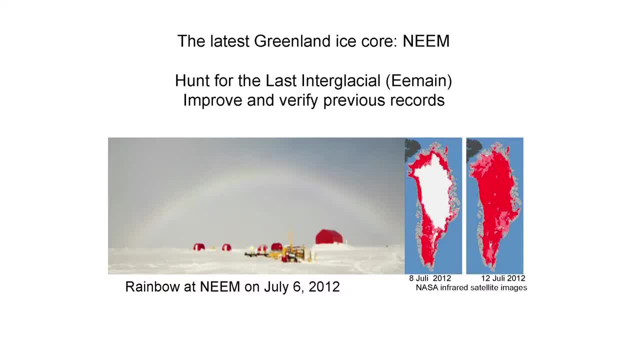 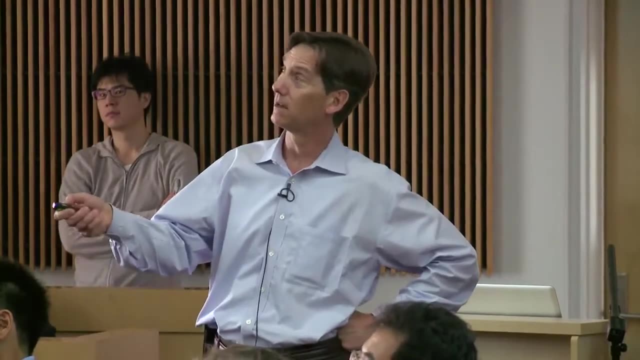 of the ice sheet and that is a rainbow. You see snow bows every now and then, but a rainbow requires some liquid water And that is was a real stunner. It actually rained up at Neem. We had melting of, and on July 12th pretty much all of the Greenland Ice Sheet had surface. 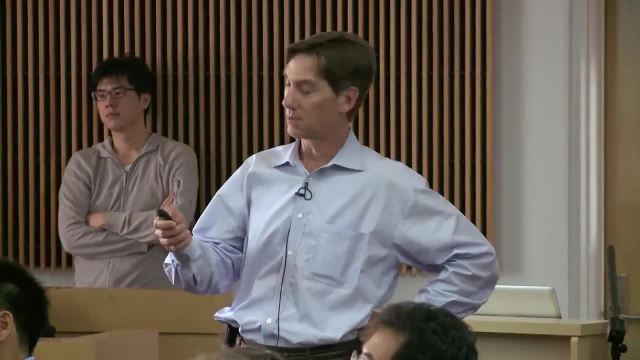 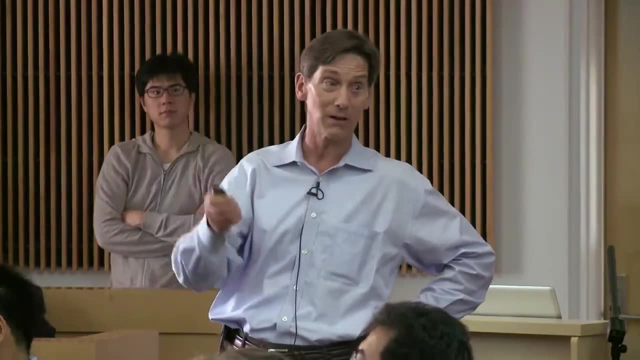 melting, But we actually had rain at Neem. Now this is: this turns out to be a a a. I won't go deeply into it, but this is a fundamental problem for us because we like it cold. We like it cold because the ice we pull out of the hole needs to be cold and stay cold, And 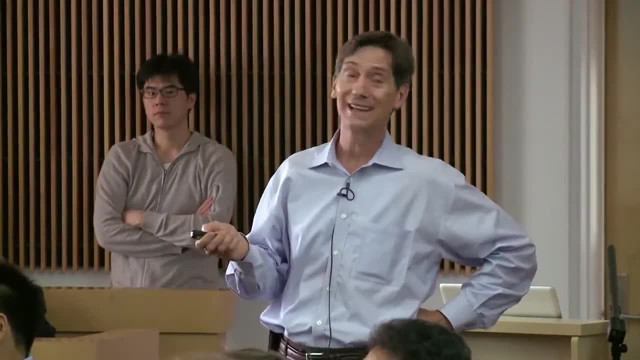 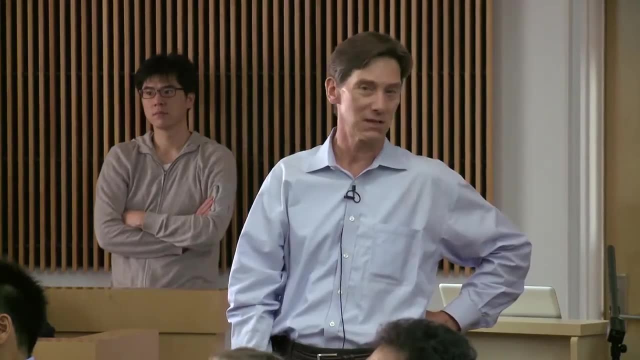 this is a challenge for us. The other challenge for us is that we get in and out of this place in large C-130 Hercules aircraft with skis on them, And for those of you who ski, you know that if you're skiing on snow that's wet and sticky, you don't go very fast And 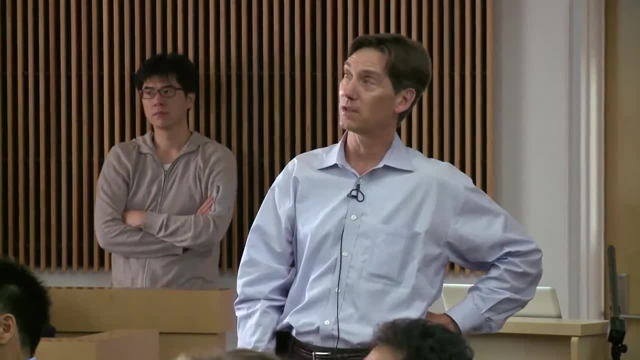 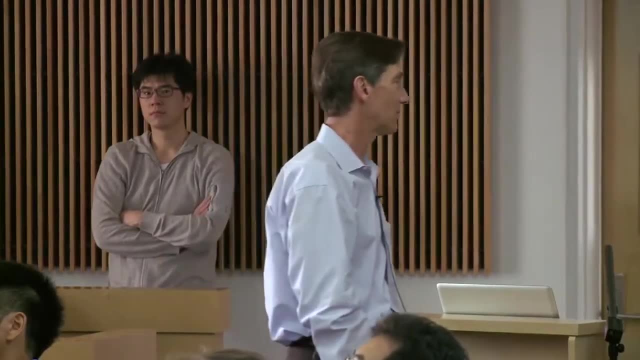 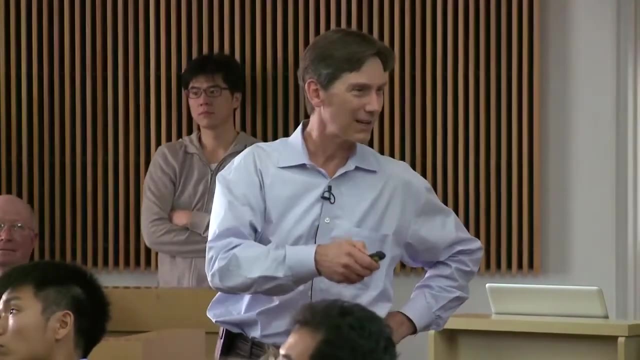 neither do airplanes, And they can do such fundamental things to you as as say: I'm sorry, but there's not enough power to get this airplane off the snow surface. We're going to have to leave you behind, And they do that occasionally. So we have debates about what's more important. 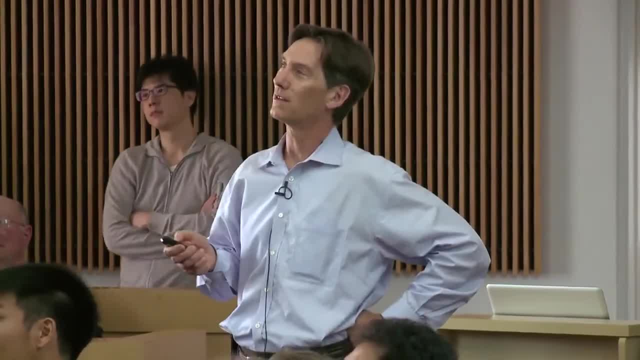 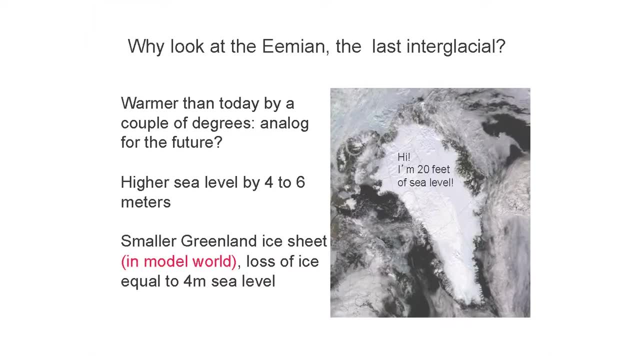 Retrograding ice cores or retrograding scientists? Hopefully we won't get there. So why look at the last interglacial period? It is interesting for a number of reasons, but I think the most fundamental reason, the one that I get most excited about, is that it is one of our analogies. 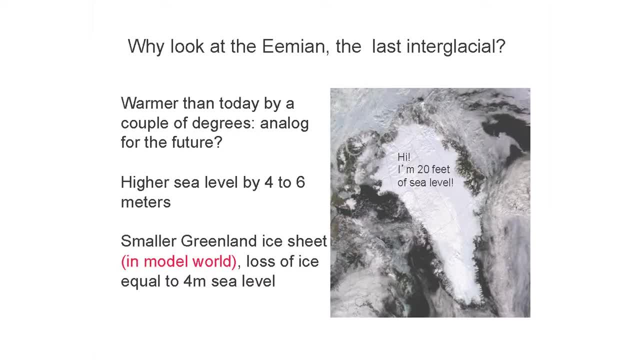 for the future. We have a couple of analogies for the future, but this is one of them. We're looking at a time period of roughly 120,000 to 130,000 years ago, It was warmer than today by a couple. 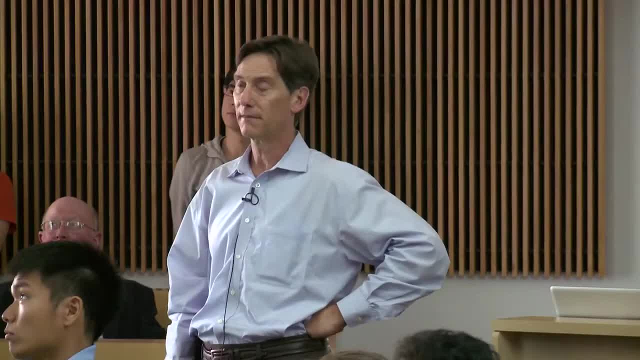 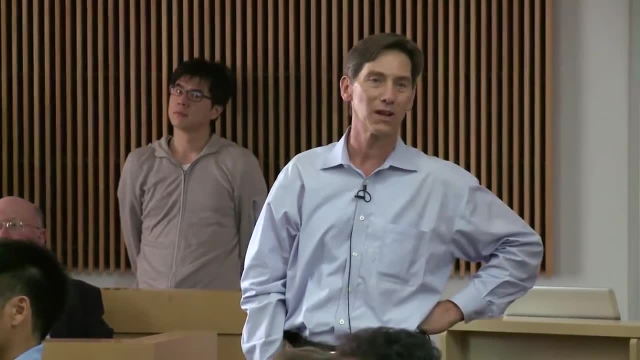 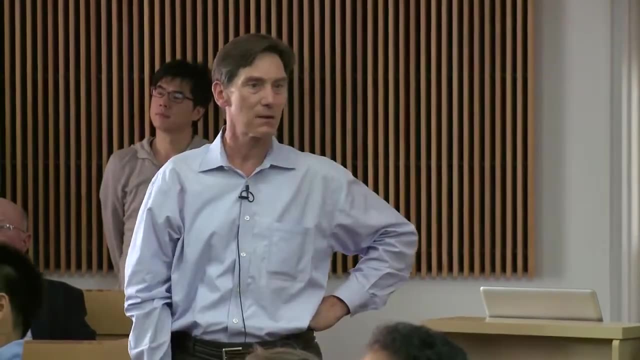 of degrees, which is obviously an analog in a sense, in that we are in a warming world. Sea level was higher by something in the neighborhood of 4 to 8 meters, And I'll show you some other numbers there, And that's where we're going as well. As time goes by, sea level is rising. 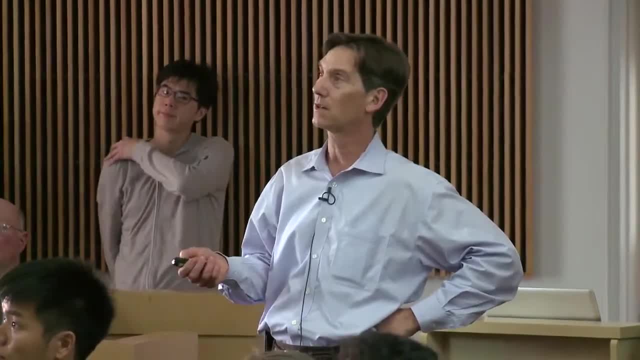 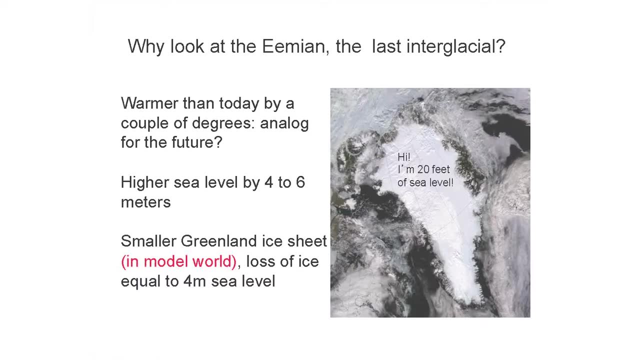 today. It will continue to rise today. We'll talk about that. in the mid part of the talk And there was a smaller Greenland ice sheet- And I say in model world because we don't really know- This is what we were after in the NEM ice core. Could we indeed say something about the size of this ice sheet? 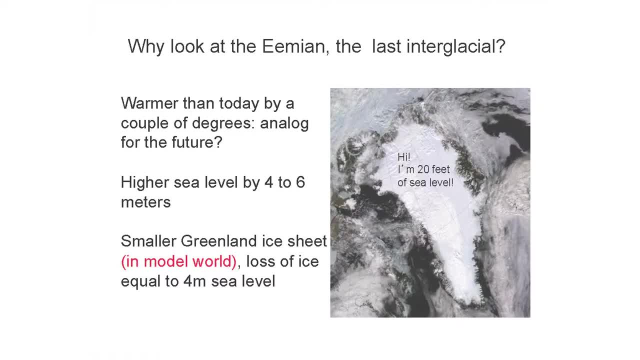 in the past And the speculation was there was a loss of ice somewhere equal to about 4 meters of sea level rise. So can we indeed verify that, And that's what really we were after in the NEM ice core, Slide 10.. 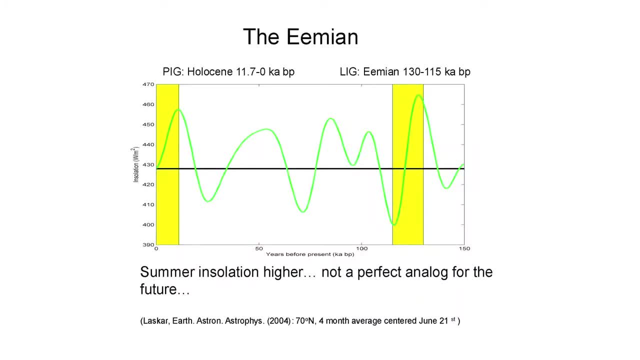 Slide 11.. Slide 12.. Slide 13.. Slide 14.. Slide 15.. Slide 15. Slide 16.. And this just shows you that the last interglacial period is not a perfect analog for the future. It was warmer because summer insulation was higher, not because greenhouse gases where? 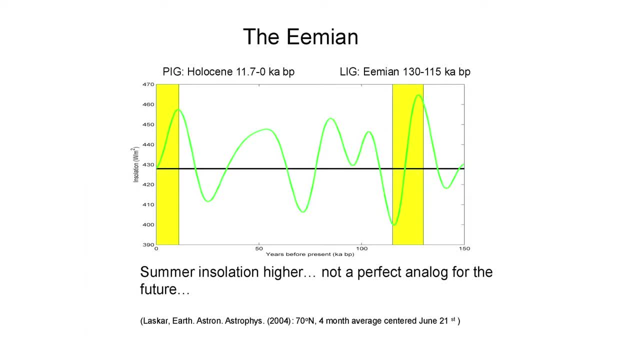 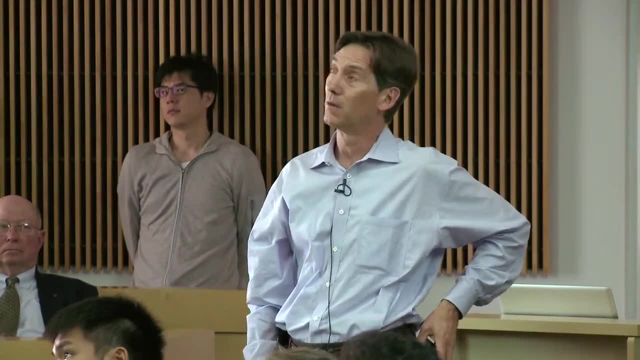 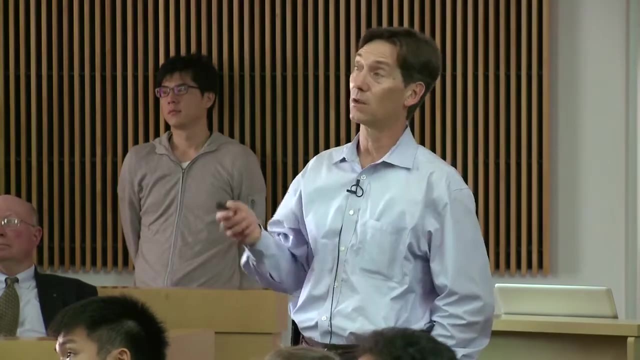 higher Greenhouse gases were maybe around. CO2 was about 300 parts-per-million, so it wasn't much above the 280-ppm baseline that we see for the pre-industrial period. So it's not a perfect analog, but it's still the best shot we have. It's the closest analog in the 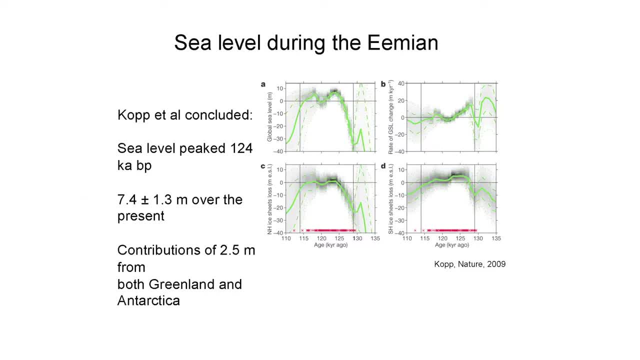 past, Sea level during the Eemian was higher than today. as I pointed out, There have been a number of studies recently, In 2009,, Kopp et al did a statistical study where they took all of the observations, put them together and estimated that sea level peaked, as I say here, somewhere around 124,000 years ago. 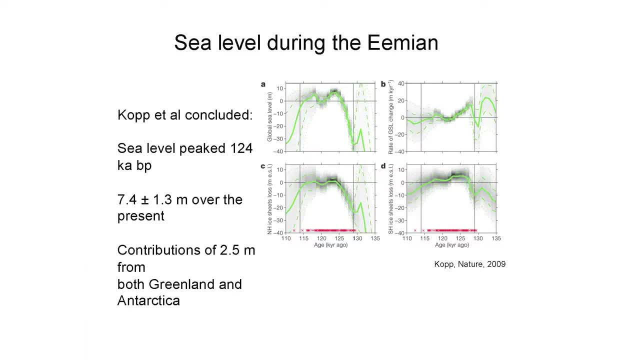 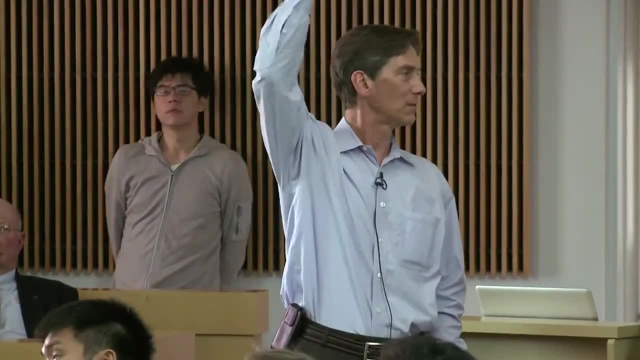 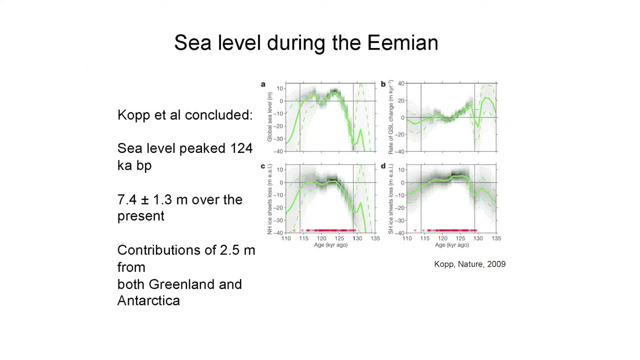 Roughly seven plus or minus one meter higher than the present. For those of you who have been to the coast, imagine seven meters above you, Imagine 20-something feet above your head. That's where sea level was. And they concluded there were contributions of something like two and a half meters from both Greenland and Antarctica. 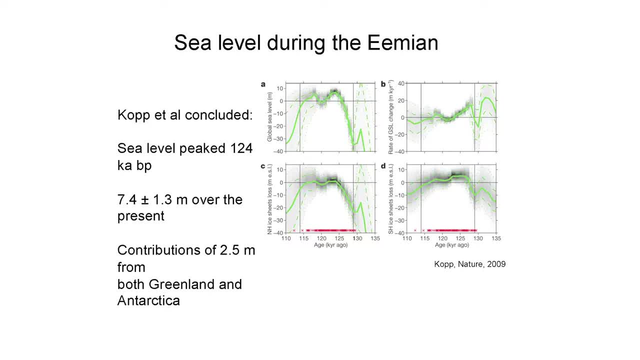 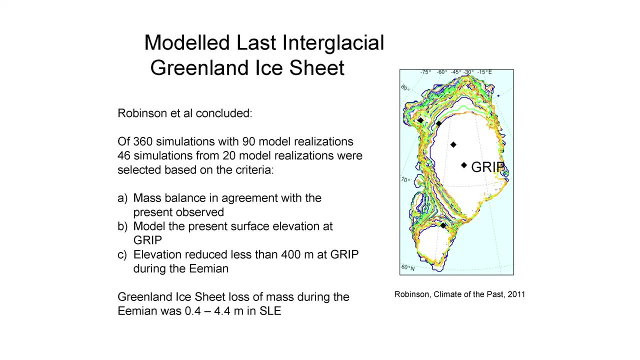 And that's important, and I'll stress why that is true in a few slides. So there have been a number of modeling studies that have looked at the Greenland ice sheet, A recent one by Rossi Robinson and group in Climate of the Past where they looked at various realizations of the Greenland ice sheet. 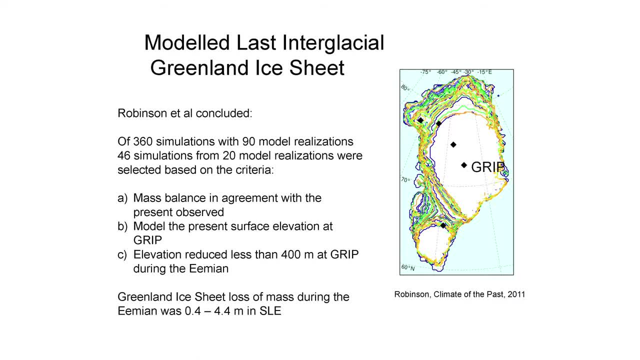 In this case they took, as it says here, 360 simulations, 90 model realizations, And of those they took, 46 simulations from the 20 model realizations were selected based on the criteria. you see here that mass balance was in agreement with the present. 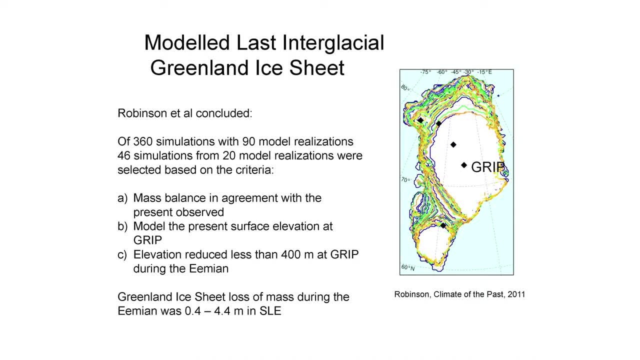 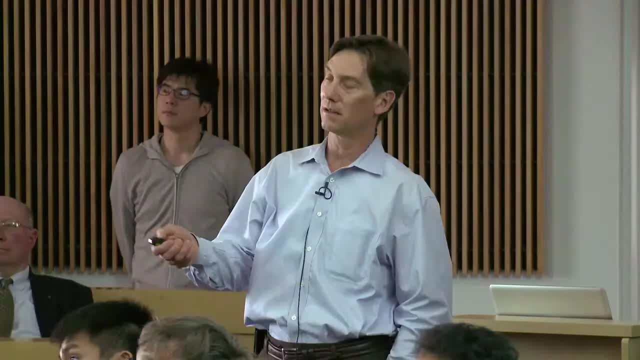 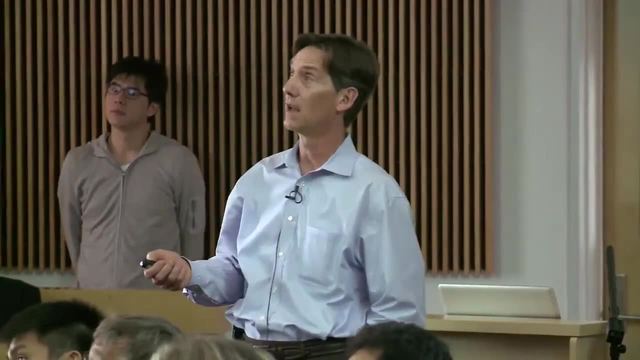 observed the model. the surface model had to be right at grip, which was the center of the ice sheet here, And there had to be no really large loss of ice as some models get when they look at the Greenland ice sheet in the past. 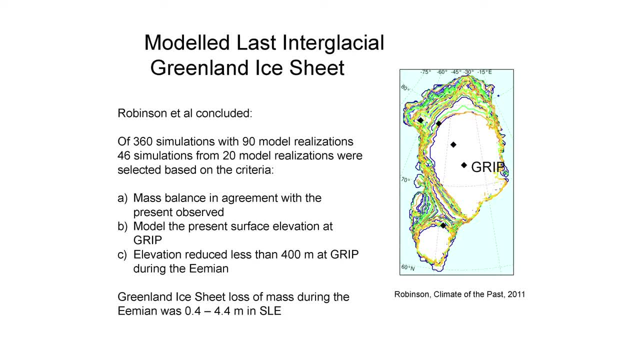 And these are typically models that are driven primarily by insulation and by greenhouse gas levels. So you're looking at, basically, the impact of summer insulation on the Greenland ice sheet. So the conclusion was that the Greenland ice sheet lost mass and was somewhere in the neighborhood of about the same. 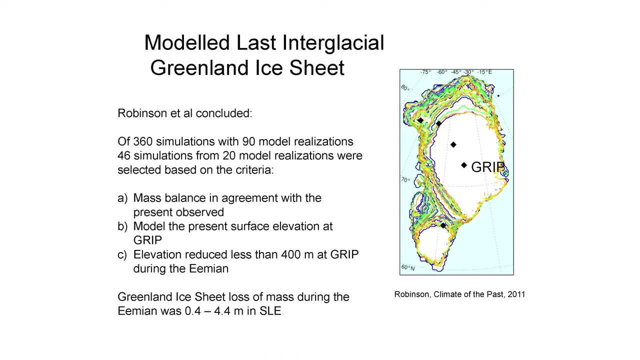 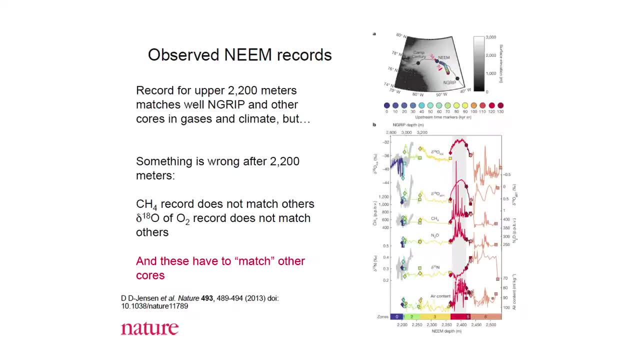 which is 4 meters sea level equivalent- less in its mass in the past, So roughly about the same as that 2.5 meters that we see here. So what did we observe? One of the interesting things was we were able to measure the ice core in the field for the first time. 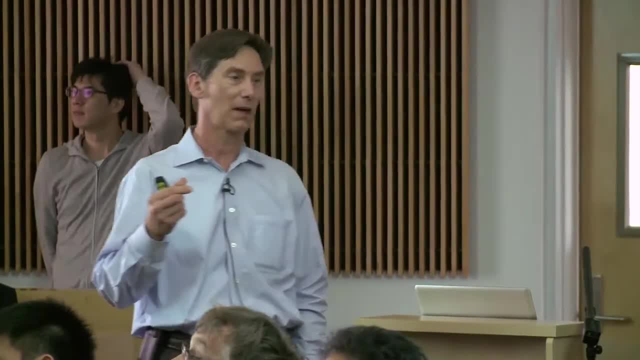 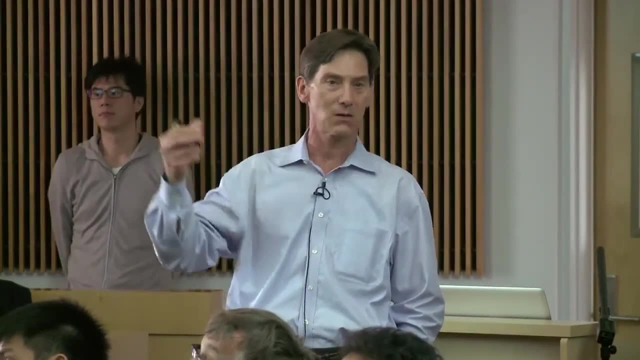 And I'll come back to this, but this was a breakthrough. We have what we call continuous flow analysis. So if you've never been on an ice core site, we take the ice core, take it down, right out of the drill. We let the liquids evaporate off the surface of the drill fluid. 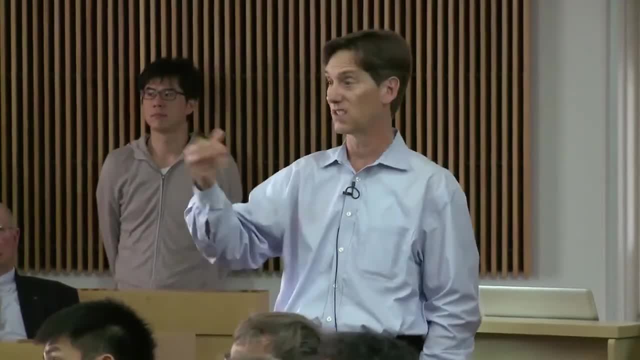 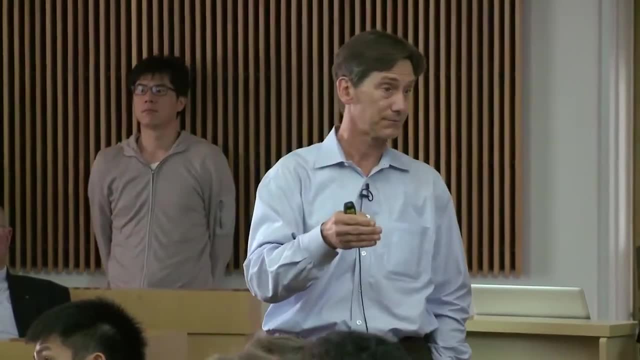 Then we take it back and if it's cuttable, that is, if it's not in the brittle ice zone- and you can get into that detail if you want. But basically then we slice the ice core and we begin to analyze it. 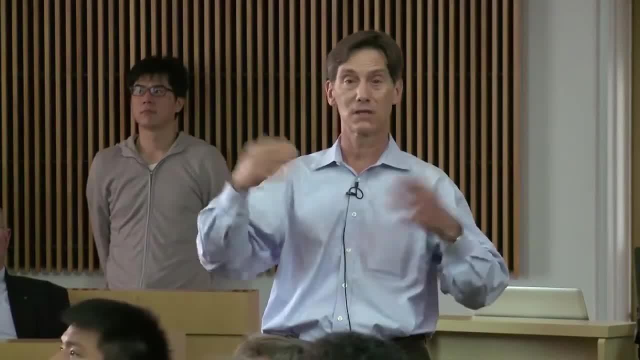 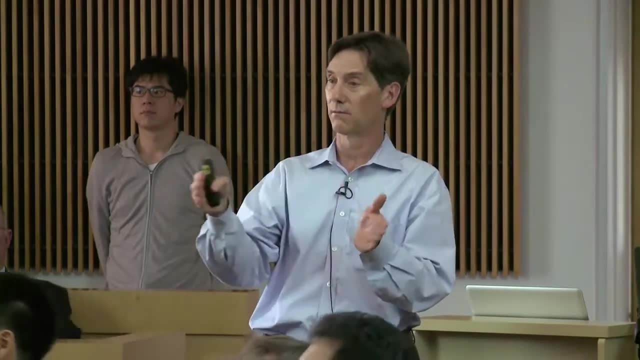 Right then. and now we have what we call a continuous flow analyzer that measures chemistry. It's a melt head. We just take a stick of ice, put it on top. We can also measure stable isotopes. So in real time we know where we are in the ice core now. 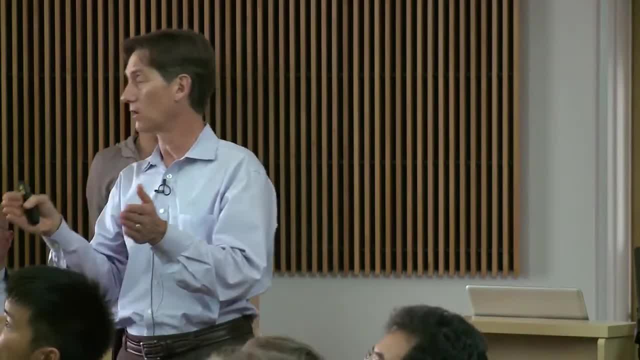 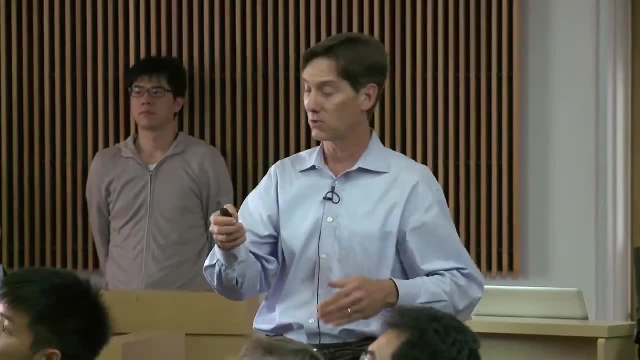 And that wasn't true in the DI-3 ice core and it wasn't even true in the GIF-2 or GRIP ice core. This is only in the past couple of ice cores have we had the capability of knowing where we were as we were actually measuring this. 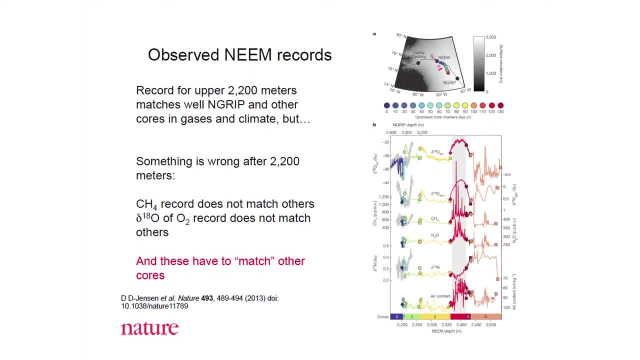 So we knew that up to about 2,200 meters everything was right, because it looked just like North GRIP, or not just enough like North GRIP that we knew everything was pretty normal. Past about 2,200 meters, things began to change. 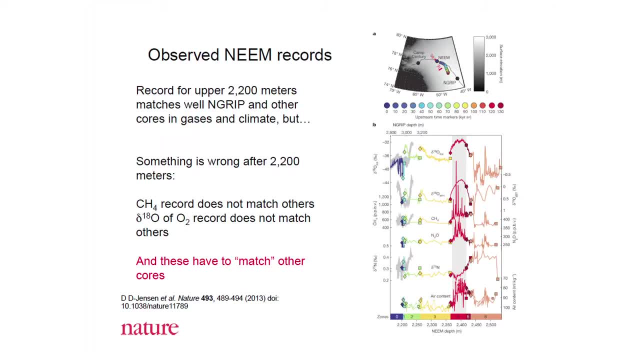 Things began to get really weird, And this is the actual records here. You see, the O-18 of the ice was cruising along. The colors are color-coded for a reason you'll see in a minute, But obviously they weren't color-coded when we got them. 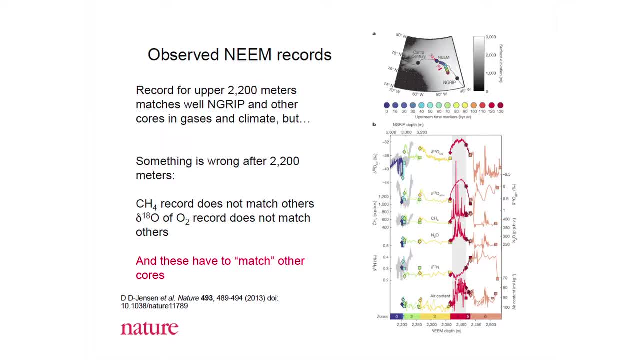 And so they were cruising along. We saw what we thought was a pretty clear chunk of the emian. There was some craziness down here at the bottom, things bouncing around And then we hit bedrock. The second analysis you see on this, which is important, was the del-O-18 of the atmosphere. 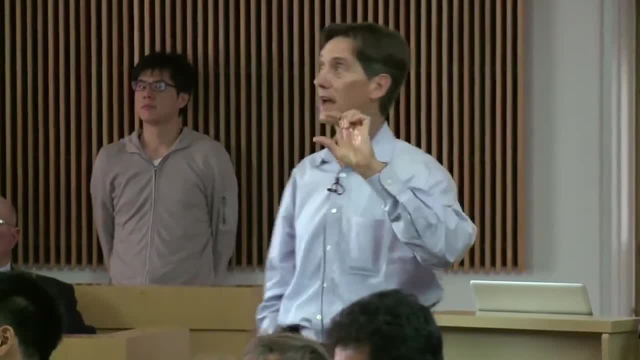 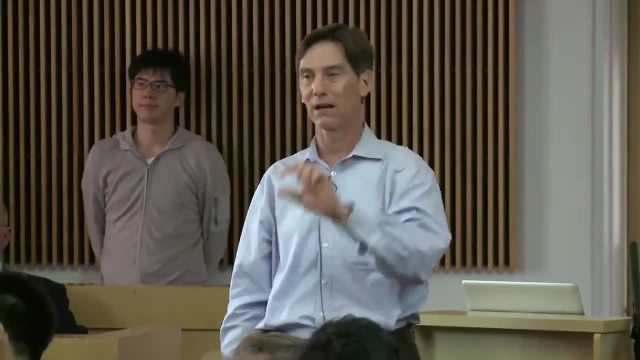 So the oxygen-18, oxygen-16 of the O-2 of the atmosphere. That's important because that's one of those measurements that has to be the same in all ice cores. So if you measure it in Antarctica, since it's a common atmosphere and the atmosphere is quite well mixed, 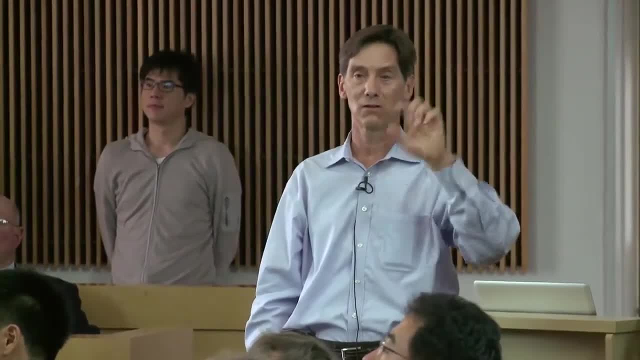 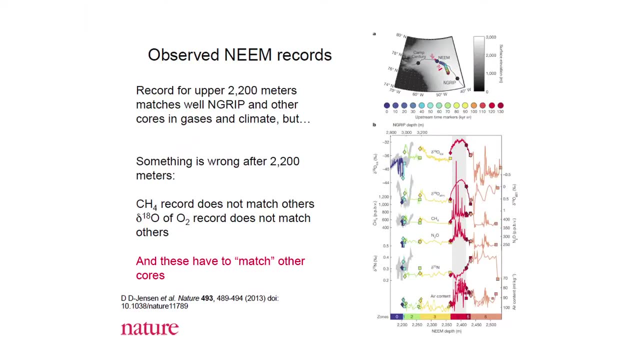 particularly for oxygen. you know that the del-O-18 that you measure in Antarctica has got to be the same as the del-O-18 of O-2 that you measure in Greenland. So this is a very important measurement for us. Methane we also measure. 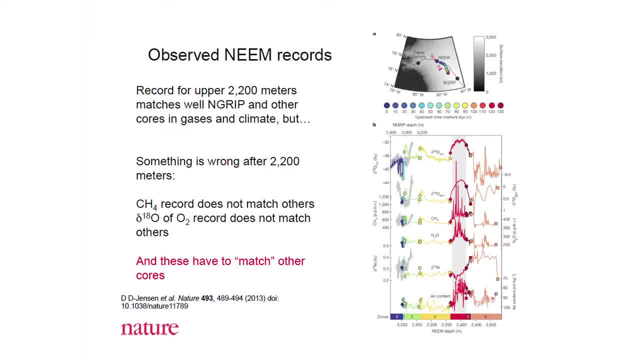 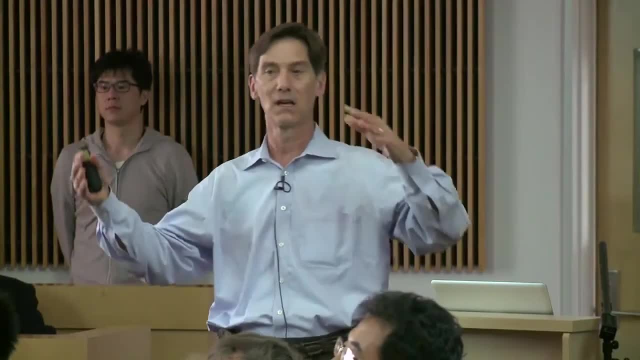 Methane is obviously a very important greenhouse gas, But it's also one of those gases that, while there is an inter-hemispheric gradient to methane, it's also got to behave basically the same between all ice cores, And so methane is something that we use to synchronize ice cores, that we use to put ice cores together. 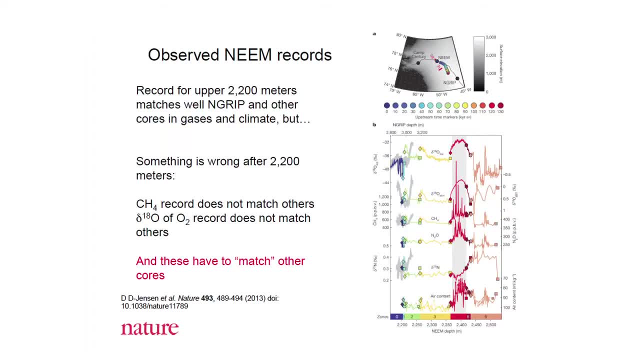 So we measure that, and that's measured in real time. Nitrous oxide is the next measurement you see here, And then there's a couple others at the bottom that I'm not going to get into very much, other than point out that we do measure air content, which is a rough proxy for how high the ice sheet is. 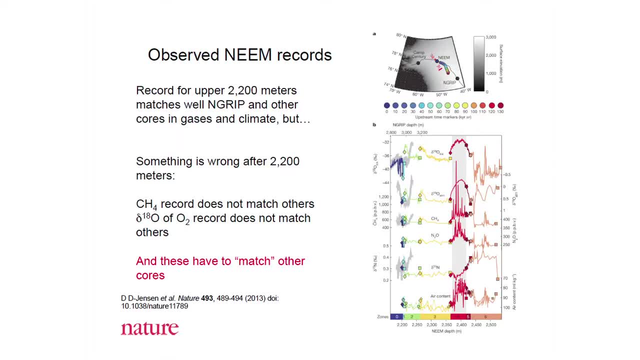 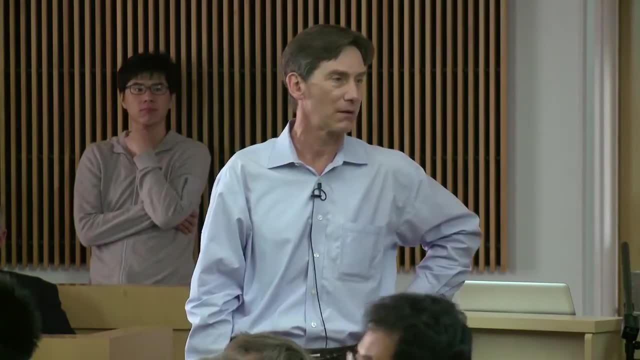 What we noticed immediately in the field was a couple of things. One was: methane had these huge spikes, And that's wrong, Because those spikes don't show up in other ice cores. They didn't show up in Antarctica, where we have ice cores from this time period. 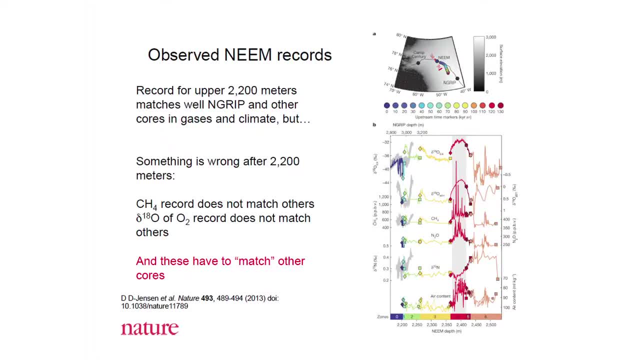 And so we knew that we had some problem here. Now the problems weren't huge, Because this, as I'll point out in a minute, is consistent with melting, And what this told us was that probably the emian was significantly warmer than it is today. 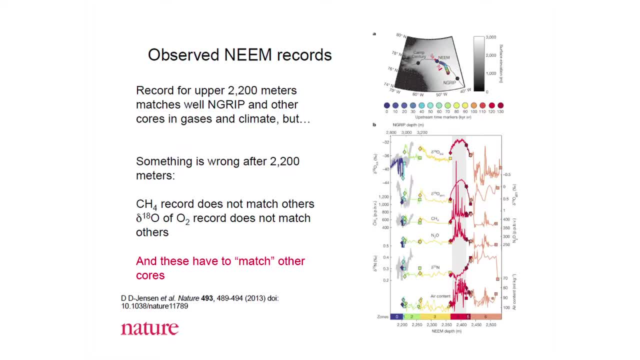 Because we don't see lots of melting today, But we do see lots of melting during the emian, So that's an indication that indeed it was much warmer. Nitrous oxide was basically telling us the same thing. What we also knew right away was that the del-018 of the atmosphere did not look right. 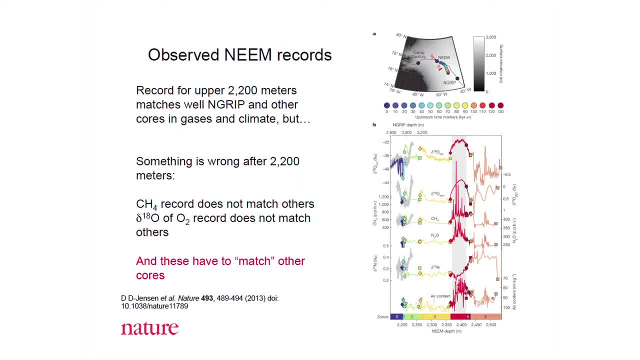 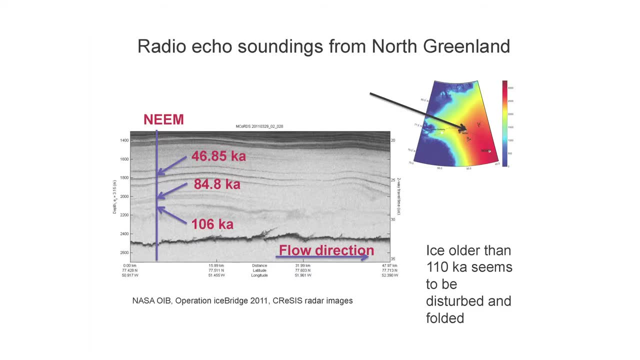 And so we knew that we had trouble with the ice core. There was something fundamentally wrong. Now we did a lot of work prior to drilling the ice core in looking at radar echo layers in the ice sheet. This is a slice from Neem. 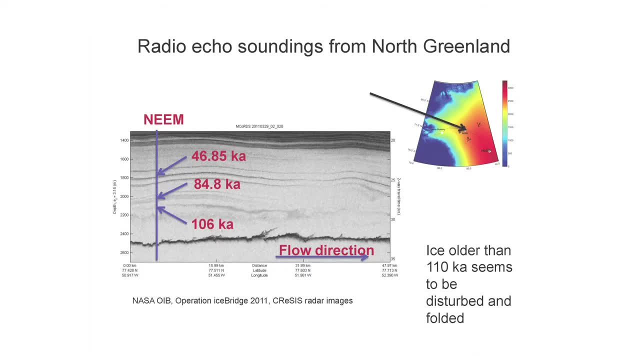 Here's the northwest corner of Greenland. This is the ice divide here And you see, with the flow direction coming here, that you see you can look at these radar echo layers and you can see that they're nice and flat And that's what we like to see when we go in and drill an ice core. 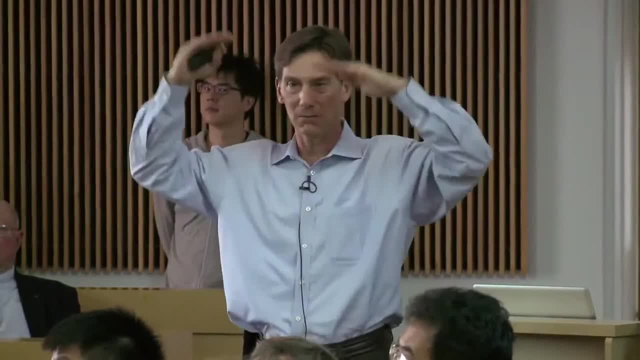 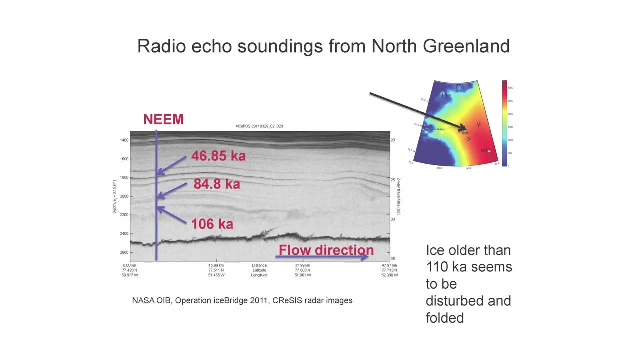 And the technology. at the time we started Neem, we could actually see that everything looked layered, It looked nice. I remember we had long arguments over whether or not there was any kind of turbulence at the bottom, any kind of problem at the bottom. 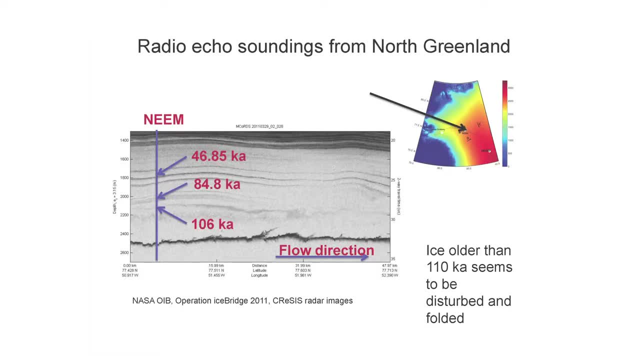 And at the time, with the best radar that we had, we couldn't see any problems, And so we thought we were in pretty good shape, or we thought we were in as good a shape as we were going to be. This is a later picture from Prasad Goganini's group. This is a picture on the north side of the ice divide, And here we have the. These are layers which are quite traceable from one ice core to another. For example, we can trace this from North Grip, where the thing is dated, and we know exactly where we are. Here you can see: at 84,000 you can see some really interesting folds and dips in the ice flow direction. This case is going in this way At 100 and something thousand years ago. we know that this is roughly the 109,000 threshold. 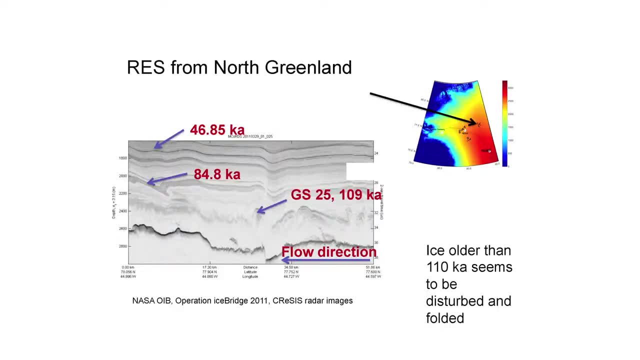 and you can see all sorts of bumps and wiggles in here. So, as technology has improved, we're now able to see: yes, there's problems in this area If you go a little bit to the south of the Neem area. 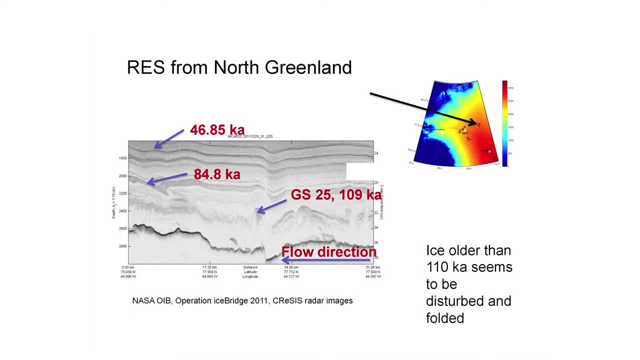 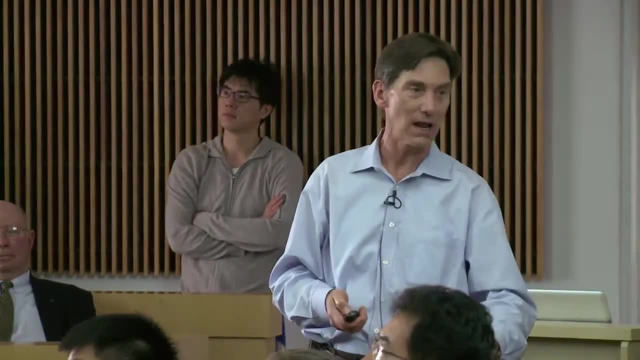 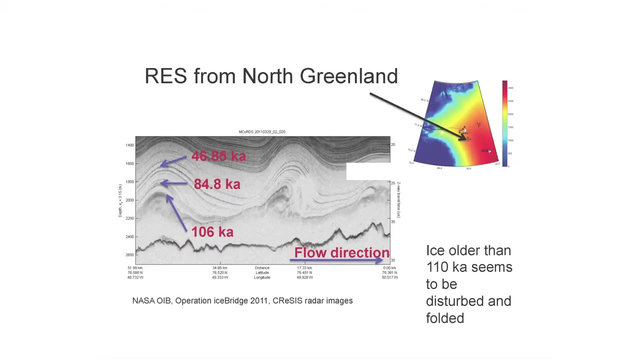 you can see even really fantastic features in here. This, by the way, is the reason why I'm now writing the proposal for the next big ice core, And until we actually map all these radar echo layers in the ice sheet, we're not going to go back and try to drill a deep ice core to get the Eemian. 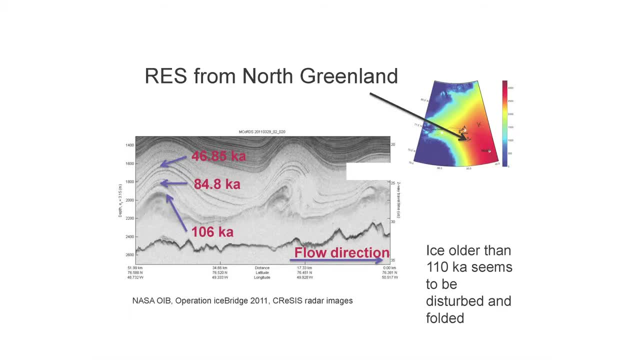 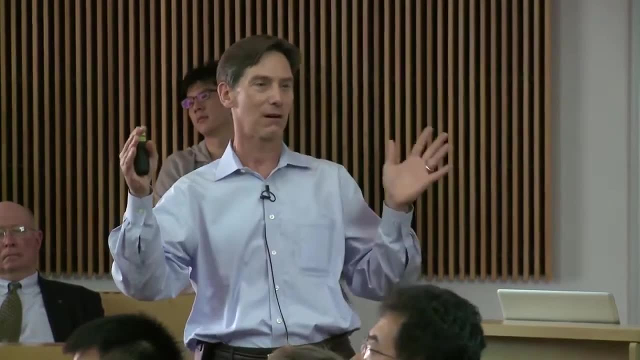 because obviously we need to know exactly what's going on, and figuring out all this interesting folding in here is something that we're going to need to deal with. So, basically a long story short. what we discovered was that this record I showed you before- 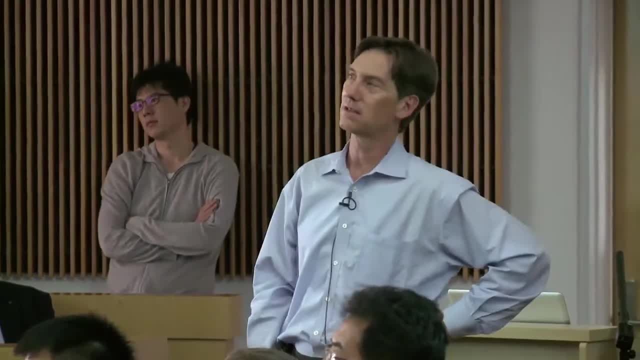 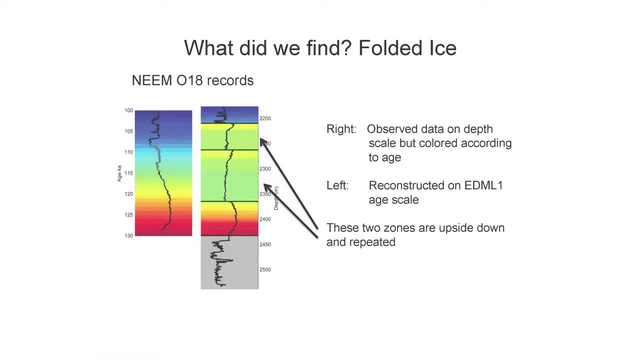 and the color coding is still the same- had a couple of pieces that were upside down and repeated, So the ice had folded over and I'll show you a little movie of what we thought happened. but basically the ice had folded over and we ended up drilling through it more than once. 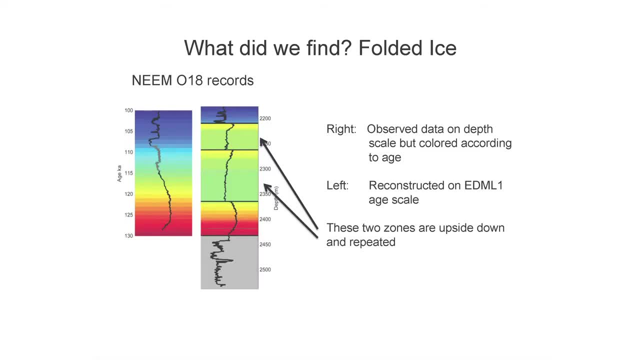 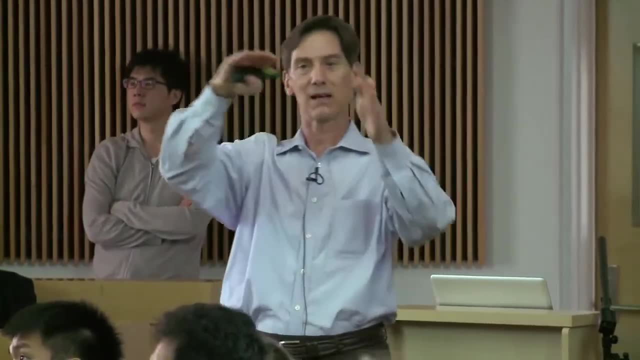 and having a piece that was upside down. Now, how do you know that? One of the challenges is: you've got this scrambled record and those of you who are geologists and you know, you go out in the field and you look at rocks. 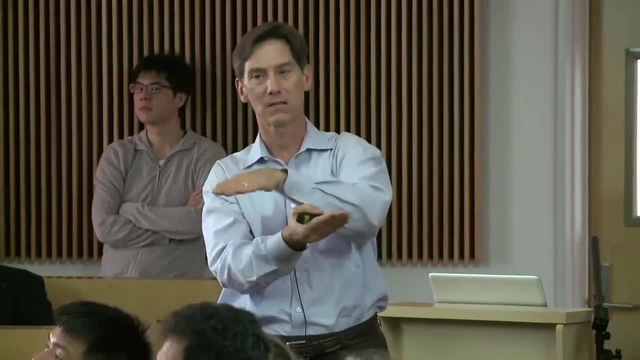 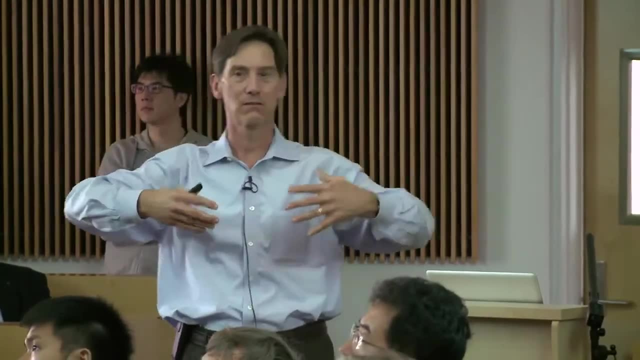 Do you guys do that at all around here? Maybe not. Anyway, they do that right. Geologists go out and do that And they look at rocks and they see all the folding and stuff and they try to put stuff back together and try to re-. 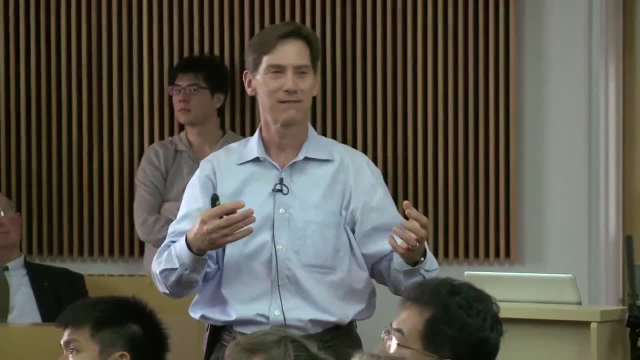 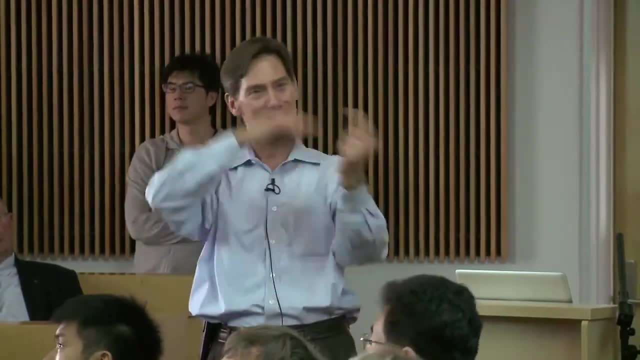 get the deck of cards, if you will, stacked back up the way that they would have otherwise, And so we spent quite a bit of time arguing about it. I remember Dorda was in my office for a couple of days and we plotted things differently. 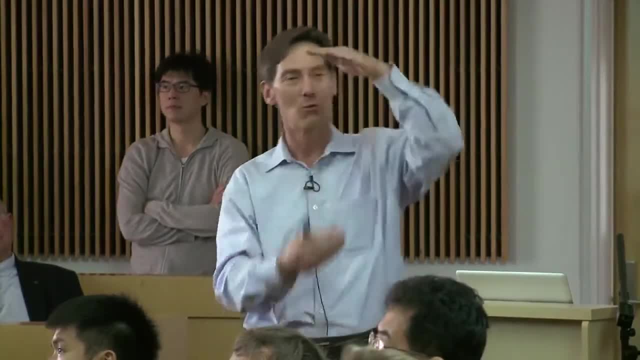 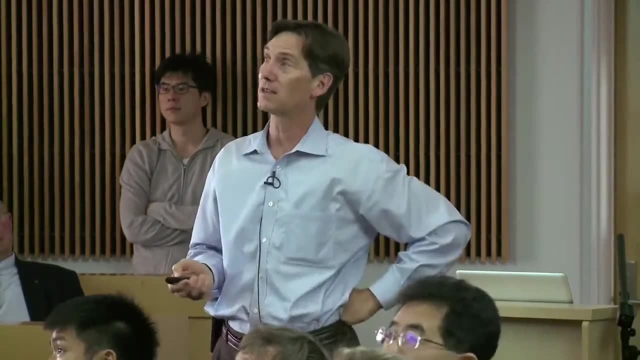 We messed around with things. Basically, what you want to do in order to make this, put it back together is you want to plot things that you know have to be correct, And it's sort of like a phase diagram, And then you take what you've got and see how it lays on there. 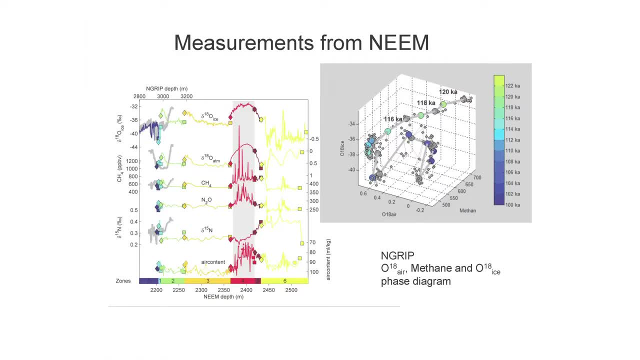 and find the most logical way in which the pieces go back together. So, fortunately, what we had from North Grip was we had the del-O-18 of air- We talked about methane- and the del-O-18 of ice And we were able- we are able- to plot in a three-dimensional space. 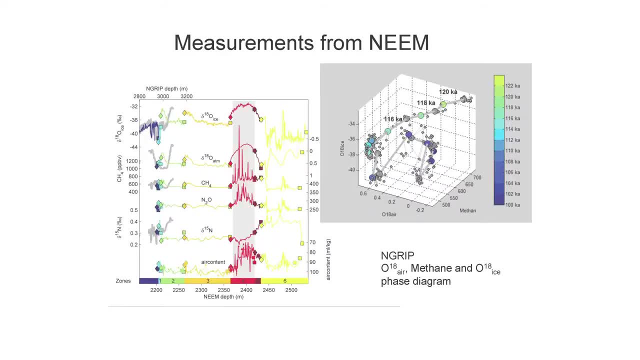 the evolution of what the North Grip ice core looked like. So in this we knew. we know that North Grip was not folded at the bottom And the reason for that is a little more complicated story. But basically it's melting at the bottom of the North Grip ice core. 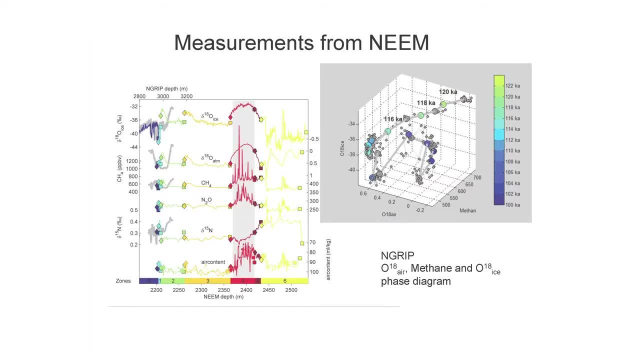 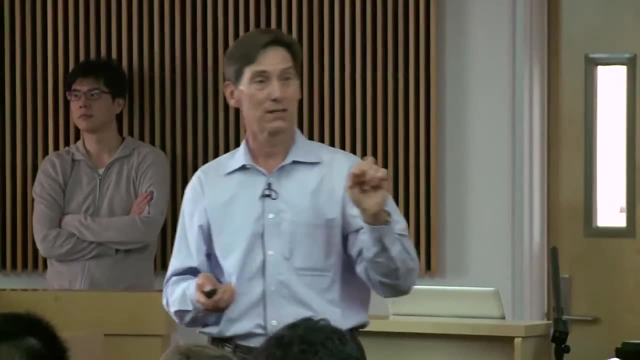 And so the ice never gets a chance to fold there, because it never sticks at the bottom. It just keeps melting off the bottom, And so we knew that we had to match this particular phase diagram, And this is what we got when we added the neem. 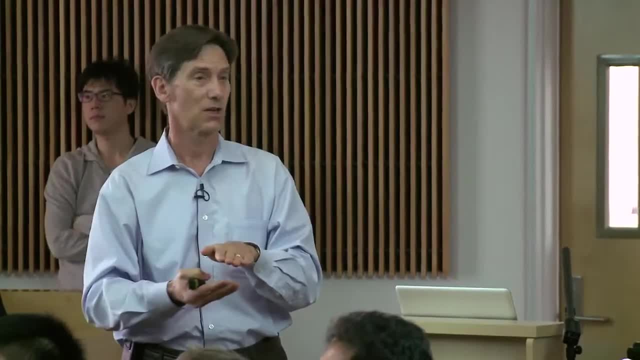 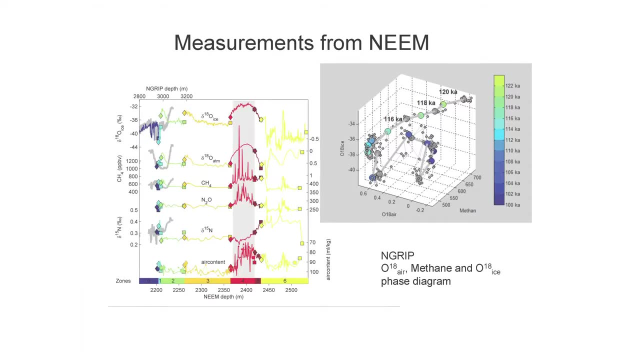 So now you see, by the way, the methane scale has been expanded, which is why that three-dimensional diagram I showed you before has now been collapsed And you see, almost all the information we saw before has now collapsed into the lower end of the methane scale. 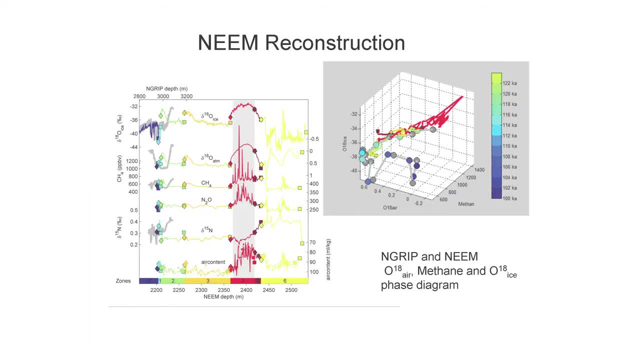 Because we have these high methane peaks, for example. we know that this can't be right And you can see over here where those high methane peaks are. But everything else- and I'll now show you one slice through this- everything else made sense. If we invert. And we can also tell that Greenland did not contribute more than roughly two meters to the sea level rise in the last interglacial period. So we can tell from the climate, we can tell from the height of the ice sheet that indeed this locality Disney. Who's behind climate change? I'm not going to go there. You ponder that There's some interesting parts of the United States under 20 to 25 meters of sea level rise. This is one of them. This is the. so the same idea of one degree C per year, change for five years and then a plateau, But the plateau might have been different In deuterium excess, which is a combination of deuterium and O-18, and I won't go into the details. but it's a very rapidly changing parameter and we think it's tied back to the ocean condition. You see here that the deuterium excess shift occurs about one to three years at all of these sites. This is the end of the Younger Dryas. It cruises along and drops. This is the end of the Younger Dryas It drops. This is the North Grip and Neem. I won't go into any kind of detail here. I do want to show you that this is the bowling warming. in deuterium excess space. So these are two isotopes combined- cruises along drops and you actually get features in here that are very similar from the location. So we're not looking again. this is not noise, We're looking at signal in here. And this is a shift in one to two years of something fundamental in the climate system. All right, So I told you I would give you no answers, but I'll give you some speculation. All right, I had a postdoc, Jacqueline Flugiger. who worked with me and we tried all sorts of models. We tried simple models, We tried complex models. We tried to get the model to make a change happen of the magnitude we were looking at in the time period we were looking at. So, in other words, I wanted to see a change of 10 degrees Celsius and I wanted to see it happen in anywhere from 50 years to one year, And we couldn't get a model to do it. And it's still true today: We cannot get. we cannot get these kind of abrupt changes to occur in our most sophisticated general circulation model. Now, I don't know why that's the case, but this remains a challenge. It remains a challenge for the models. It remains a challenge for the paleo community. to try to understand what all this stuff actually means. So there are many striking features. They're fast, They're huge. Going from Mobile to Minneapolis climate-wise is a very big deal- And I haven't made a big point of this- but the stability of these states. is remarkable. So keep in mind that you had a younger, dry-ass, cold period, which was 1,000 years long, that had a certain level of snowfall, had a certain level of temperature, certain level of dustiness, all this stuff. And then, in a matter of a lifetime or less, you went to a totally different state that stayed that way for the next 12,000 years. So what keeps these things stable in their states? How do they? how do, and this is where the ocean mechanism. has come in very strongly over time. People have argued that this has to do with the turnover of the North Atlantic deepwater, the Atlantic meridional overturning circulation. But what we have tried to do over and over again in models is put that into the model. run the thing and see what happened and we can't get the result that we want. So I think there's time- we or not time, but I've been thinking quite a bit recently about other mechanisms, and particularly atmospheric mechanisms, So I'm not going to give you any answers. I'm just going to give you today's current speculation, because I- why not? I think that there probably was a split jet stream at the time, and I think that perhaps that had impact on ocean circulation in ways that right now the models don't capture. 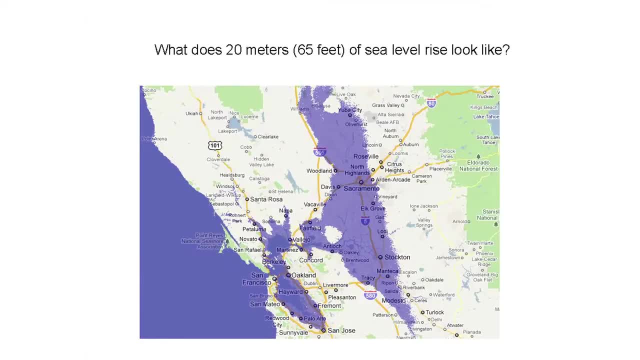 So, in other words, could you have a situation in which you had- we think there was- a very strong jet coming over the pole at the time, and that's because of dust that we see in the ice core and we can actually fingerprint that dust to China? 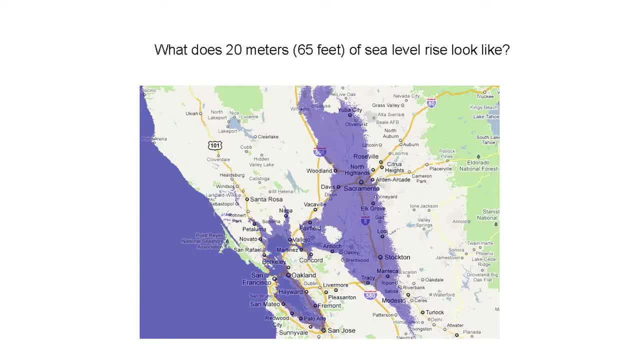 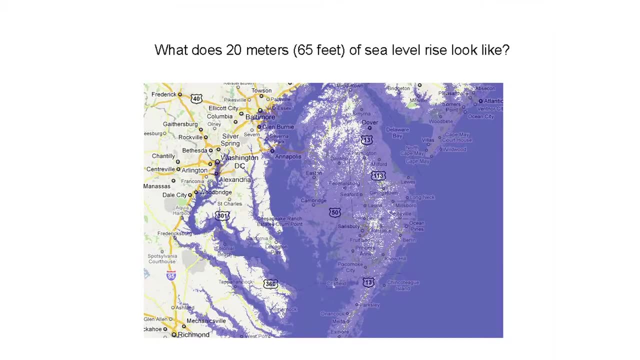 and we're pretty sure that there was a pretty strong piece of the jet stream coming over the pole. Could that have fundamentally changed the way that the North Atlantic was getting fueled with icebergs or the way it was getting fueled with fresh water, or you know something going on there? 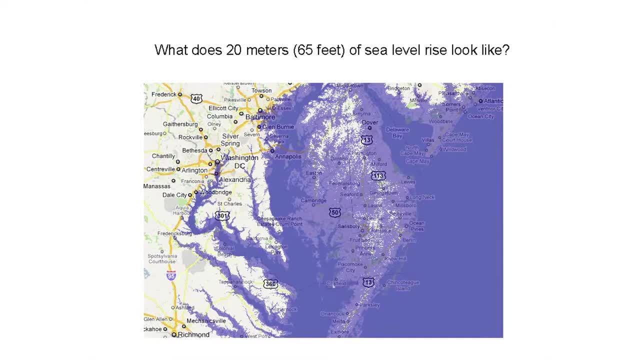 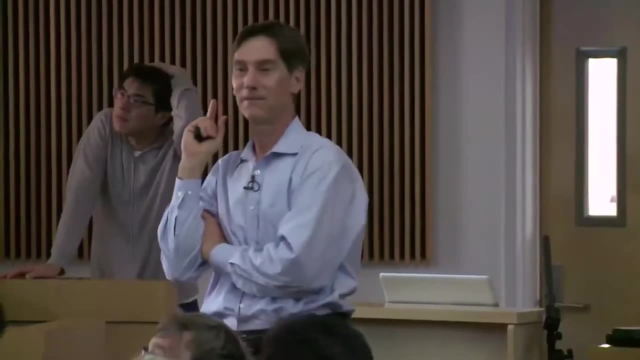 that then indeed impacted meridional overturning circulation of the North Atlantic deep water. So I don't know the answer to that. I'm just going to throw that out as a possible idea. I will point out Bill said I was a data guy. 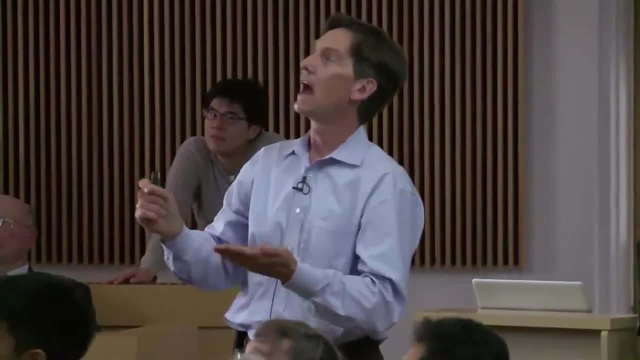 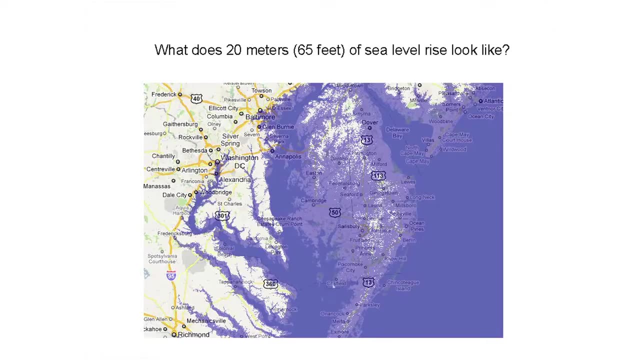 I am a data guy. I also. actually, one of my most recent publications was a publication on modeling the Pliocene. So I pointed out before that the Pliocene is a very warm time period. Models can't get it that warm either. 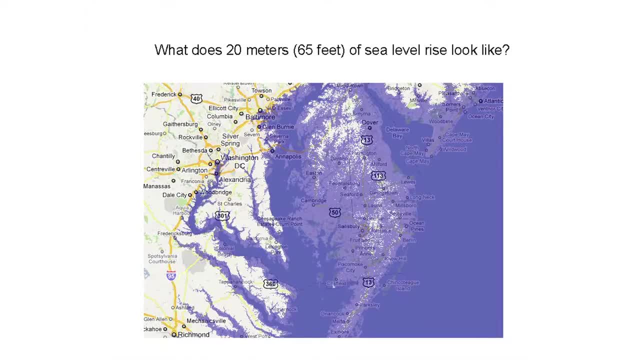 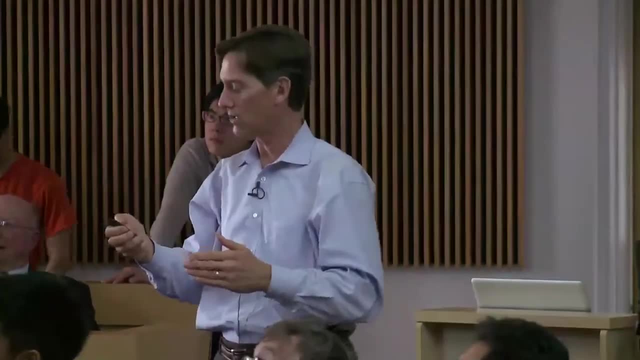 This is another point where we're struggling with the models to figure out. how do you make the Pliocene as warm as it was And, as it turns out, there may actually be a loop in here. One of the things that we found was: 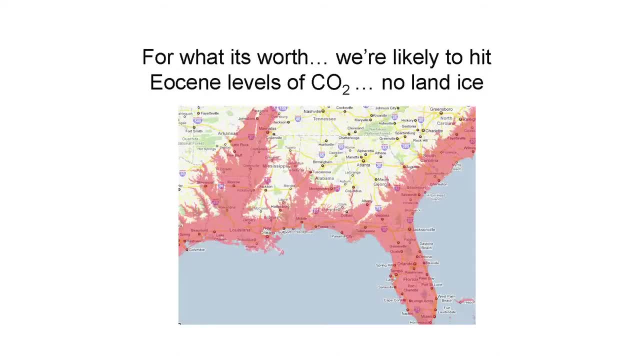 if you took all the sea ice out of the Arctic, you could make the Pliocene warm. Big question is: how do you take all the sea ice out of the Arctic? And we don't know the answer to that question, but I'm beginning to think there may be something. 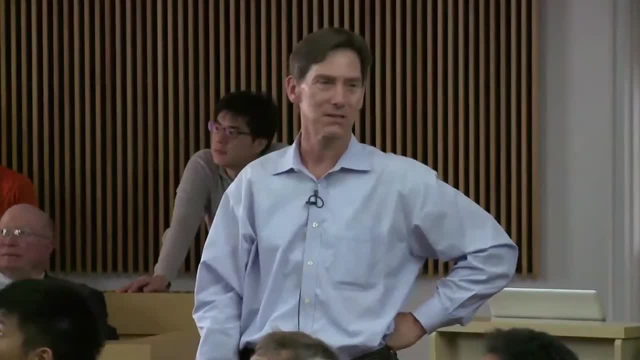 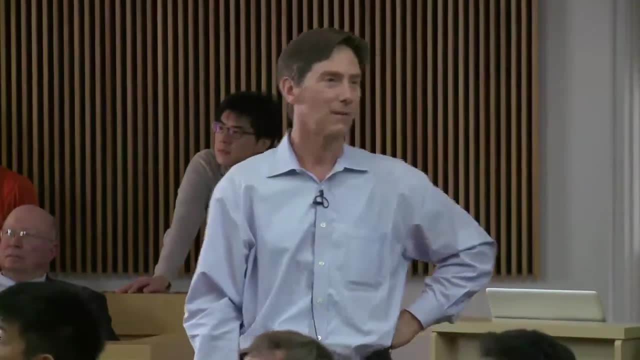 about the way the atmosphere circulates and the way the ocean circulates, that these two things might be tied together. So I will wrap this up. I'm not going to get in the low light. I'll wrap this up with a slide that these days. 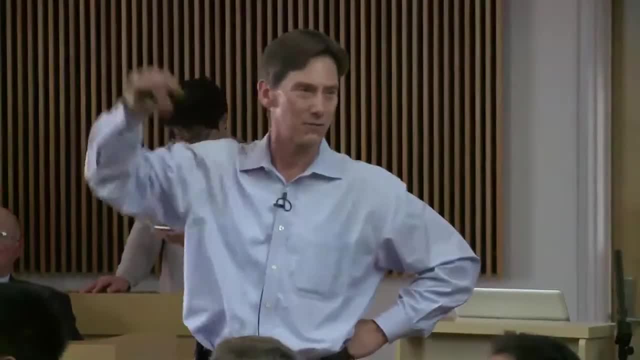 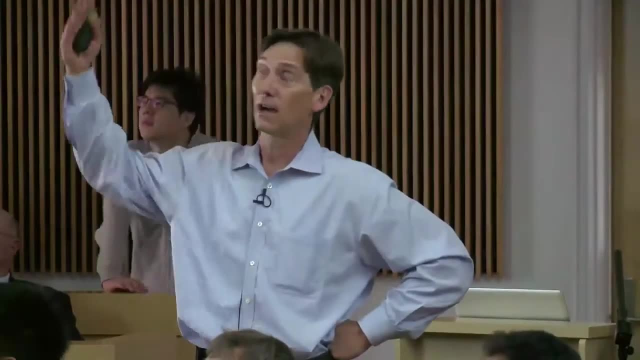 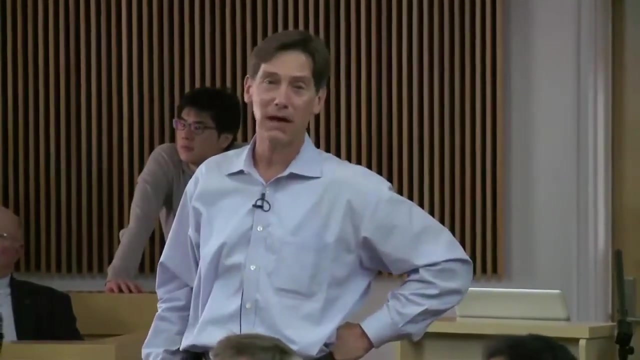 even in scientific talks. I come back to this slide Now. this has very little to do with science. It has a lot to do with ethics. So if you're expecting all science, you can turn off right now and I will rant for a while. 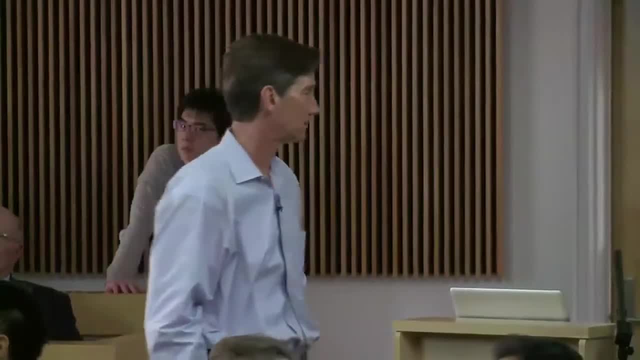 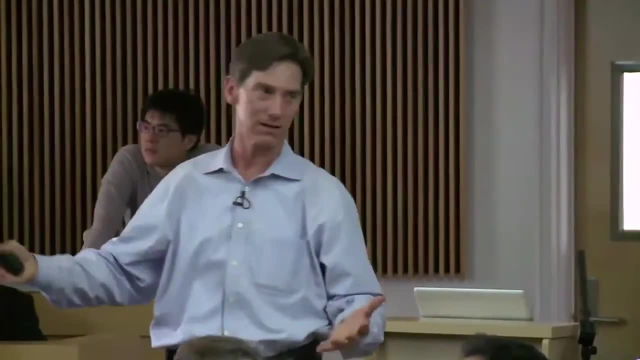 and then you can say, okay, turn it back on. We hear all sorts of stories about changing climate. We hear a lot of doom and gloom, And what I've shown you in this talk today is, indeed, we've got worries. We've got worries in Antarctica in terms of sea level. 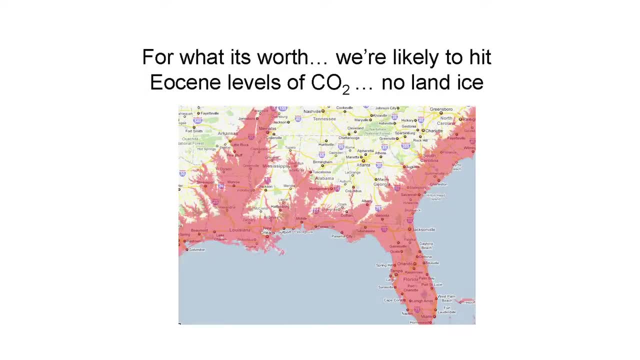 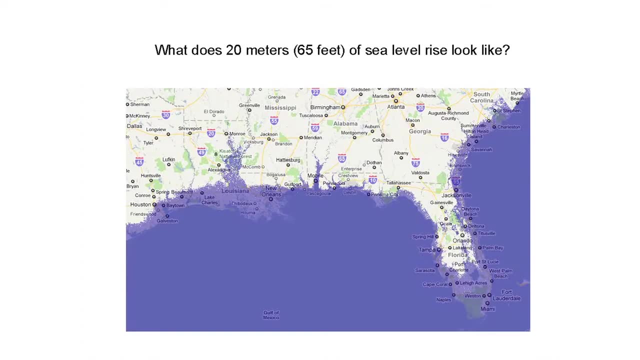 We've got worries in terms of the climate system being far more unstable and angry, if you will- than we give it credit for today. that we include in our models, that we include in the IPCC projections, we include in all of these things. 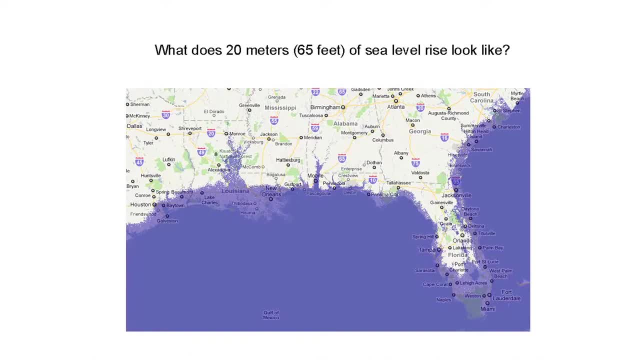 We've got an angry climate system out there, and that's not a good thing. Now you can get depressed about that, or you can take a step back and go. what's the good news Now, as it turns out, there's good news. 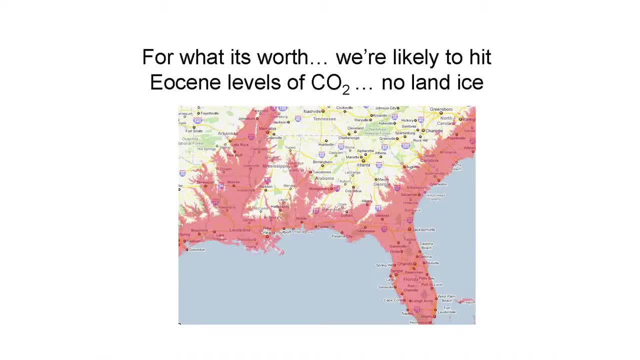 And I'm going to tell you the good news: In order for us to move forward, to move forward on the planet, we've got to figure out how to live sustainably on the planet. And in order for us to live sustainably on the planet, 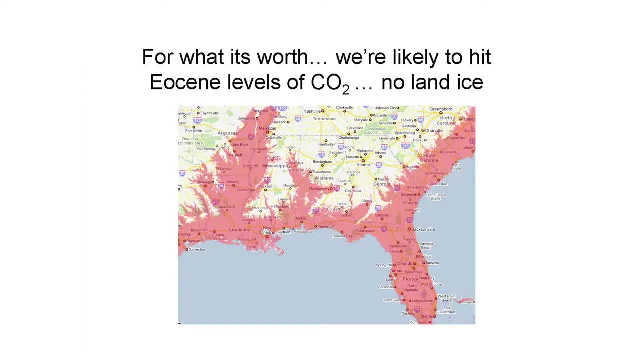 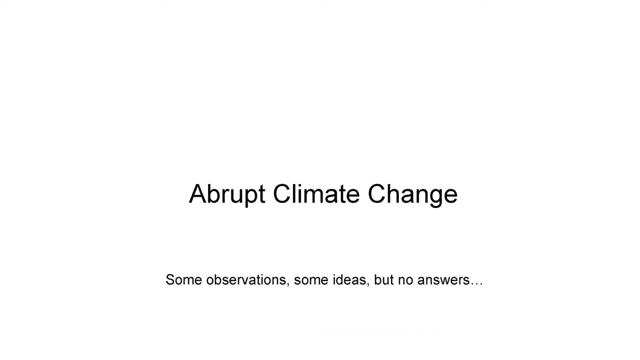 we have to overcome certain hurdles. A big hurdle is the hurdle of the fact that we live on a water planet. When you live on a water planet, climate is always delayed. It takes a while to warm the ocean up. It takes about a generation, as a matter of fact. 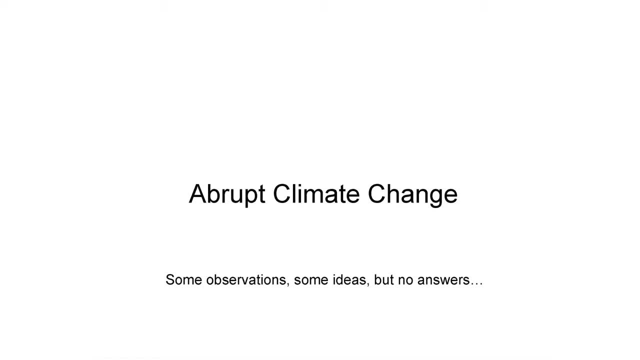 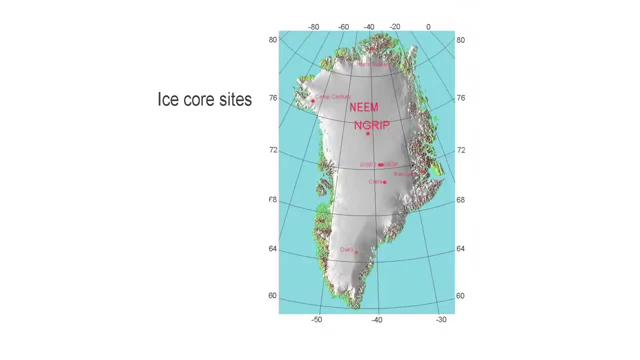 to warm the ocean up. So while we have 400 parts per million CO2 in the atmosphere today, we don't have a 400 ppm climate today, And we don't because we don't have. It's going to take a while for the ocean to warm up. 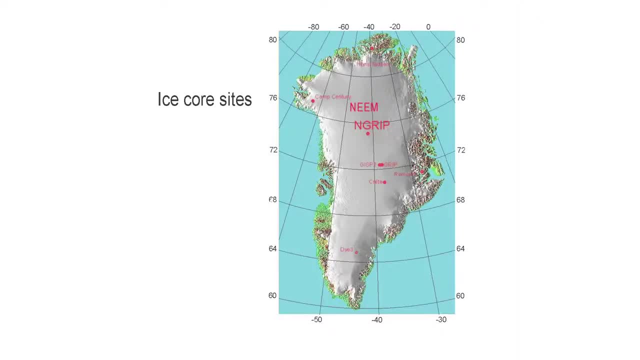 It's also going to take a while for the ice sheets to melt. There's all these lags in the system, And one of the keys to dealing with that problem is figuring out how are we going to get one generation to actually value the next generation. 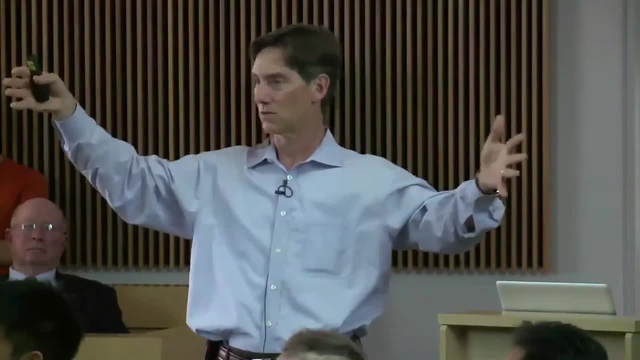 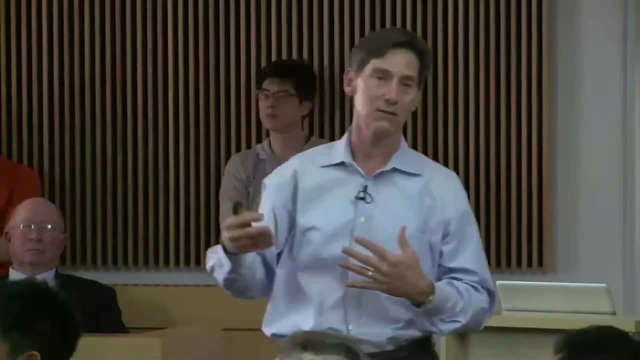 The intergenerational ethics here are huge. So what my generation is doing is burning all the available oil and coal I can get my hands on and natural gas, creating CO2 at high levels and then handing it off to my kids, While, by the way, I say, 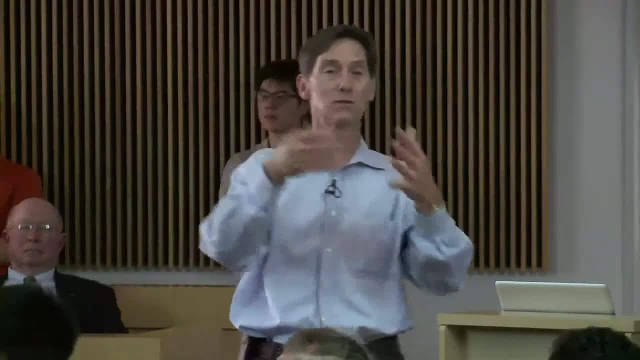 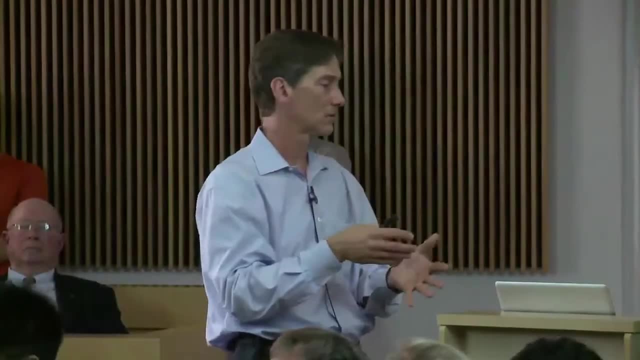 and this is true, I love my kids. I'll embrace my kids, I'll say I love my kids, But do I show that? Not really. If I really love my kids, would I be doing this to them? And my answer, honestly, is no, I wouldn't. 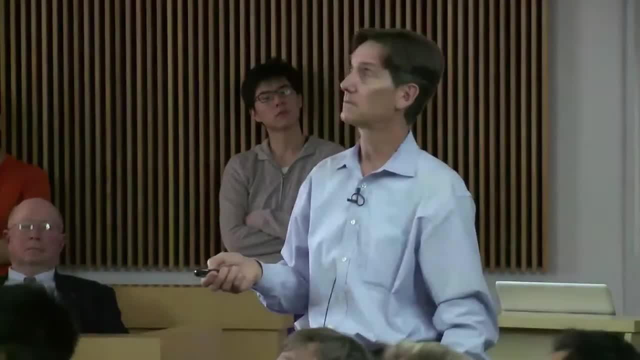 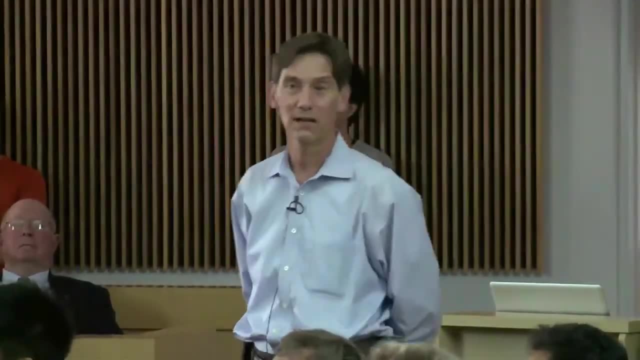 That there has to be a better valuation of one generation to the next. That's one thing we have to overcome. The second thing we have to overcome is we have to deal with population. Now, this talk had nothing to do with population, but in the end, population is critical. 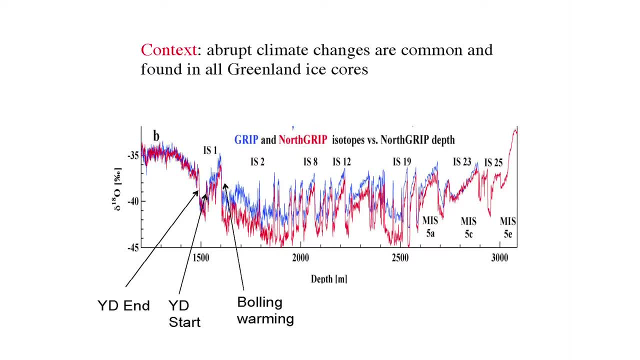 to dealing with our future on the planet and our intersection, if you will, with the climate system. What is the key to population? Demographers will tell us over and over again: it's the equality of the sexes. We live on a planet in which men run the show. 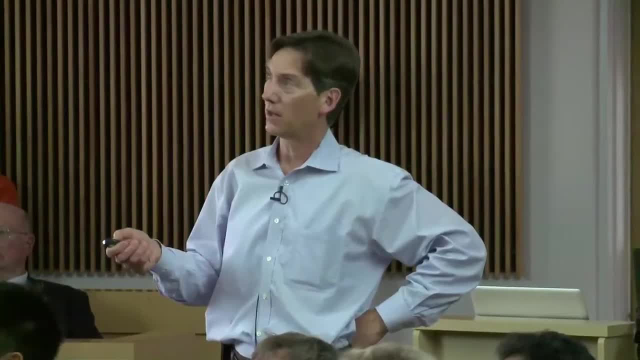 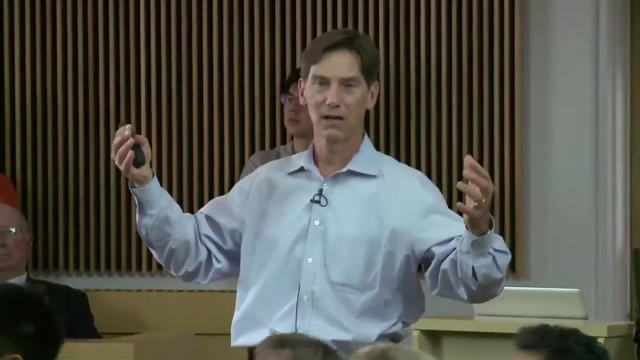 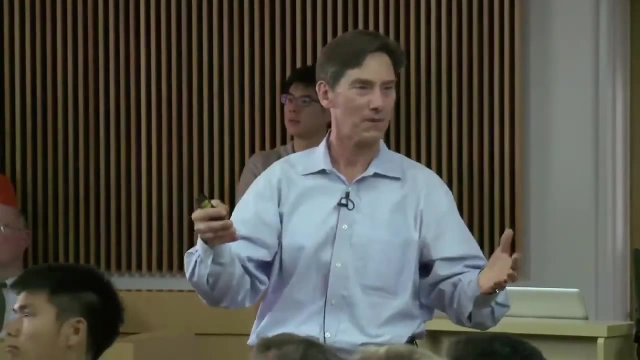 And in many parts of the world men are valued only for the number of babies they have. As long as that continues, you will not be able to deal with population on this planet. And lest you think we are doing so well here in this wonderful industrialized country of ours, 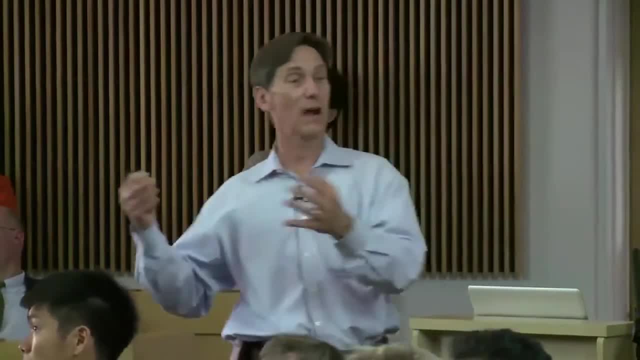 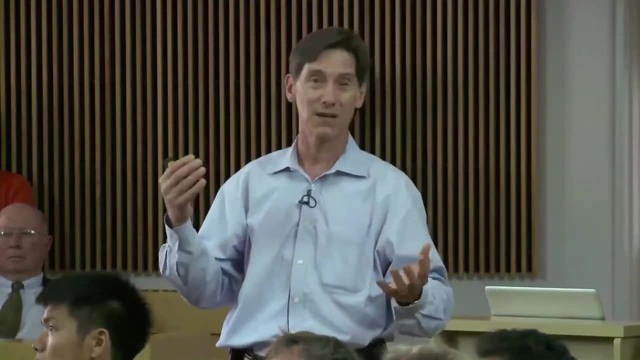 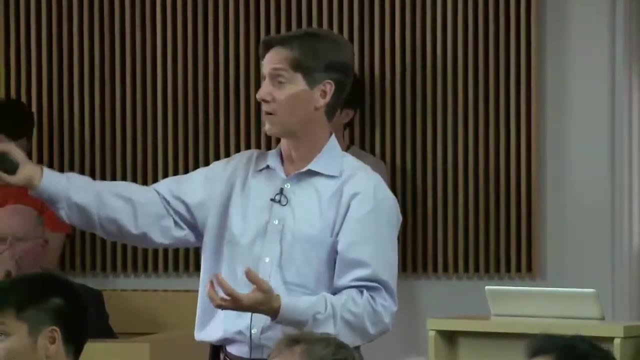 who was the first female president of the United States, Clio, When did women get the right to vote? This is a world which has got things turned around in terms of its relationships, the relationship between men and women, And until that relationship becomes more of equality. 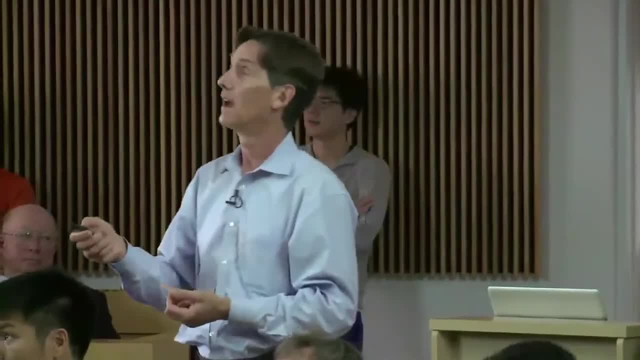 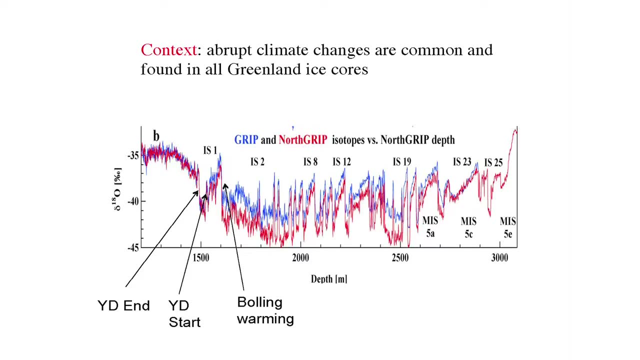 you will not be able to deal with population. Third piece of the puzzle is: as long as you have 2 billion people on the planet who are not participating in the economic wonderness, wonderfulness of what we have today- the middle class and beyond. 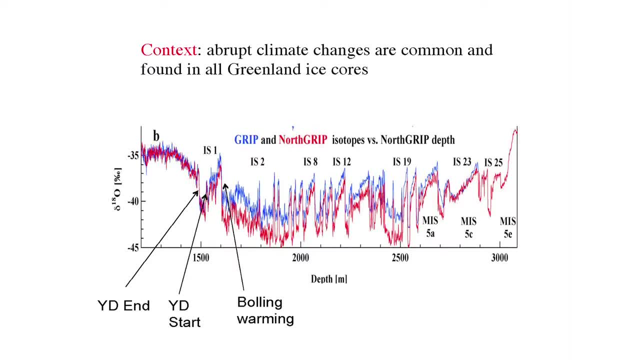 and indeed there are 2 billion people who daily either starve or don't get enough calories. they don't care about the environment and they don't give a rat's patootie about climate. they care about where they are going to get their next meal. 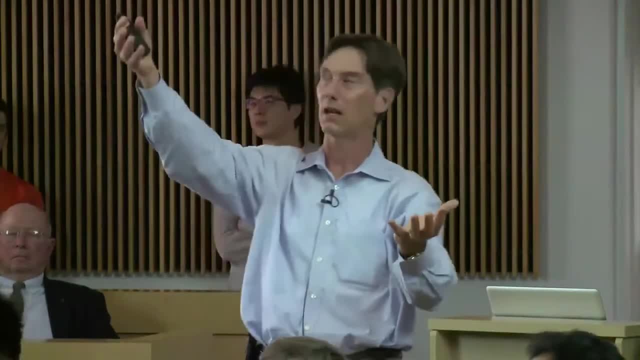 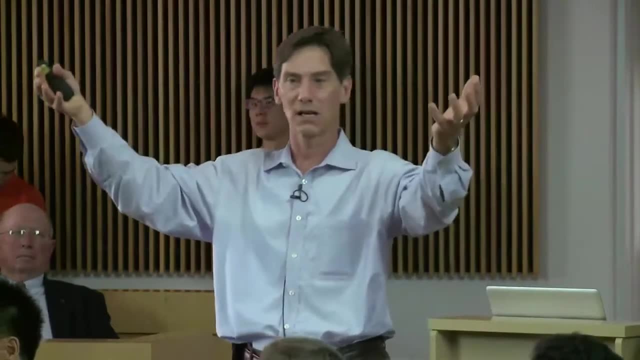 and they are going to care about putting shelter over their babies' heads and they are going to care about feeding their kids. So until you have better wealth equity on the planet, you are never going to get to a situation where you can control and deal with the big issues. 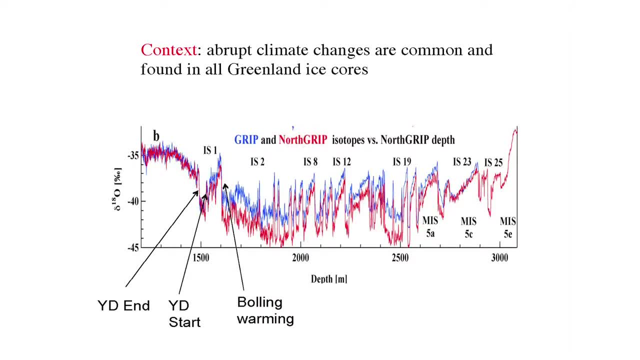 of our, as a collective species, valuing the planet on which we live Now. I think it's good news that, in order for us to live more sustainably on this planet, we have to actually value our kids, indeed, as well as in words. 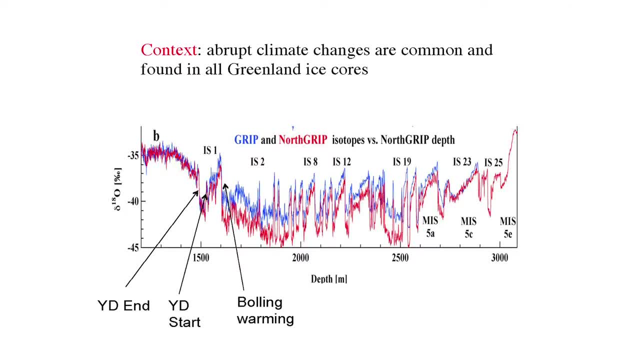 that men have to treat women better and share the power and the wealth on the planet, and that the rich have to actually treat the poor a little bit better. If we can get those 3 things under our belt, we can get closer to sustainability. 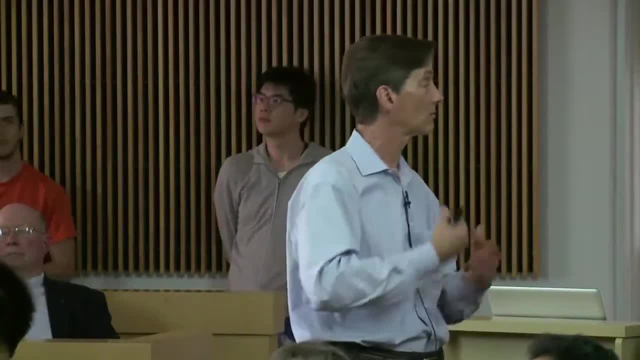 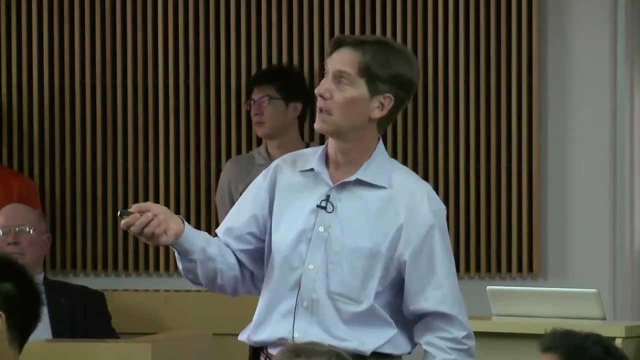 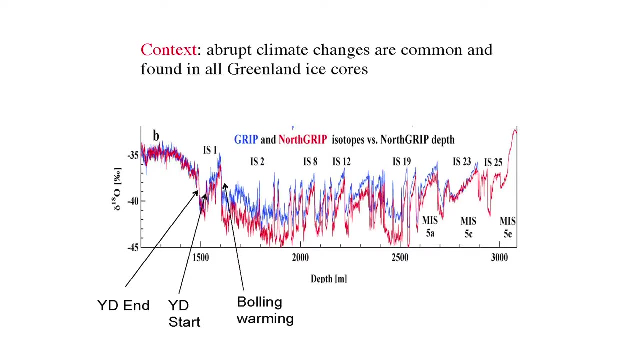 and we can get closer to sustainability. Thank you for listening. I appreciate very much the time that you've given me today and I'd be happy to answer any questions. I don't know where to look. Fortunately, I said nothing controversial in the last. 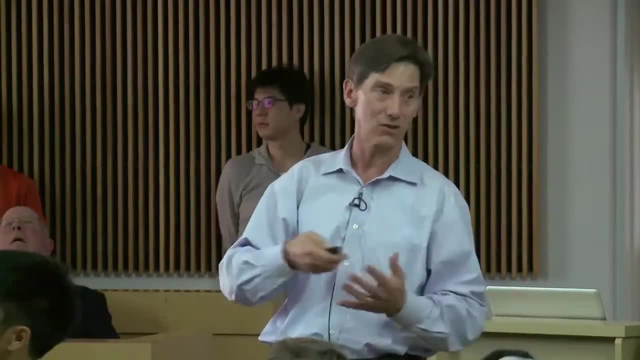 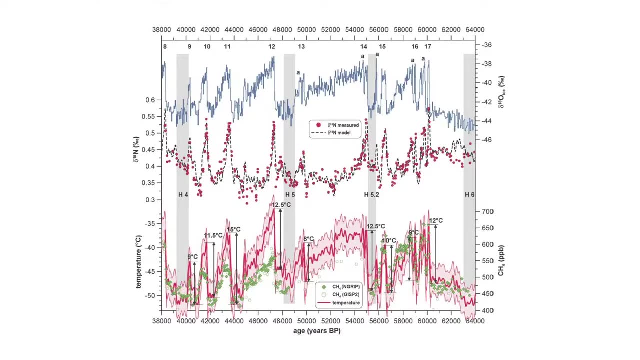 Yeah Marat, Yeah Marat. So I've been talking a lot about climate change and the magnitude of the climate change and the timing Data is from Greenland. Are you talking about green climate, profit climate, global climate? How do you go from one to the other? 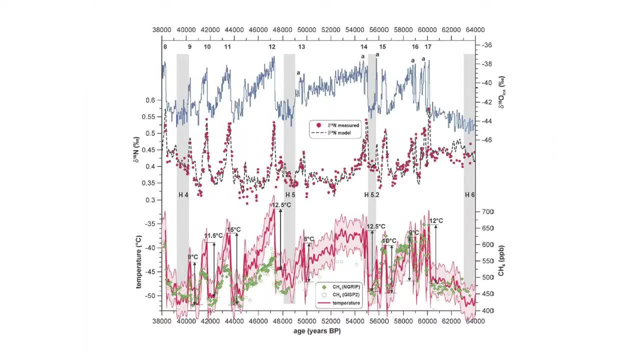 There are. I didn't You know in the time allotted there's no time to go and look at all the records around the world, but there are, particularly in the Northern Hemisphere and in the tropics, quite a few records that show. 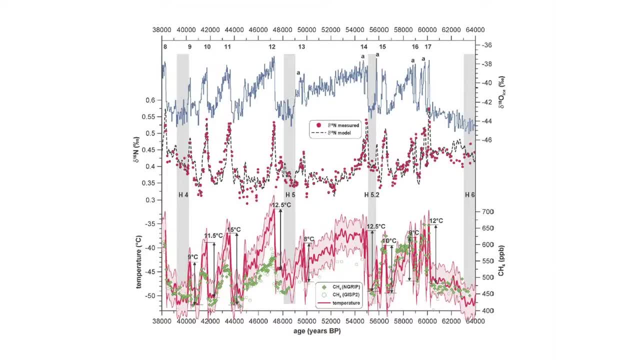 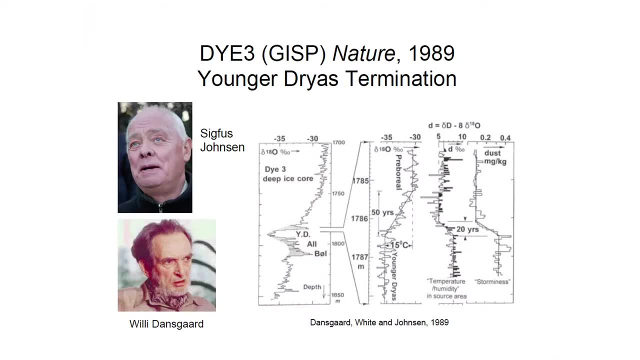 you know cave records in China, ocean sediment records, the Cariaco Basin, other places that show that abrupt climate change is not just a Greenland phenomenon. Were it just a Greenland phenomenon, we'd be talking about something different. It doesn't translate as well to Antarctica, as you know. 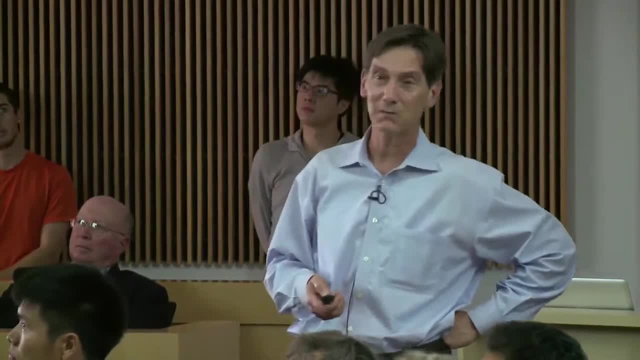 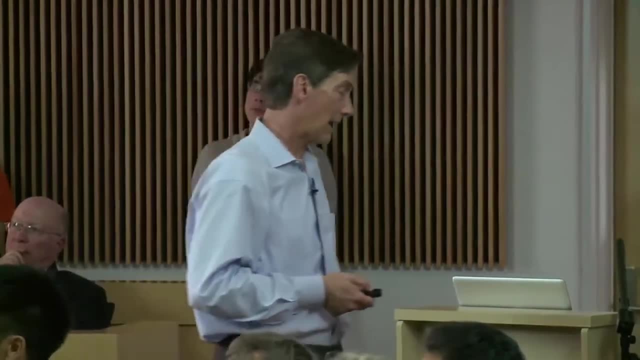 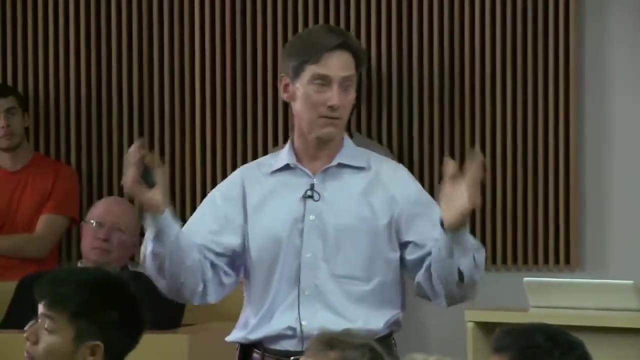 and that's one of the features of abrupt climate change that we'd like to understand more about. Yeah, I have a related question. When you talk about the temperature swing, is that the mean annual or is it the mean of the summer? I don't know. 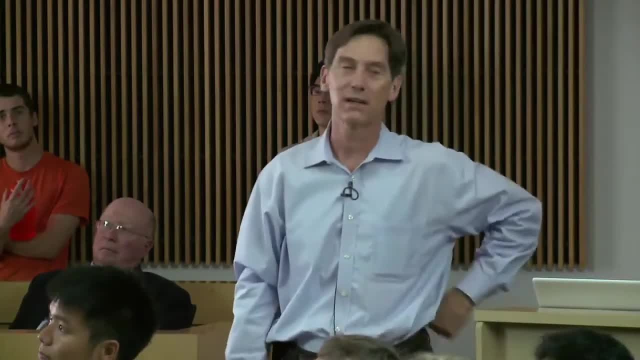 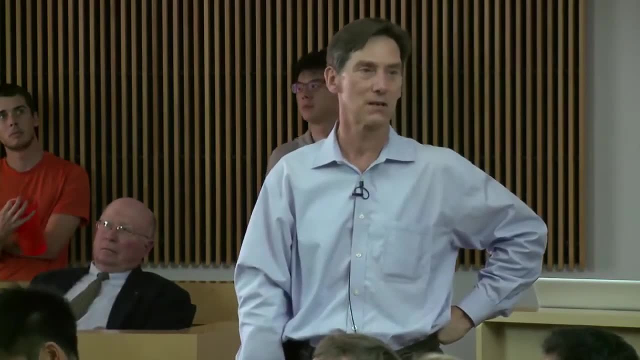 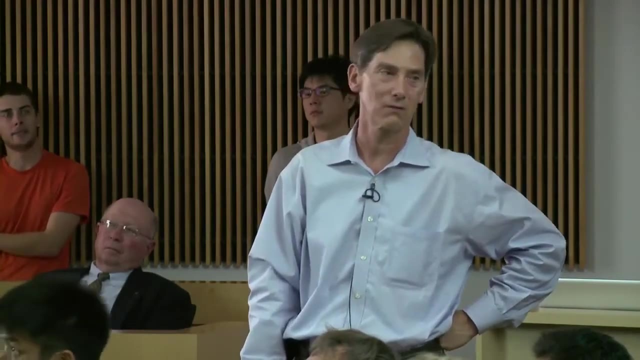 And I'm not sure we will know. More than likely it is seasonally biased, particularly if you think about when it gets really cold, you lose some of that winter precipitation, And so what you're looking at is going to have some seasonal bias. 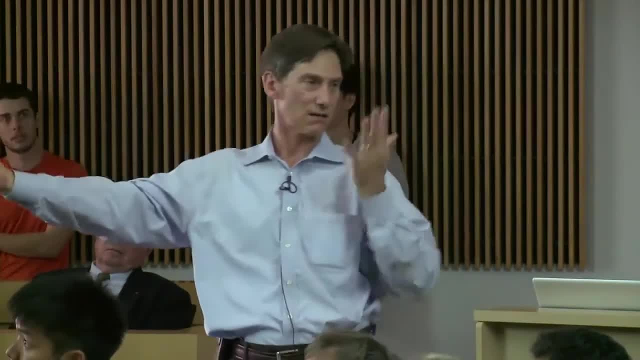 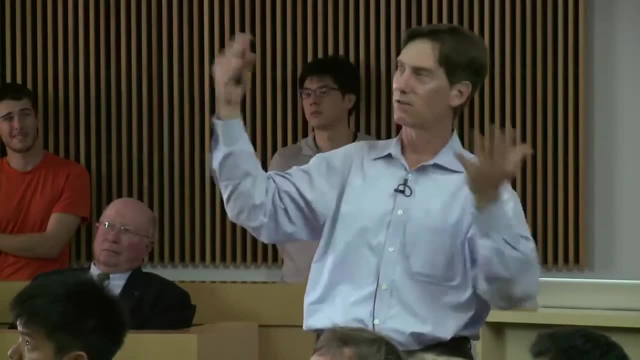 The longer answer to your question is that, while the temperature is calibrated by a method that I really trust, which is the nitrogen-15 of N2, the isotopes are being used to give you the year-by-year changes And the year-by-year changes in the isotope. could well have seasonal imprints all over them. If you could imagine a year in which you didn't have a winter, you'd have an isotopic composition that was pure summer. Okay, As a possibility. So the answer to your question is way more complex. But you do need to be careful about that. No, Is there like beer waiting or something like that? Yeah, Yeah, Yeah, You would just create a puddle at the surface and you get a little extra methane in there. Yeah, the it's not. you know, typically we go. we try to go places, Bill, where you don't get melting, to get gas records because, yeah, What we found in this far northern part of Greenland is that more than likely we're going to have trouble with that. So even if we got a perfect record of the Eemian, it will have probably have melting in it because this is one of the coldest places we could go. So the Greenland ice sheet was quite different during the Eemian in that sense, in that you know, it was more like well, for example. the southern part of Greenland today melts frequently during the summertime, So the southern part of Greenland is probably a good analogy for what northern Greenland looked like at that time too. Yeah, So how fast can we go? So how fast can ocean currents change? So they have a lot to do with the climate. That's, you know. the core of my challenge here is: they can't you know, we don't know. but shutting down in one year, maybe that's possible, but I don't know. I mean, ocean currents have an inherent inertia And certainly in the models that we've looked at, where we basically, in order to get the North Atlantic deepwaters shut down, you put a whole bunch of fresh water out on the surface of the ocean. And that keeps the surface water from sinking to depth right. And when you do that, if you do that in one year you can get the system to shut off in one year. You can't get Greenland to cool off that fast. You can't get the whole climate system to then readjust. in a very short period of time. It's also artificial, right? I mean, here we are dumping a whole bunch of fresh water out there. In order to keep the system from reestablishing deepwater, I got to keep putting fresh water out there. So I got to find a hose with a very big tap somewhere and just keep pumping fresh water out there. It's one of the basic conundra conundra. It's one of the basic problems that we have in trying to interpret these abrupt climate changes. in terms of deepwater formation. Keeping that system shut down is a hard thing to do. Yeah, Yeah. along those same lines I know it used to be. we had to put in very unrealistic amounts of fresh water, Yeah, Yeah, No, no, we're able to put in. more realistic amounts of fresh water. That's why I think, for example, if you ponder the idea that if you've got a strong polar jet coming over- and I don't want to get too far into this because it's complete and utter speculation- but if you're constantly pumping ice down into the NADW formation areas- lots of ice coming down in there- it's possible that if you just keep that air circulation turned on, you can keep pumping fresh, fresh water via ice into that area. and keep that system shut off as long as the winds happen, Which is why I went to the Pliocene for a minute there, because, if you think about it, if there was no sea ice during the Pliocene, you couldn't have that mechanism. And so maybe there's some hidden ocean mechanisms in here that we don't know about. Yeah, So if the ocean currents and the jet stream changes, which kind of seemed like they would be a gradual change over time, what's the next thing in the Earth's system? that you would jump to to explain the rapid signature change that could happen so quickly. that wasn't the jet stream, It wasn't So, it wasn't the atmosphere of the ocean. You're not leaving me a whole lot of planet to work with. I mean, it just seems like those are kind of gradual changes that would happen. Actually, I would argue. I think the ocean has a certain gradualness built into it because of the just inertia of water circulation. I think the atmosphere is capable of some boom changes. So I actually think the atmosphere is where we should be looking. That what I don't the problem. so here's sort of the conundrum here. The ocean has lots of inertia, but it seems to be capable of sitting in one state or another state. So the state issue seems to be answerable by the ocean. The speed issue can be answered by the atmosphere, but the atmosphere doesn't seem to be the kind of system that wants to stay in one state. So, in other words, if we had a polar jet stream, 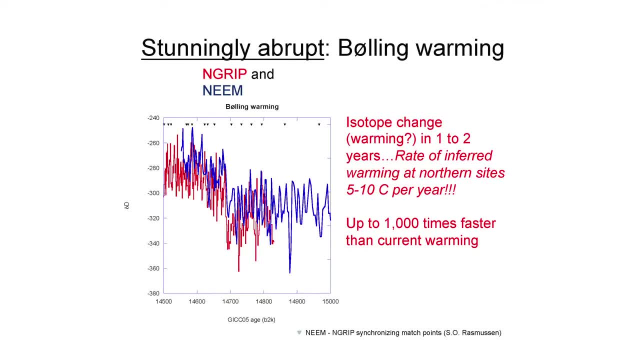 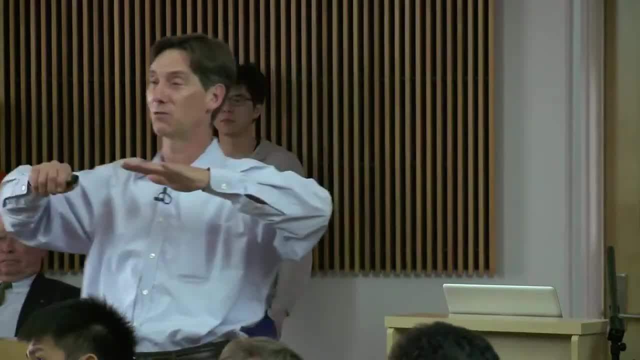 and then, you know, 14,281 years ago, boink and never decided to come back. why, You know? is it really that much of a knife edge when it comes to atmospheric circulation? And I don't believe it and I have trouble with it. 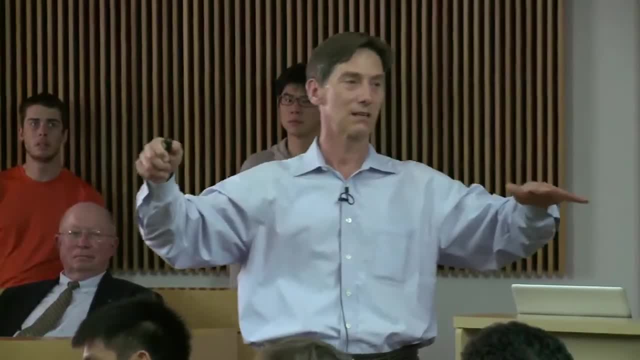 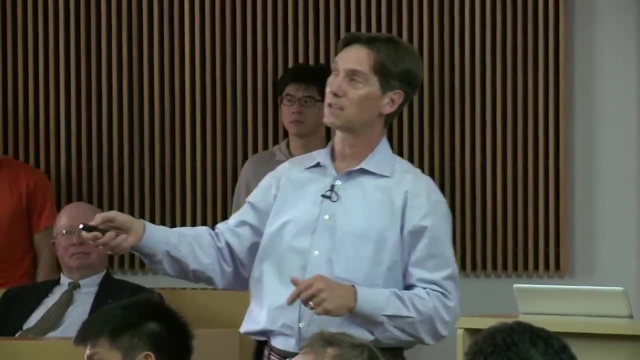 And so you've got, you know, two mechanisms, both of which can transfer large amounts of heat, one of which seems to have the ability to stay in states, but doesn't seem to be able to make things change fast enough for us. 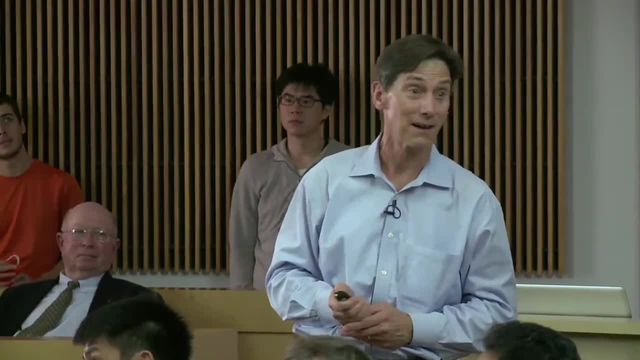 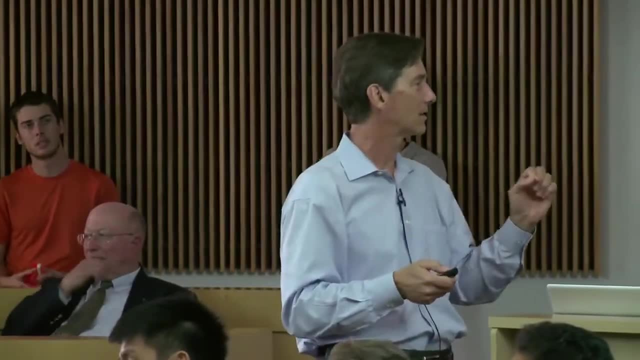 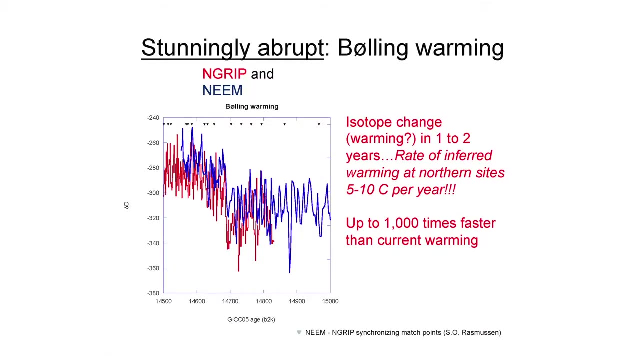 The other, which can change rapidly but doesn't seem to want to stay in states. Well, the atmospheric composition certainly changed, Dust changed, But the yeah, I don't know Certainly I mean greenhouse gases, for example. 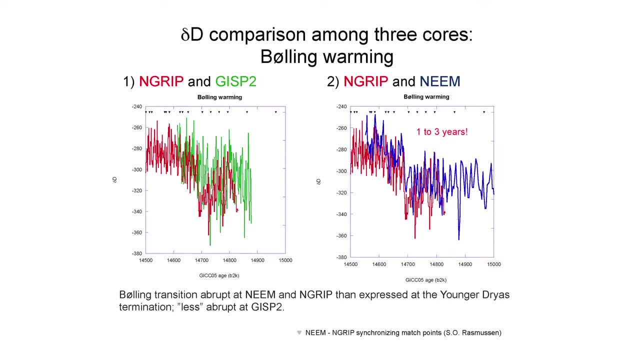 didn't change right away and I don't think they would immediately change things. anyway. Dust can change in one or two years by order of magnitude. That's a wind issue. I mean you've got this strong. I mean clearly what you're seeing in the record, I think 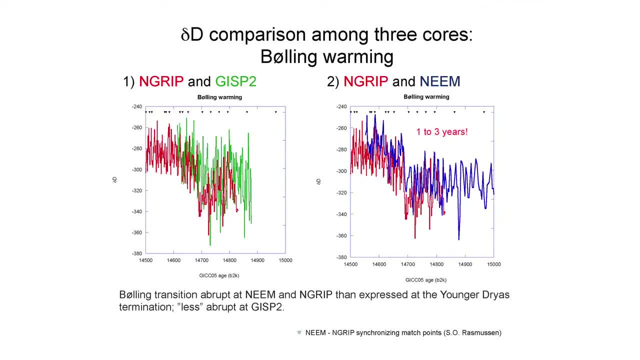 is a fundamental shift in atmospheric circulation, Why it decided not to go back and keep bouncing back and forth for, you know, 100 years or something like that. Why don't you see this crazy period, you know, when no one would want to be alive on the planet at that time? 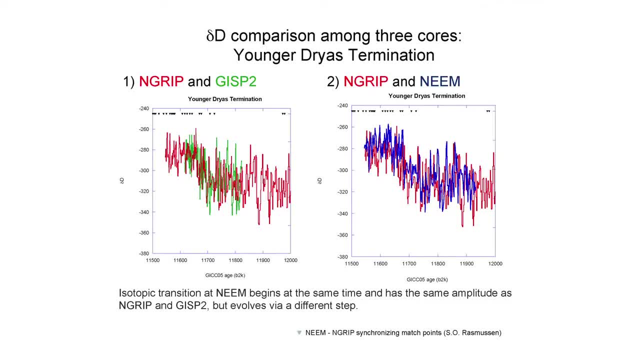 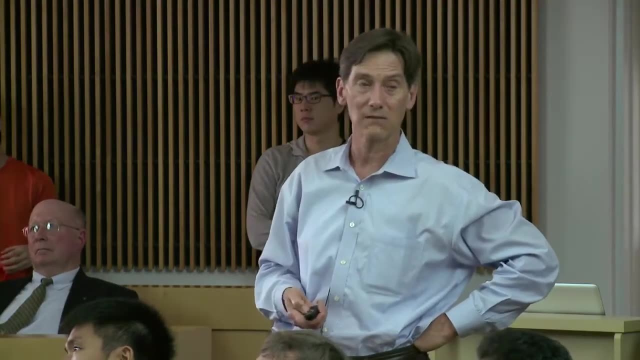 But that doesn't seem to be what happens. What happens is the system cruises along and then boinks to another state and just stays there for a thousand years. Yeah, Does the historical positions of the jet imprint themselves in a potentially sample of the way of the future in certain states in America? 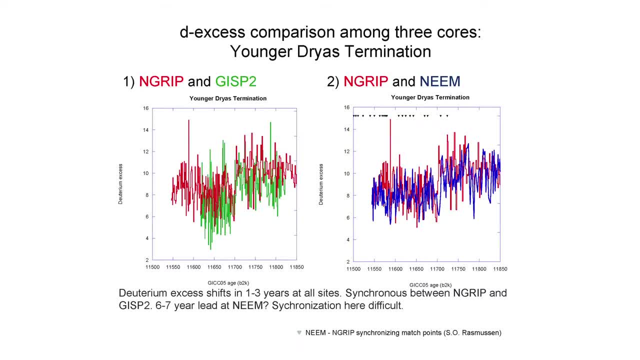 A very good question, The you know. one of the things you know what we do in the ice core business is we look at things like dust and where it comes from. So, for example, the dust that we see in Greenland. 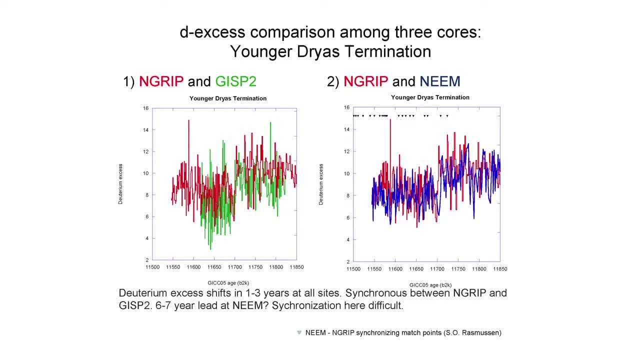 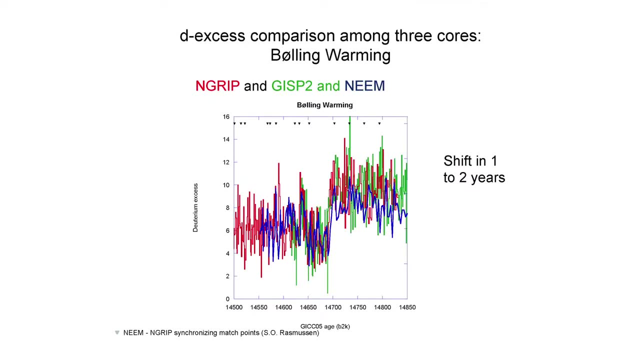 during the coal periods has clay, and the clay composition is consistent with Chinese lust, And so that's why we think that you know. either you had some mechanism by which that dust was picked up and carried all the way around the barn or, more than likely, it was carried up over the pole. 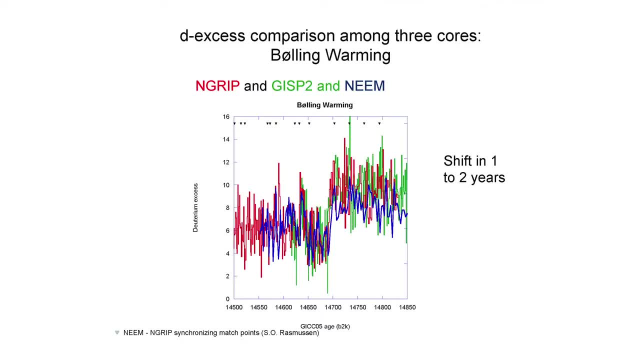 And so the idea of the polar jet comes from that, plus speculation. I mean going back into the 1970s when people first took a look at that Laurentide ice sheet and said: what is that going to do In the early models of Manabe and all. 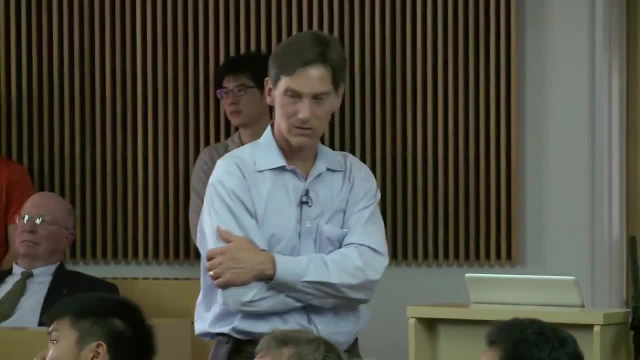 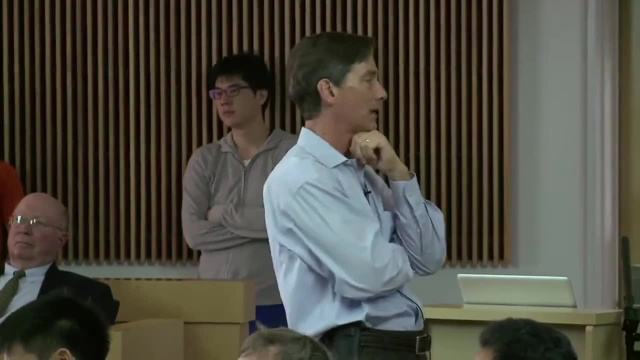 you know what's going to happen to the jet stream under that scenario- And there was. if you look back, there's some interesting papers that argue that maybe the jet stream split at that time. We don't see that so much in the modern model. 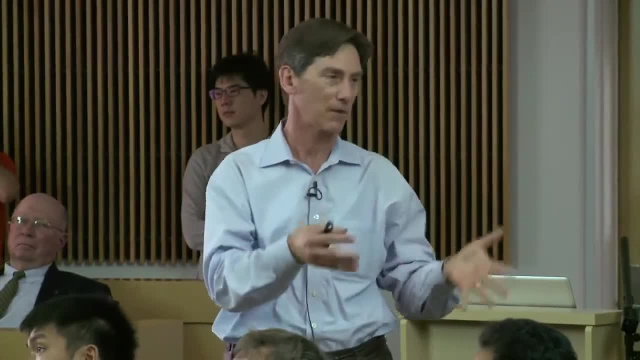 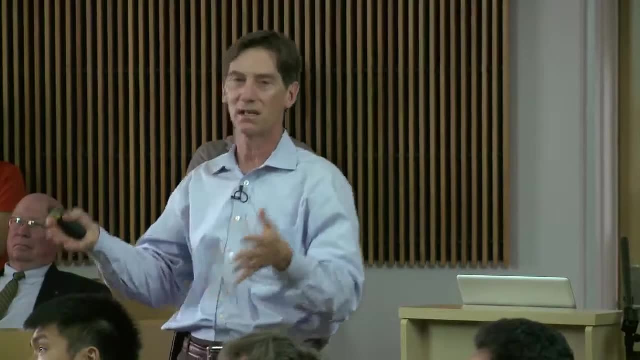 Yeah, Bill. Yeah, but you did, I did, yeah. Yeah, the question I had is: you talked earlier about the continuous, you know, right after the core is retrieved, measurements Are those followed up by discrete measurements back into the lab? 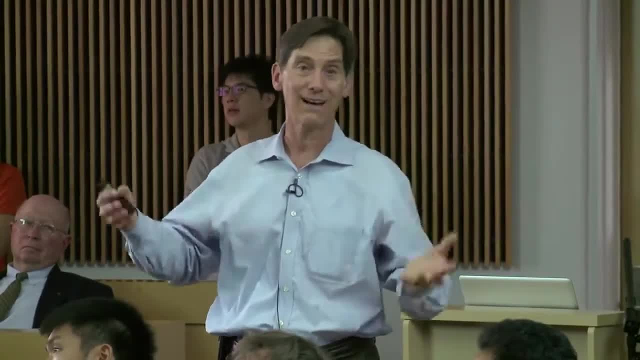 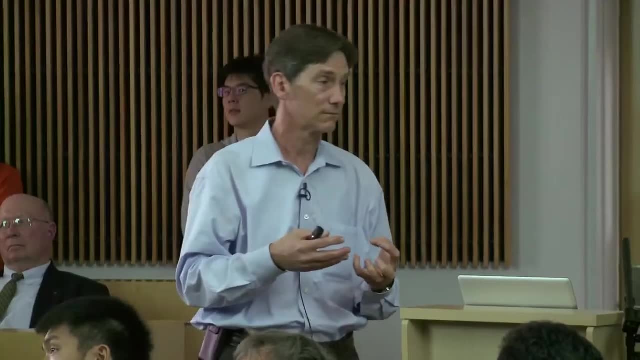 or is that sort of service? you know, do you do both of those? A good question On the Neem ice core: we're doing both, I think, the continuous flow methodology which I- that's a whole other talk I can give. 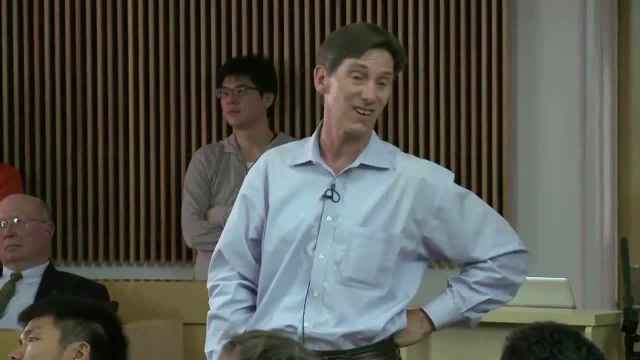 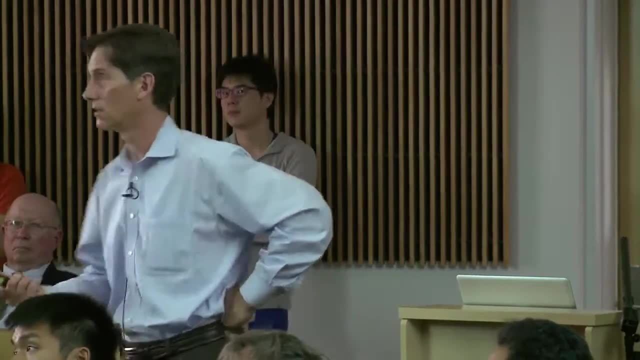 I think that's where we're going. I think that's where we're going and we don't need to do the cuts, discrete samples, anymore. Continuous flow technology does a couple of things for us that's fantastic. One is you get the highest resolution you can get out of the ice core. 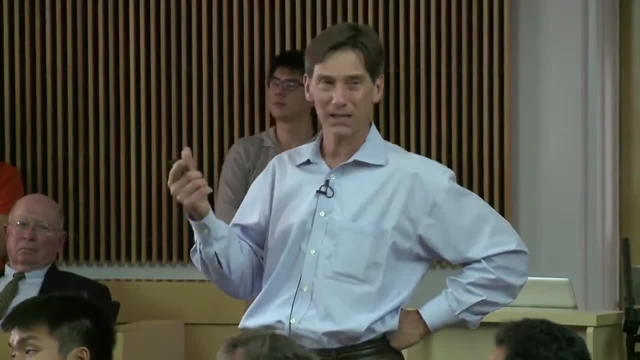 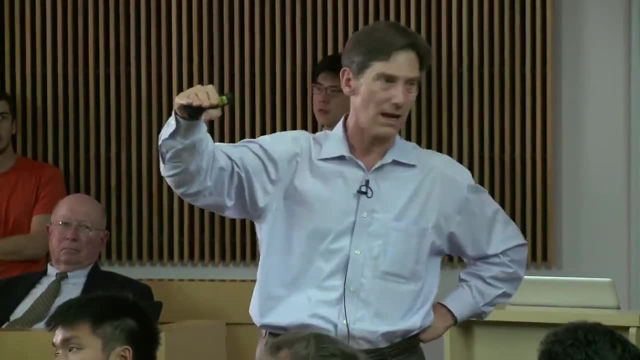 If you're willing to melt at a low enough speed, you can get the highest resolution the ice core allows you to have. The other is that in a matter of about eight months we can measure a three-kilometer ice core. That would take us five years under a cut and measure approach. 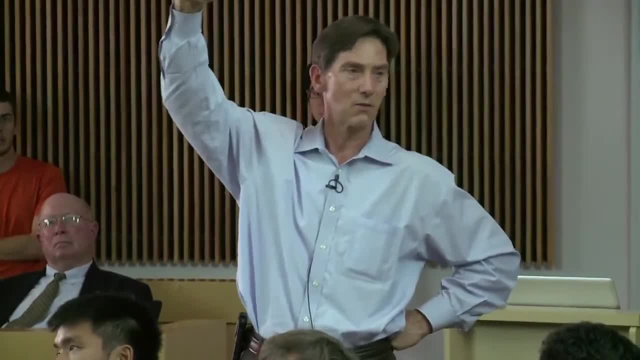 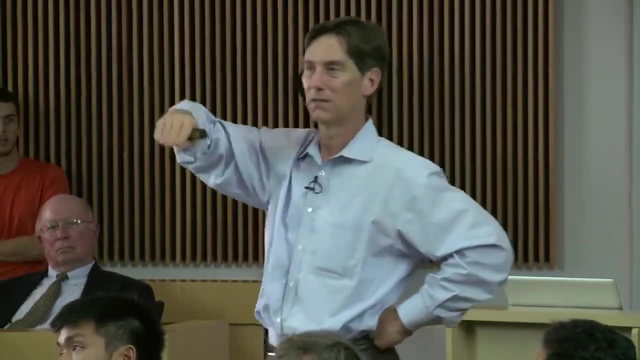 So it's going to be a game changer and the West Antarctic ice core will be finished soon and it has, you know, annual layering back 10,000 years and it has ENSO signatures going back 40,000 years. 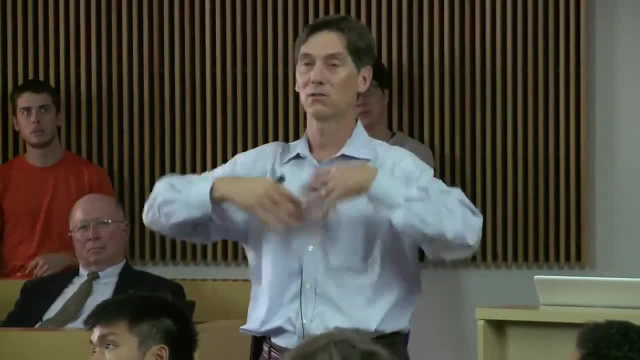 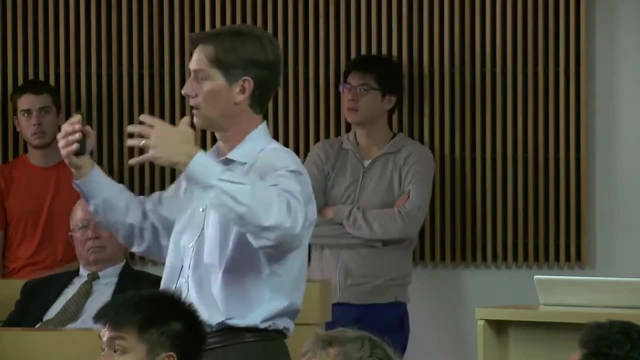 and we can tell that now for the first time ever because we got these records. One other thing I'd like to say. a lot of the ice core studies have always been presented as just SO stories. It's just this one. Yeah, You're talking about the moon removal.